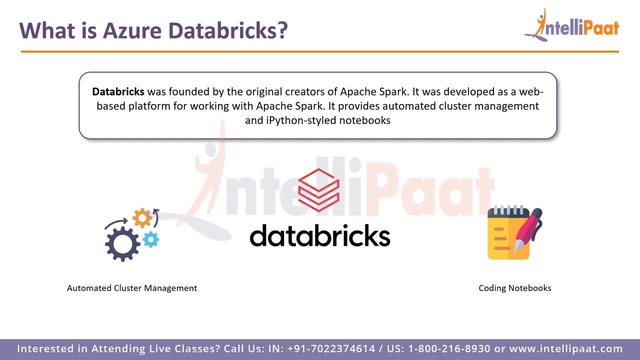 all of it is automated and on top of that you get ipython style notebooks. so if you're coming from a data science or data analytics background, so you must be familiar with jupyter notebooks. so that is what essentially ipython notebooks are. so you get them pre-installed with databricks. so 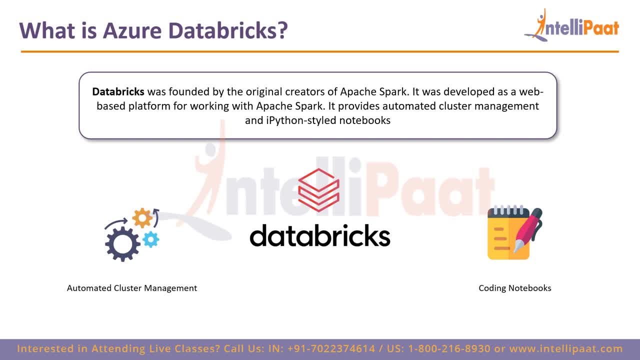 you have your cluster, you have your notebooks pre-installed. you launch your notebook on top of the cluster. whatever code you execute in that notebook will utilize the full functionality of the cluster that you have if you're using the spark libraries. so the two features we need to. 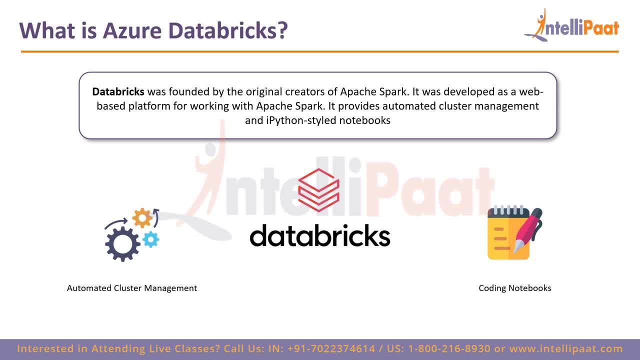 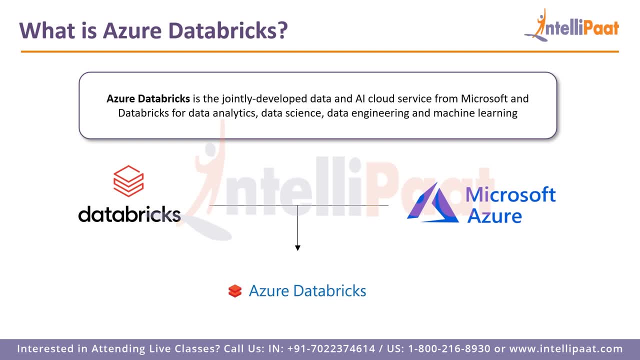 focus on when talking about databricks would include automated cluster management and coding notebooks. so now that we know what databricks is, we can move on to what azure databricks is. so when we move databricks to a cloud service, for instance microsoft azure, it's called azure. 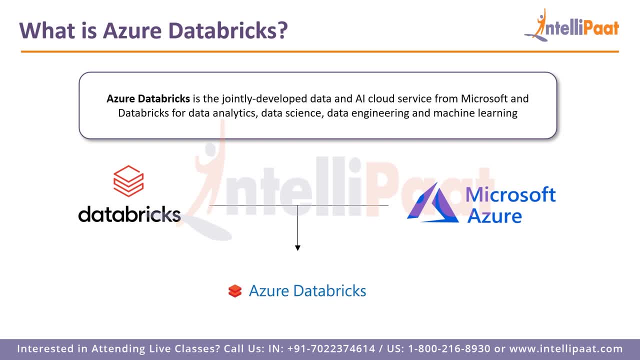 databricks. it is the jointly developed data and ai cloud service from microsoft and databricks for data analytics, data science, data engineering and machine learning, so essentially all activities related to data. you can use azure databricks for that, especially if you're dealing with big data, so we can see. 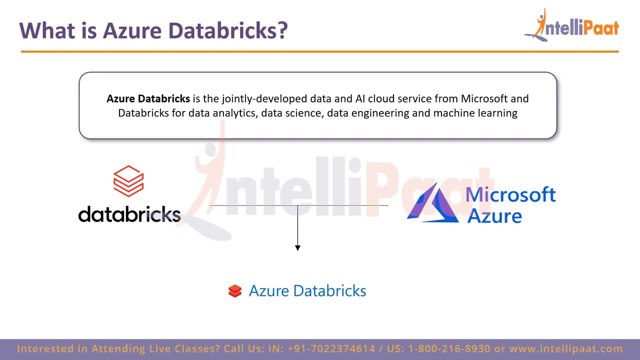 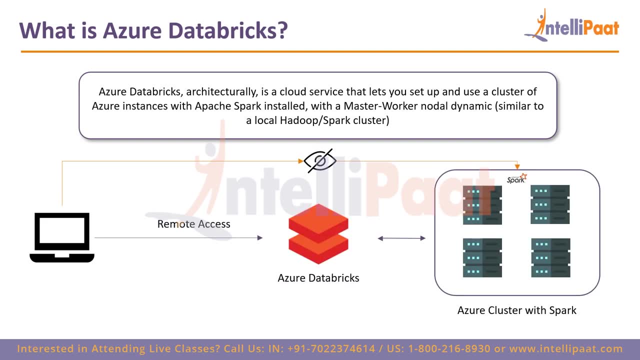 when we combine databricks with the microsoft cloud service, which is microsoft azure, we get our azure databricks service. so, if we look at the architecture that is followed by azure databricks, it is a cloud service, so it lets you set up and use a cluster of databases that are related to azure databricks. 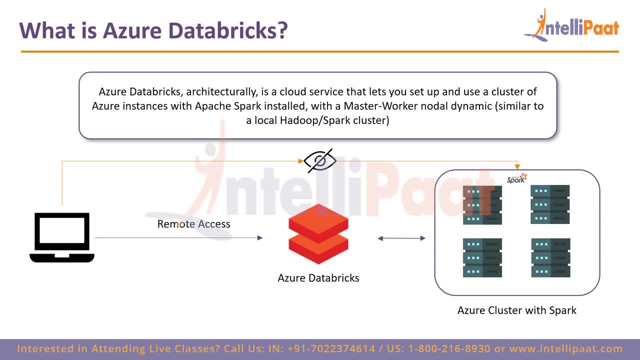 let's say, for instance, arrays like java or analyzing of already established tables, and you want to set up one for one database and then the group you send your building to that would quickly funnel out the data out in azure abcd manager, an bound case, and of course you don't. 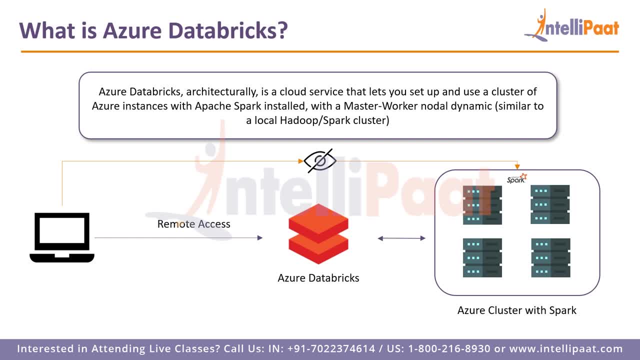 need to have enum in there for that, so you don't have to wait till it shows upasilux. check this out. once you've done that, it will let you just check this out. you'll see that on the left hand side right over here, we've recommended the hard disk space. without any左 liver bugs usually. 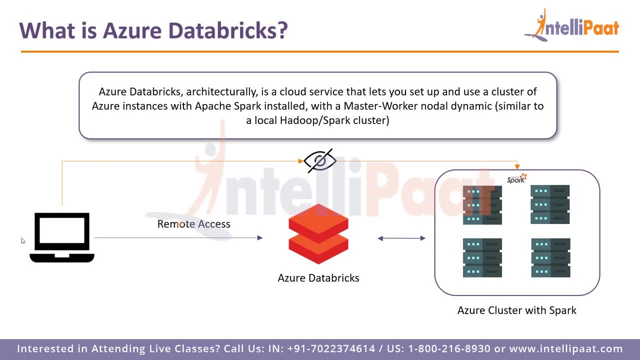 We have our remote site client. This is the device that we're using to access our Azure Databricks service. Then we initiate our remote access to our Azure Databricks console- say your web browser, And then that's all we need to do. 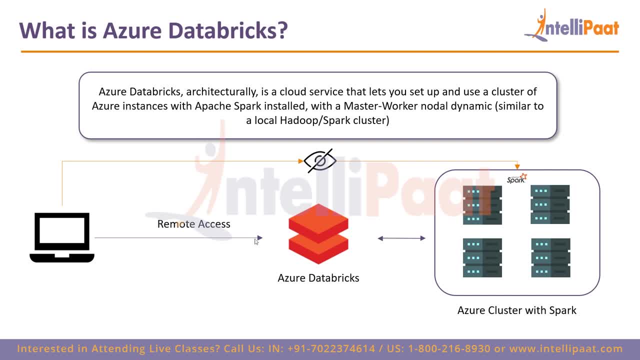 Here is where we will be basically interacting with. We wouldn't be able to see the actual servers, We wouldn't be dealing with any of the complexities of maintaining the actual instances that we are running for our cluster, The nodes that we are running for our cluster. 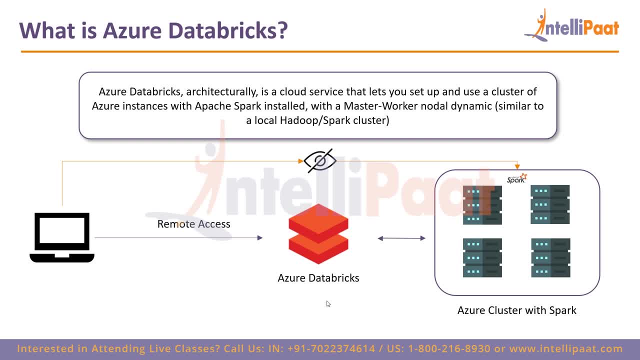 we don't need to deal with that. Azure Databricks manages all of that for us. So once we send our commands to our Azure Databricks service, it will send those commands to the cluster that we have for the Spark cluster that we have. 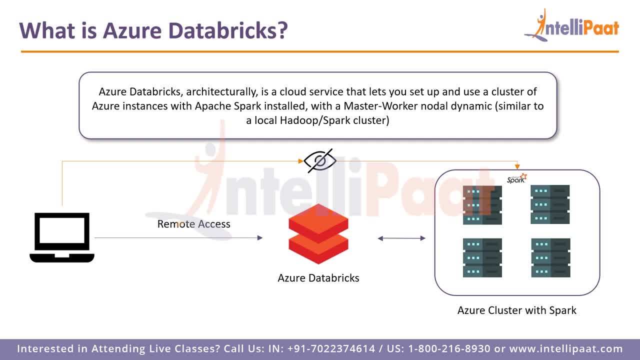 And we will get our use cases resolved. And when dealing with cloud services, the main advantage is abstraction, So we do not need to deal with any of the complexities of the cluster. So that is why we have the invisible icon over here, because we're not dealing with the cluster directly. 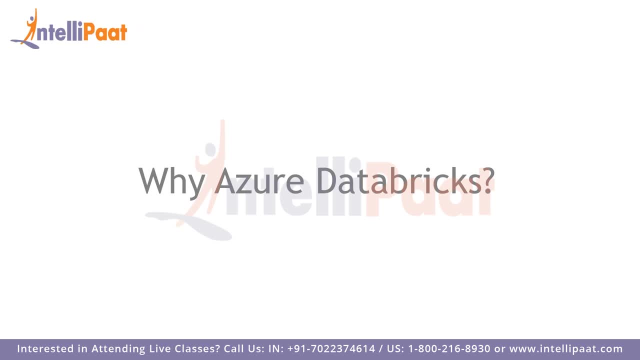 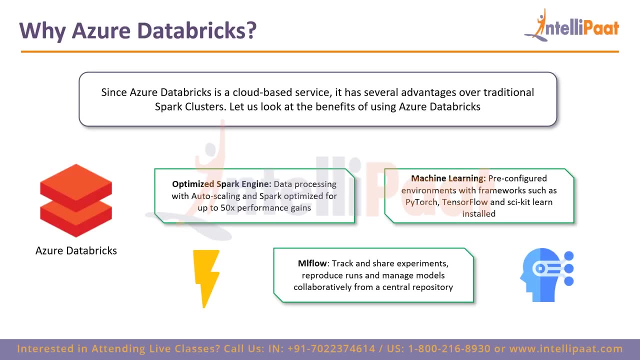 So now let us move on to why Azure Databricks. Why do we use Azure Databricks as a service as opposed to any other means of analyzing data or big data? So, since Azure Databricks is a cloud-based service, a Microsoft managed cloud-based service at that, 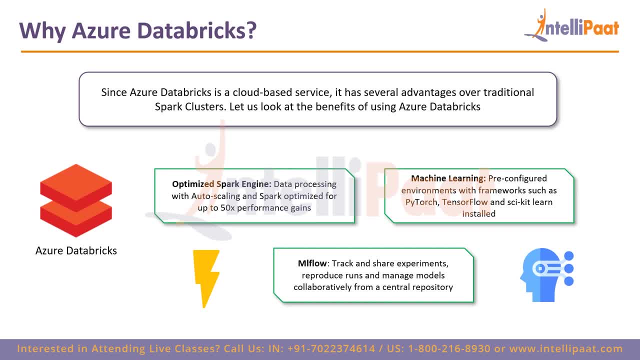 it already has several advantages over traditional Spark clusters, which means that locally hosted Spark clusters, which means that locally hosted Spark clusters or locally hosted Databricks clusters- when we are using Azure Databricks- we get several advantages over them. So let us look at some of the benefits that we get. 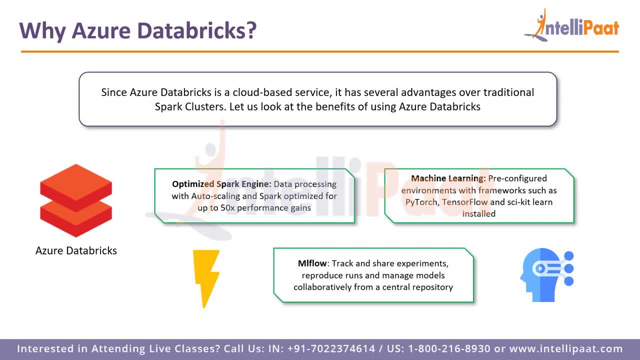 when using Azure Databricks. So, firstly, an optimized Spark engine. So what does this mean? Data processing with auto-scaling and Spark optimized for up to 50X performance gains. So 50 times performance gains, right? So say, if you're hosting a local Spark cluster? 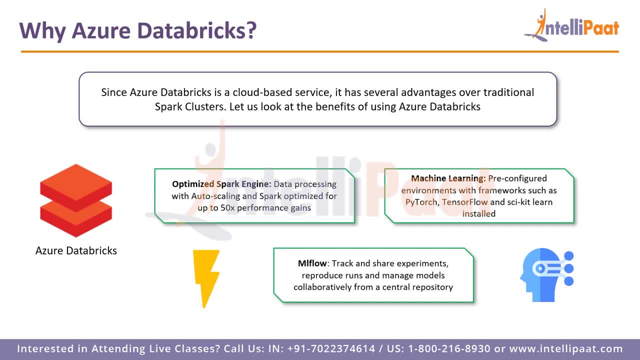 So say, if you're hosting a local Spark cluster in your office space or in your server room, you don't have such complex features as auto-scaling or optimization of your Spark engine. You don't have those features automatically available to you. You have to manually adjust a lot of things. 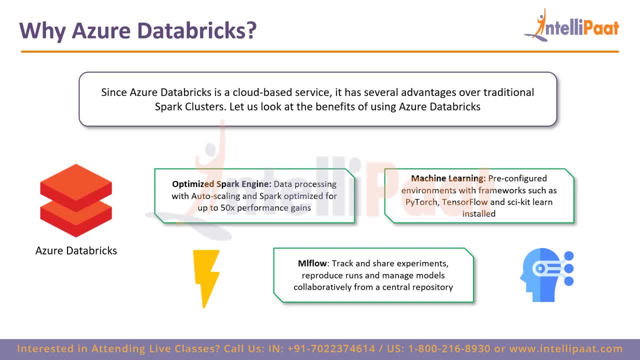 You have to manually install or remove nodes from your cluster. So when you're dealing with a Microsoft paid service, when you're dealing with a Microsoft cloud service, you get auto-scaling features with it. So, depending on the use case that you have, 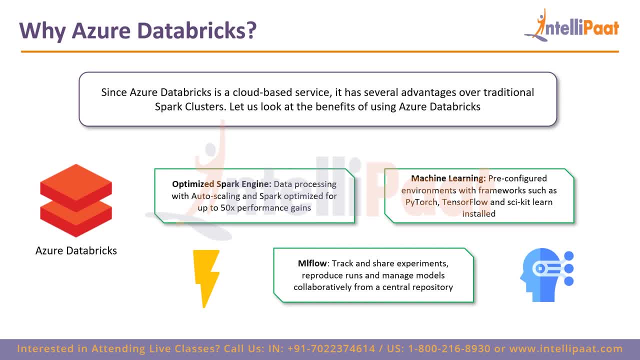 depending on the workload that you currently are dealing with, are dealing with, microsoft has the option to scale up your cluster or scale down your cluster. so it helps you reduce costs and it optimizes uh the, the cluster requirements, the cluster hardware settings, according to the complexity of the job that you have at hand. then uh, machine. 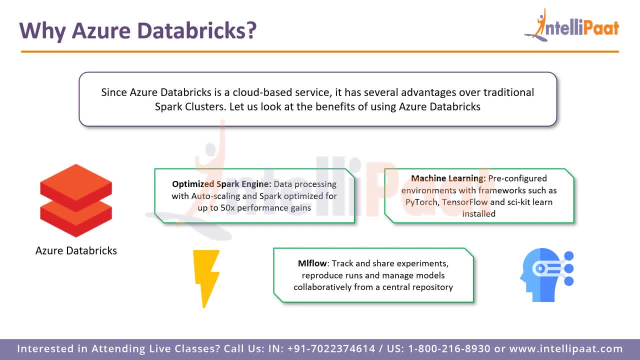 learning. so there are pre-configured environments with frameworks such as pytorch, tensorflow and scikit-learn already installed. so we will get into this when we get into the data bricks utilities. but basically the point is, all of these libraries such as pytorch, tensorflow and scikit, we can get. 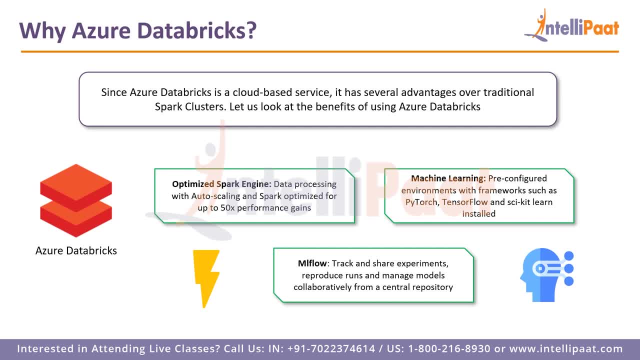 pretty easily when we are using data bricks, instead of having to manually download those libraries and installing them into our environment. and then ml flow: track and share experiments, reproduce runs and manage models collaboratively from a central repository. so ml flow is a feature provided to you by microsoft ashore which helps you uh. 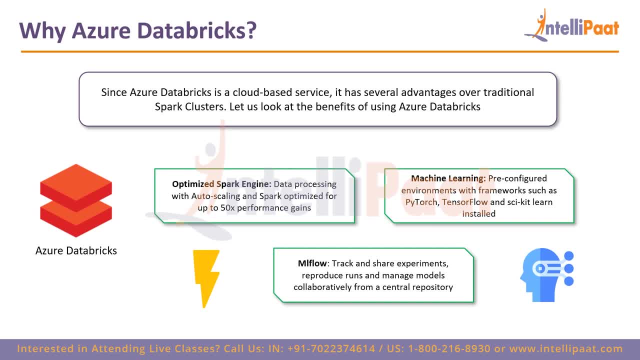 basically collaborate with your teammates that you may have in your data analytics team or your data science team. you can share your experiments, you can try to reproduce the runs with the models that have been created. you can manage the models that you've created and you can manage them, uh, from a central 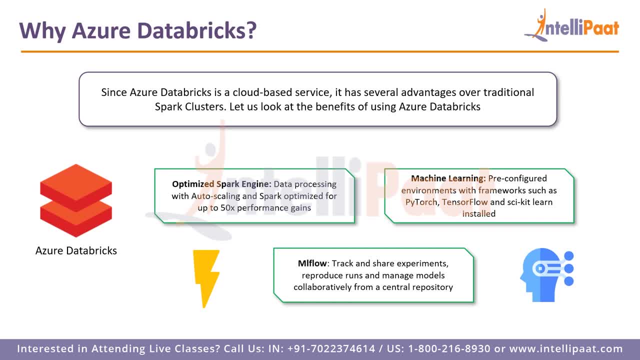 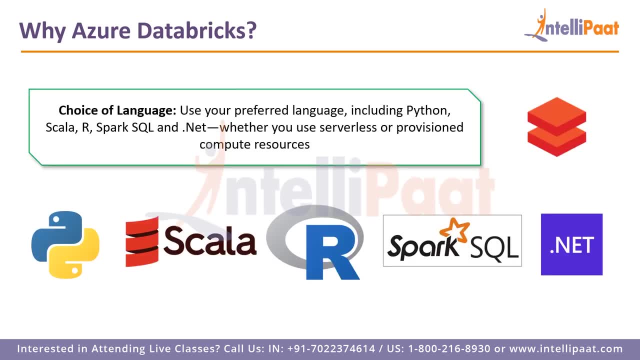 repository so you can push and pull uh all of the models that you've created and deposit them into a central repository so that your teammates can access them as well. then, uh, one of the best features that you get with using data bricks in general, not just azure- 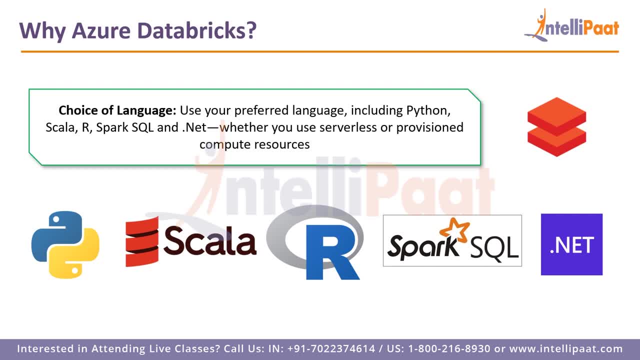 data bricks is choice of language. so, uh, especially in microsoft azure data bricks, when you're uh launching a notebook, once you've set up the cluster and once you're launching the notebook, you get an option to start your notebook in the preferred language that you would require. 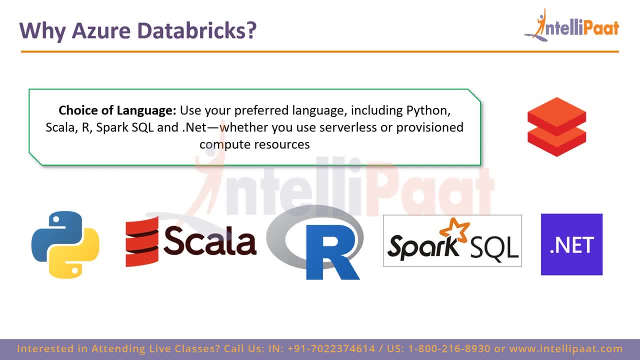 right, so you can start up the notebook in scala or spark, sql or dot net. so whether you use serverless or provision compute resources, you are able to do that. so the best thing about this is that, uh, you can get started with your use case pretty easily. you are not dealing with a lot of setup. 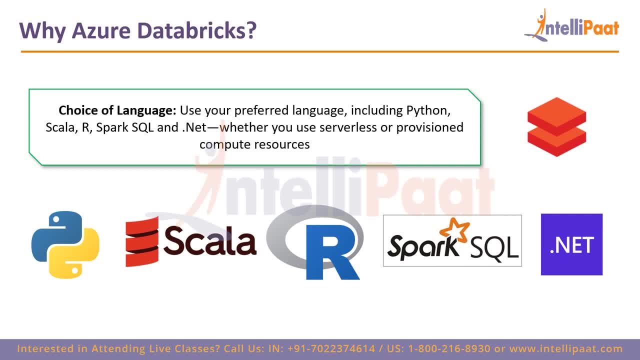 over here. you are not dealing with a lot of administrative job right now. you're only dealing with the use case. you're only dealing with analyzing data, processing data, visualizing data, or whatever your use case may be. so, uh, the next feature would include collaborative notebooks. so 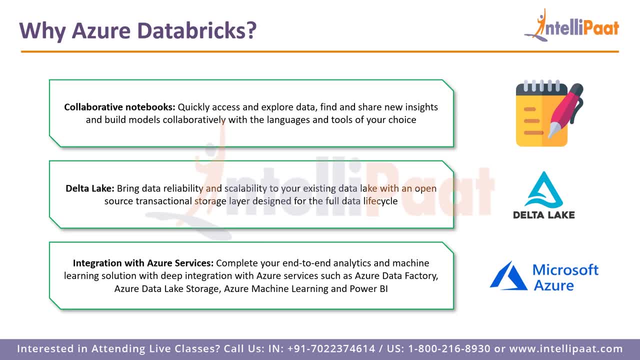 quickly access and explore data. so notebooks obviously can be opened by others as well. you can also do it by your own people. the other teammates can look at your code, they can execute that code. they can make changes to that code, they can make modifications better or efficiently. 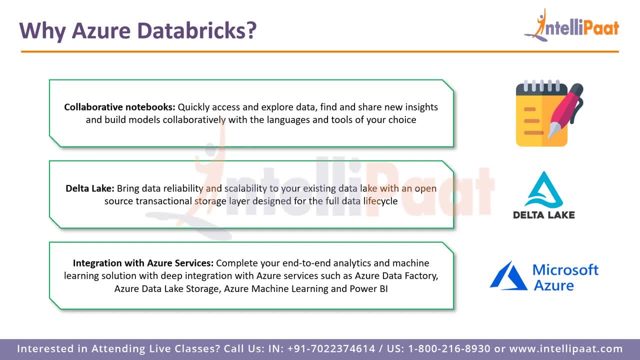 optimize the code. so all of this is basically accessible in a cloud environment pretty easily. you don't have to manually share anything so quickly. access and explore data, find and share new insights and build models collaboratively with the languages and tools of your choice. delta lake- so microsoft assure gives you the service of delta lake so you can bring data. 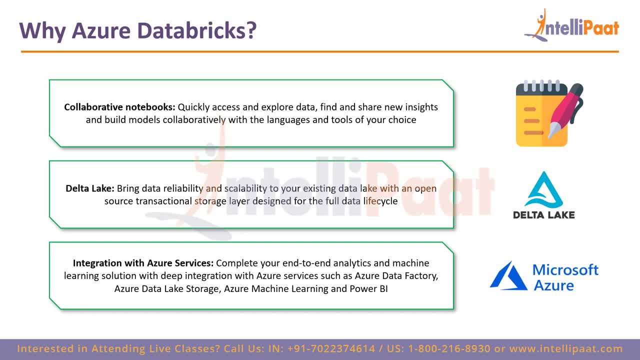 reliability and scalability to your existing data lake with an open source transactional storage layer designed for the full data lifecycle. so when you are using your data bricks with Delta Lake, you can have your data already index for you for faster transactions, integration with other Azure services. so the best. 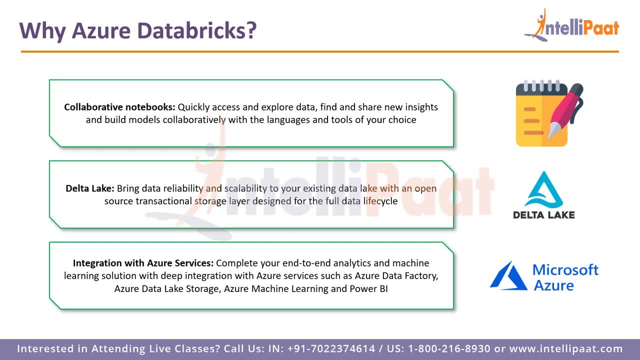 thing about cloud services is that there are other cloud services for various other things as well. so this is the case for AWS, this is the case for Google cloud and this is the case for Microsoft Azure as well. so when you're creating your Azure Databricks instance, when you're creating your cluster and your 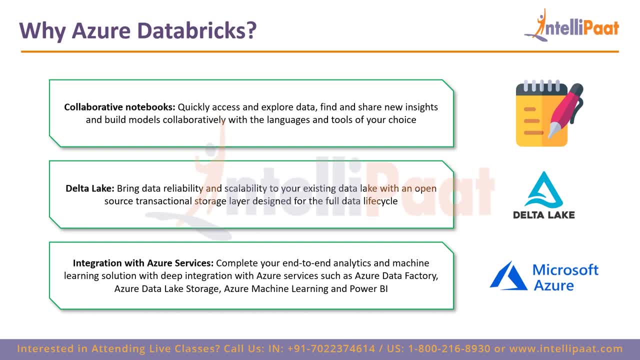 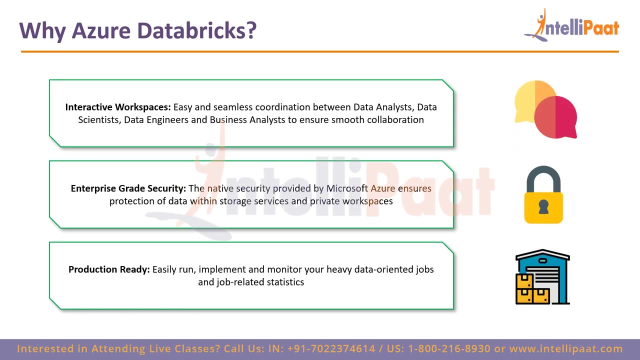 notebook. you can also integrate with other Azure services, so these could include Azure Data Factory, Azure data lake storage, as we discussed before, Azure machine learning, if we are dealing with complex machine learning models, and power bi, if we are dealing with business intelligence. other features would include interactive workspace. 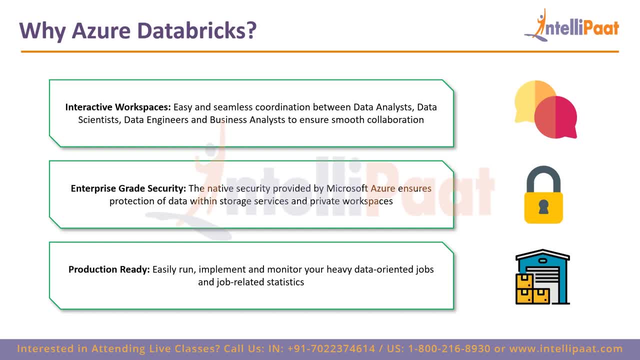 so the easy and seamless coordination between data analysts, data scientists, data engineers and business analysts. so people coming from a data background, a coding background or even from a business analyst background can have a smooth collaboration between them, because these workspaces are interactive and easily accessible by one another and enterprise create security. so another. 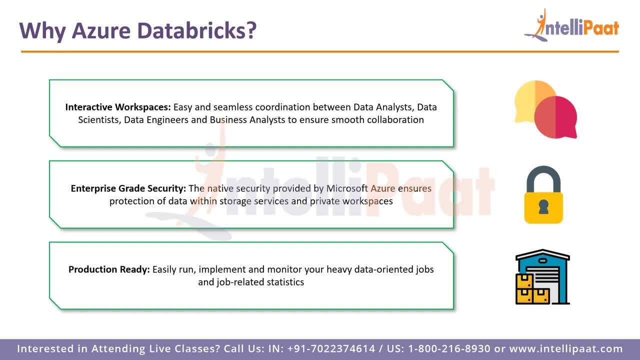 good thing about cloud services is that you get security by default and these companies- they are liable. they are legally liable for any data breach or data loss or any attack by any attacker. right, so it is their job because we are paying them to protect our data. so we get enterprise grade security already. 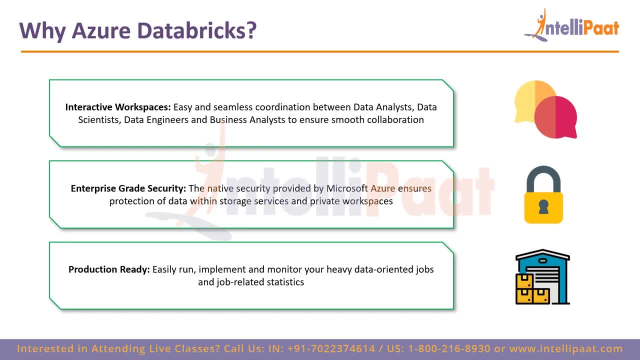 available with our Microsoft Azure Databricks workspace. the native security provided by Microsoft Azure ensures protection of data within storage services and private workspaces. so we already get that, regardless of we are using a Microsoft Azure storage service or if we are using workspaces and Databricks itself, we can be absolutely sure of enterprise grade security. 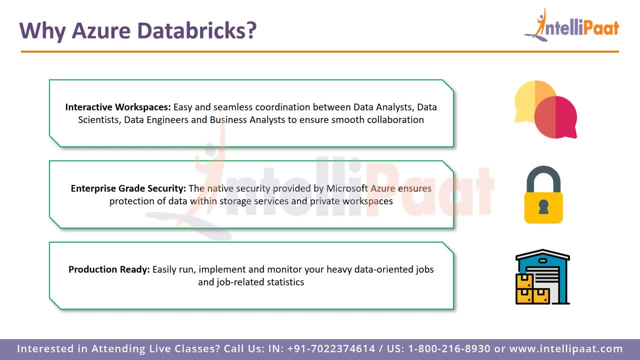 and production ready so you can easily run. you can easily implement and monitor your heavy data oriented jobs when you're running big data jobs on your notebook or your cluster and you can get the job related statistics that you're currently running very easily as well, because a cloud service. 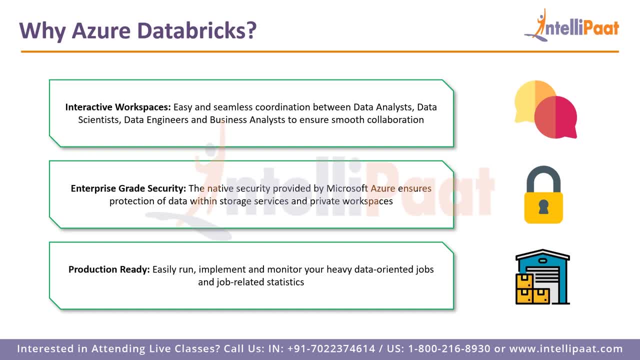 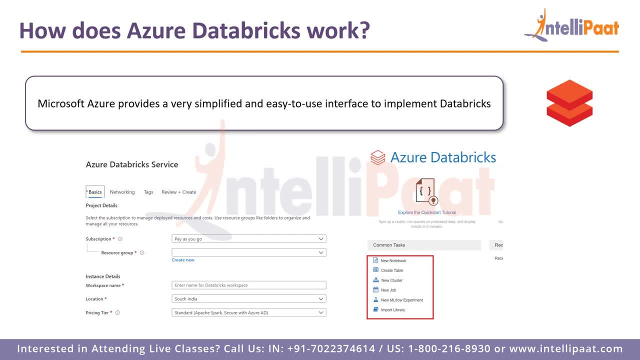 such as Databricks. Microsoft Azure Databricks helps you monitor that. how does Azure Databricks work? so using Azure Databricks is actually not that hard, because you only have to deal with a certain a few UI elements that you get with Microsoft Azure on the default. you have to enter some details and according 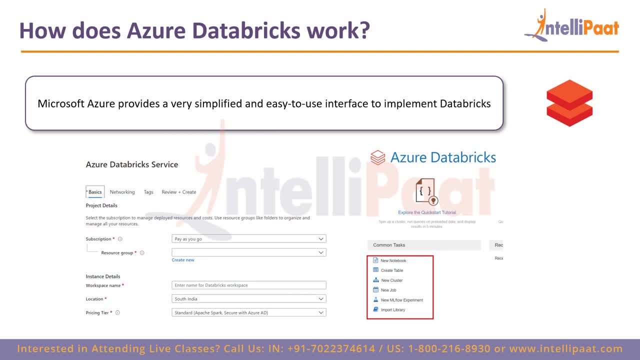 to that, your cluster or workspace will be started. so it's pretty, pretty easy and we'll see that when we reach the hands-on section. but before we actually get to the hands-on section, we need to make sure that we have all the data we need to get to the hands-on section before we actually get to the hands-on section. 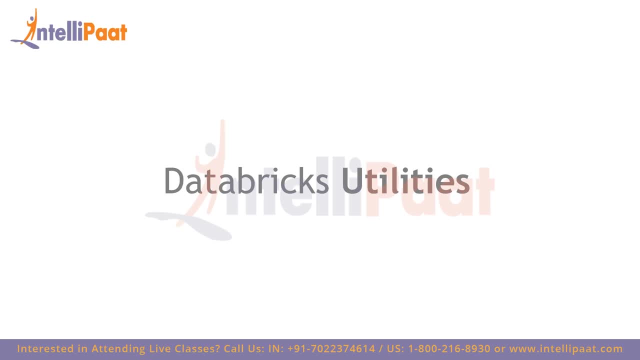 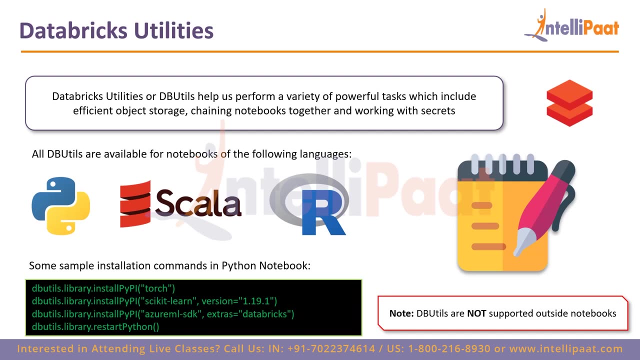 we need to deal with Databricks utilities first. so this is a Databricks exclusive utility set. so this is basically the set of commands that you already get pre-installed with your Databricks setup. so, outside of your normal Python, Spark or Scala Spark setup that you have, you have these. 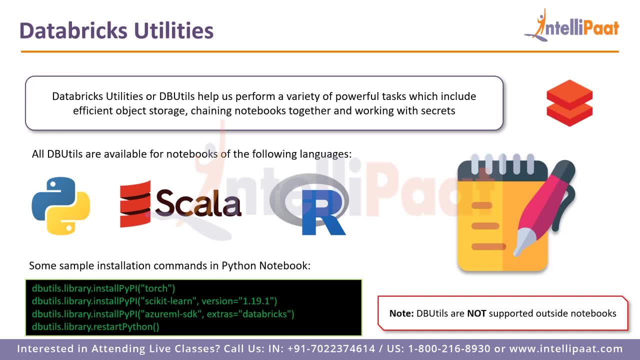 external commands in order to install libraries or packages or in order for you to integrate various as well. say, you have a file available on your data storage service in your Microsoft, sure, and you need to import that file, so you cannot directly, uh, do that when you're using Python with Spark, so you need 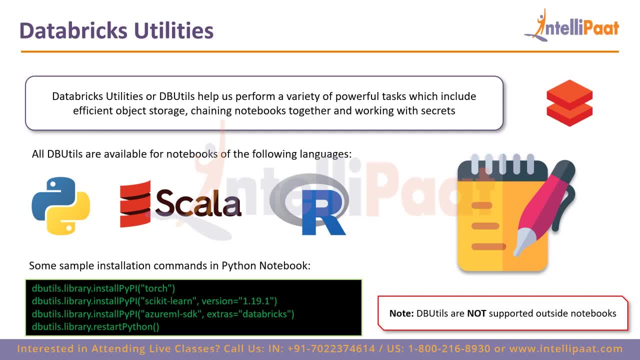 some external element attached to it. so that is where DB utils comes in. so DB utils helps us. help us perform a variety of powerful tasks, which include efficient object storage, chaining notebooks together, so if you have multiple uh ipython notebooks, you can chain them all and perform their functionalities in a sequence, and it also helps you to work with secrets. 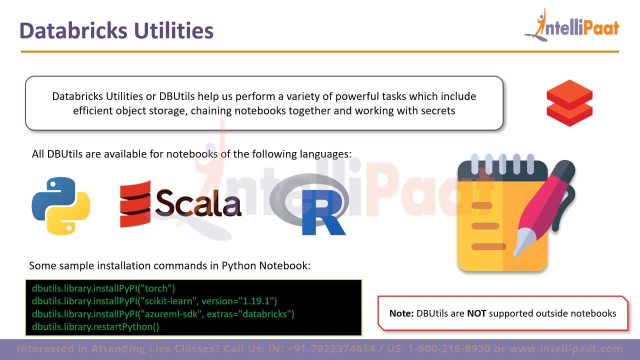 so these secrets are with regards to authentication. these could be passwords, certificates or keys in general, like public and private key pairs. so all of those things you can basically configure into your db utils in order for you to authenticate into a another microsoft azure service, and then you can essentially import your data from there, which we will see. 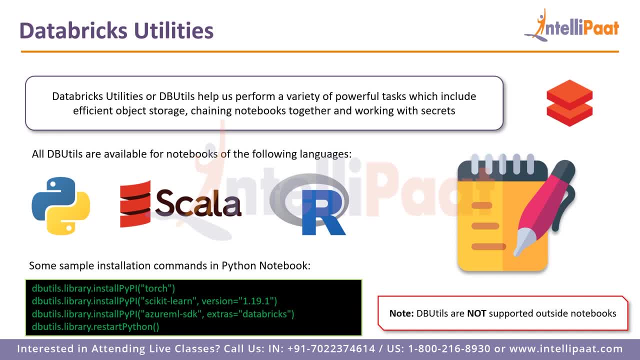 in our hands-on. so one thing to note over here is that db utils are not supported outside notebooks. so you can only use db utils when you've launched a python or a scala notebook with your cluster that you've created, with your spark cluster that you've created. so db utils are not supported. 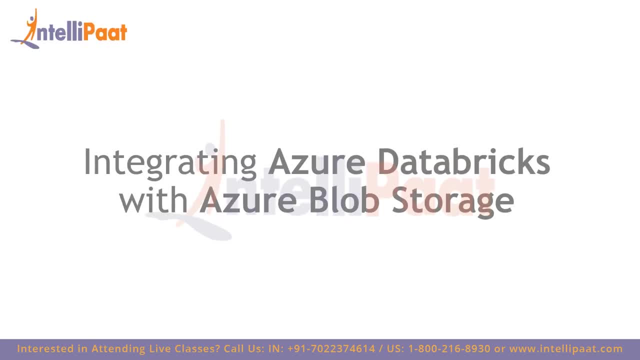 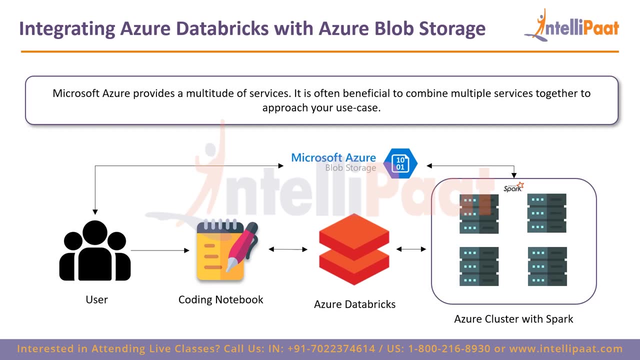 outside of notebooks, integrating azure databricks with azure blob storage. so azure blob storage and azure databricks are both services provided to you by microsoft azure. so these are two separate services, but as long as you're using the same resource group, you should be able to combine these two. so why would you need to combine? 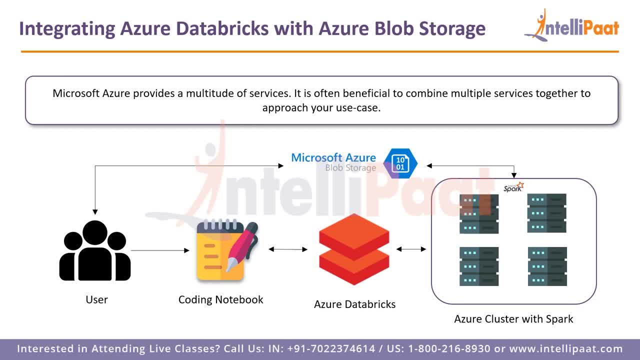 these two. let us see that microsoft azure provides a multitude of services. it is often beneficial to combine multiple services together to approach your use case. so, basically, the advantage of combining multiple services together is that you don't need to engage your local hardware into anything like. currently. i'm using my laptop to look over this presentation, so i want to keep my 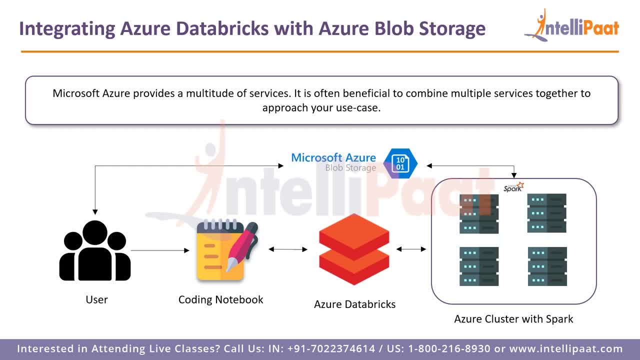 laptop clean, or maybe my laptop is of a lower hardware configuration, maybe i don't have enough disk space right, so in that case i would want to use the cloud services to handle all of my use cases. so i want to use the cloud service to handle my big data storage needs. so i would store it into 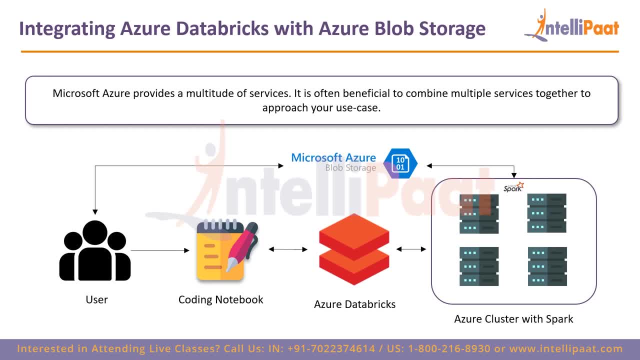 a azure service that i have. i need the cloud service to process my big data, so for that i'll use the cloud service. so all of my use cases are being solved by the online services provided to me by microsoft azure. so say if you want to integrate two services such as databricks and blob storage. 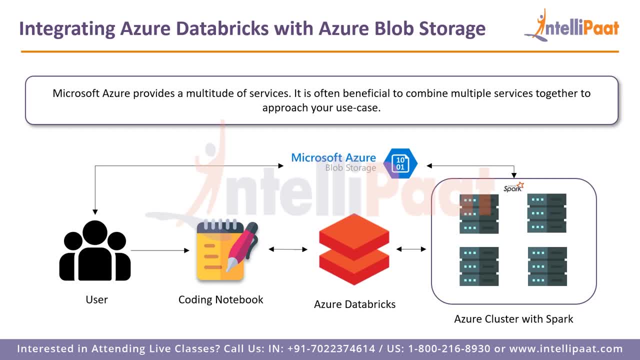 then this is the workflow or architecture for that. so you're the user, you have your device present to you, available to you, and what you'll do, basically, is you'll interact with a coding notebook, right? so this coding notebook is a ipython or jupyter notebook that your azure databricks will create for you. so the way this works is you interact. 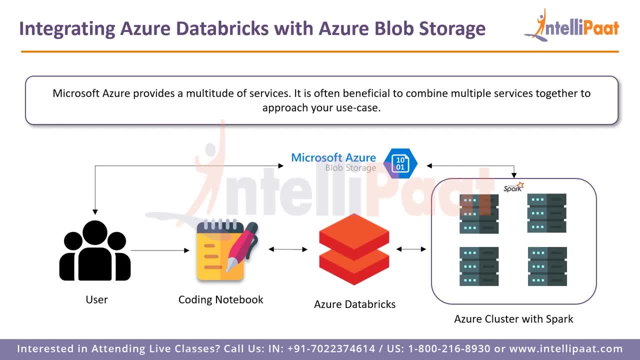 with your azure databricks console. you launch your coding notebook and you type some commands into your coding notebook. the coding notebook commands are then sent to the databricks service and the databricks service sends those commands to your azure cluster. right, so the cluster that you created after you've created your databricks workspace and you've created this notebook on top. 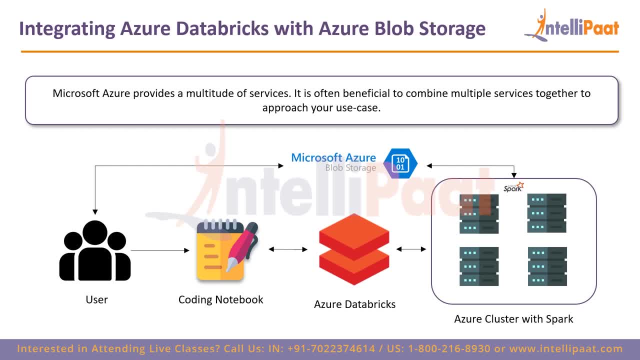 of that cluster. so those commands go into the cluster. then, depending on the authentication provided to the cluster with regards to your blob storage account, the authentication details are sent to the blob storage service, the data is fetched from the desired directory, it is brought back inside the cluster, the data is processed and you see your output on your coding notebook now. 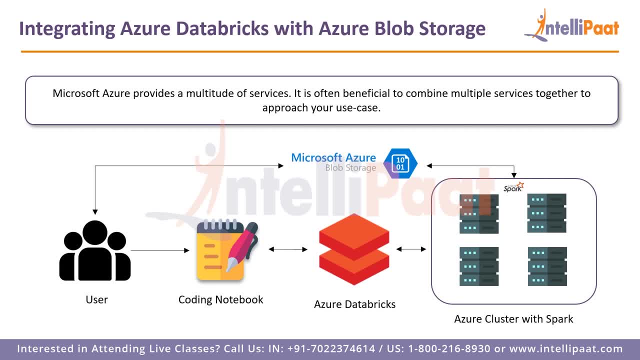 it just works two-fold also, so you can directly upload your data to your microsoft azure service. once you've uploaded that data over there, you can then access your coding notebook and access that data from your azure databricks service and then process it and then get your results, and from then on you can also store the output that you've created back. 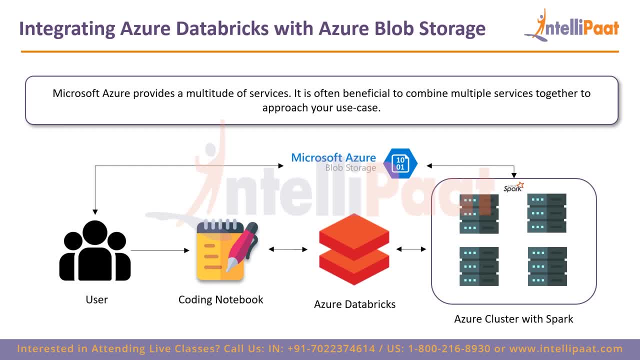 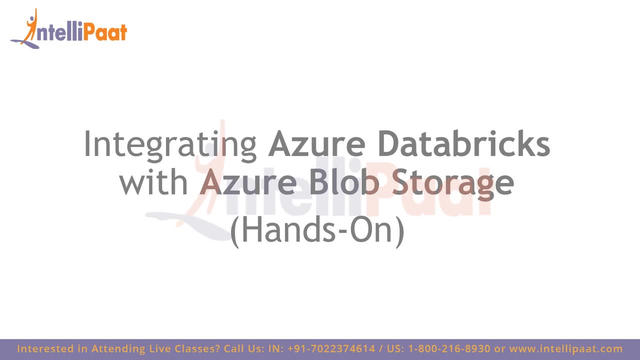 into your blob storage space, so all of this is very easily handled and seamlessly integrated together. so now, now that we've discussed the architecture, let us look at how to actually implement this with our hands-on section. so, now that we've gone through the introduction to azure databricks, we will now be heading over. 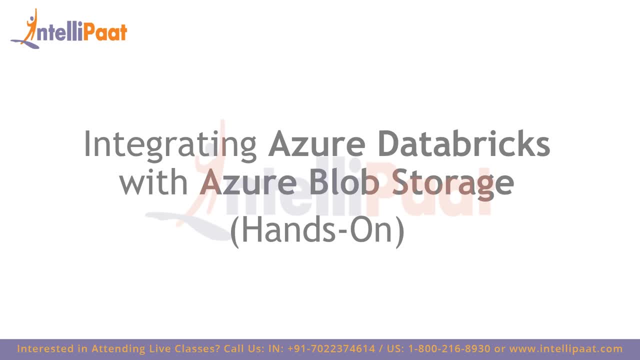 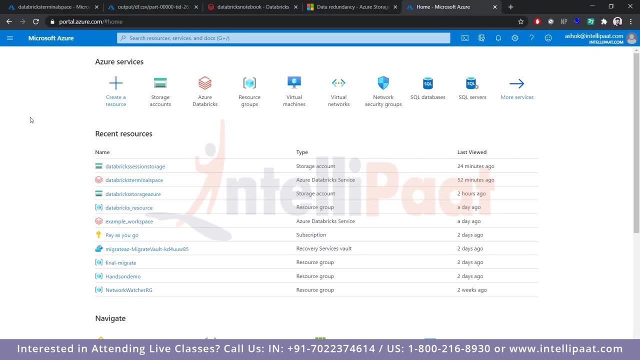 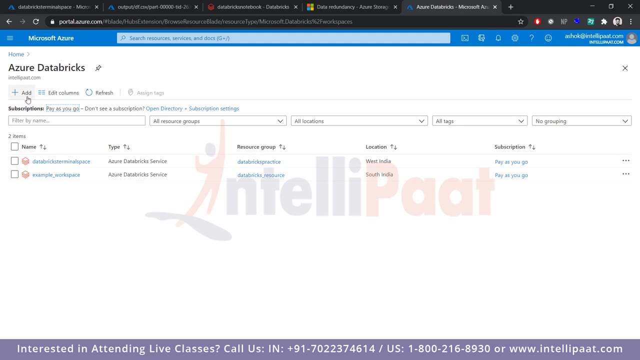 to the hands-on section of things, where we'll be integrating azure databricks with another microsoft azure service, which is azure blob storage. so let us get to it. simply go to the azure databricks service on your azure portal, click on it and then simply click on add. so once. 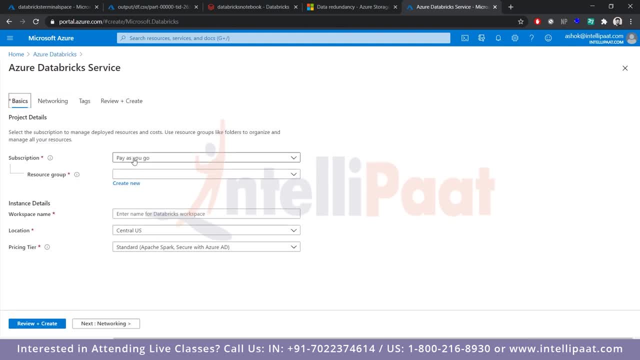 you've clicked on add, you'll get a lot of options. so the subscription will be pay as you go. create a new resource and then click on add. so once you've clicked on add, you'll get a lot of options. now, if I pick a resource group as you want, remember the name. just be sure that you remember. 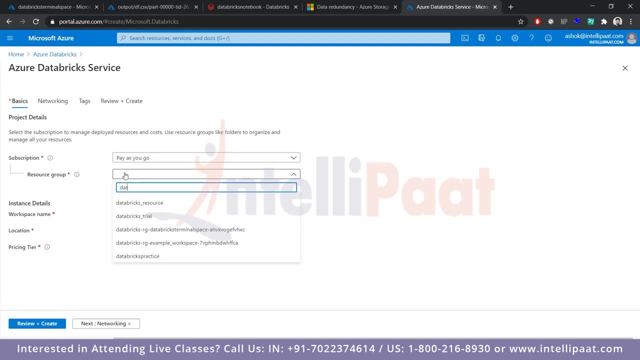 the name, so i can type in something like databricks resource group, and you can give anything that you want, but for now let's just use the databricks practice resource group. so this, this is a resource group that has already been created, and then you can name your workspace anything, so let 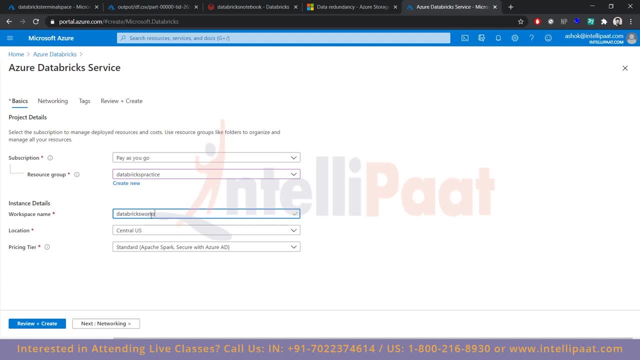 us call this databricks workspace one and select the location that you would prefer. So it's generally a practice to select the location that is the closest to you. So let's select West India and then we can simply decide the pricing table. So in the pricing table, go for the trial one, because you're going to be practicing. 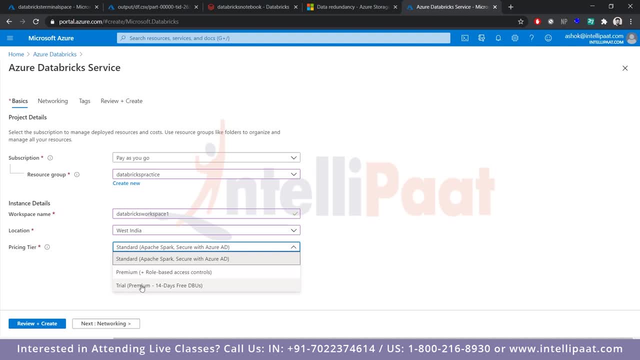 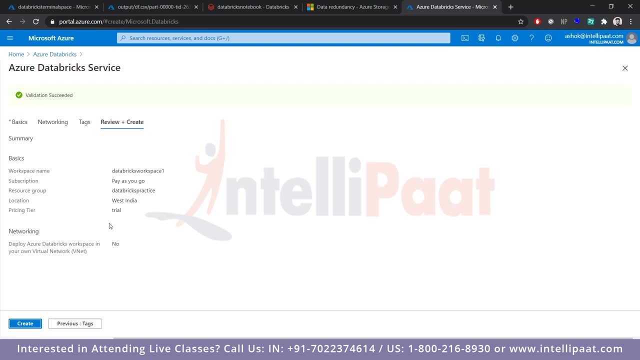 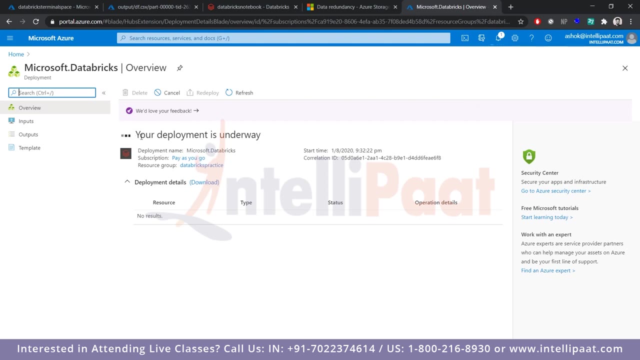 You're not going to be actually implementing any organizational needs. So go for the trial version and then click on review and create. Just look at everything that you've selected, see if it's right and then click on create. So once you've done that and the deployment is underway, you will have to wait up until your deployment is actually ready for you to be able to go to your resource and do what you have to do. 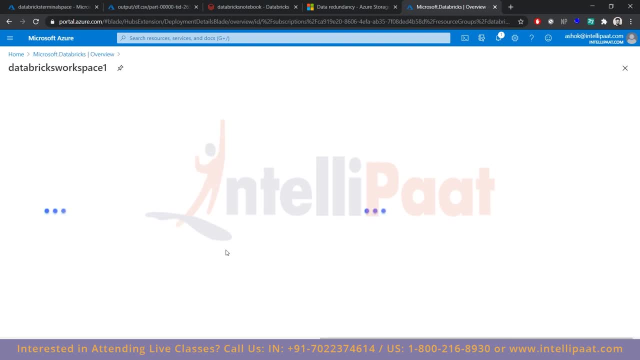 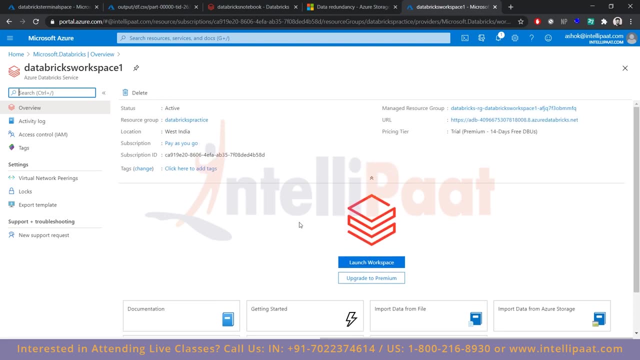 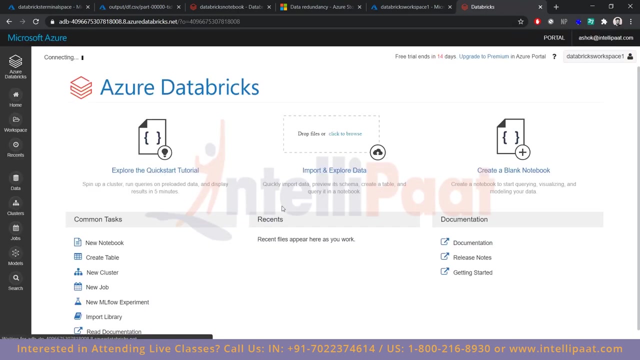 And once your deployment is complete, you can go to your resource and launch your workspace that you require. So you can click on launch workspace from here and then you can essentially log into the Databricks portal. It will sign you in And from there on, 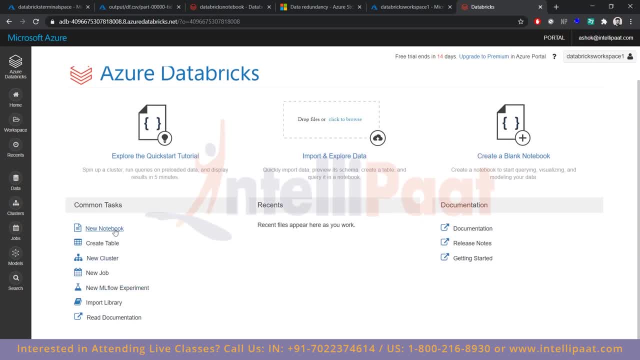 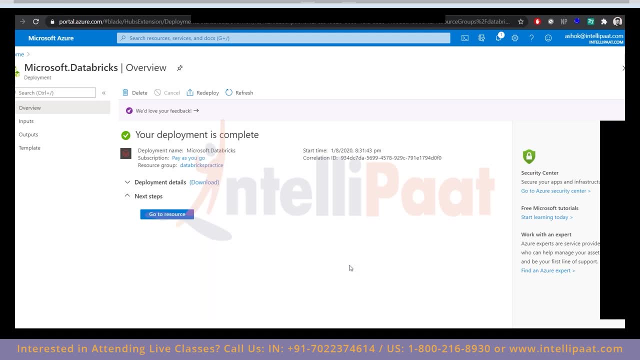 You have these familiar options where you can create a cluster, create a notebook and essentially get started with your Databricks journey. In Databricks I was confused with an AWS service. In Databricks we don't actually use the HDFS. 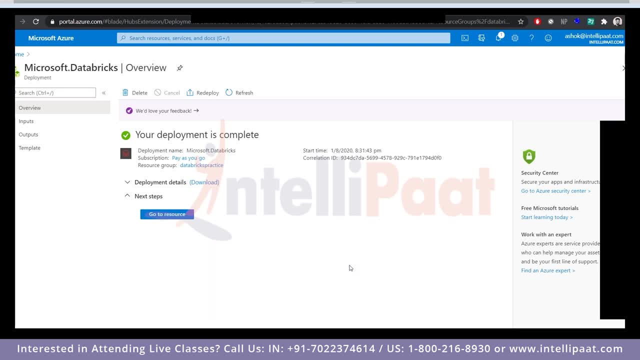 We're using DBFS, So it's the exact same thing as HDFS, except DBFS has this network element to it which helps us combine cloud instances. So Databricks file system In theory. in practice it works in the same way as the HDFS. 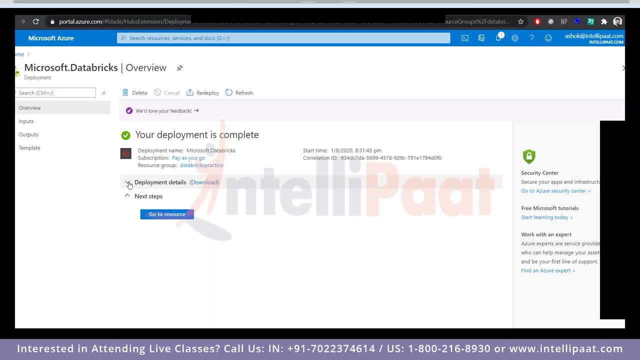 So there is no Hadoop. Hadoop is not coming into this. Hadoop is not coming, It's not required. So then, how this is happening. So in the Spark practice that you may have done in the past, the theoretical information is: Spark is not dependent on Hadoop. 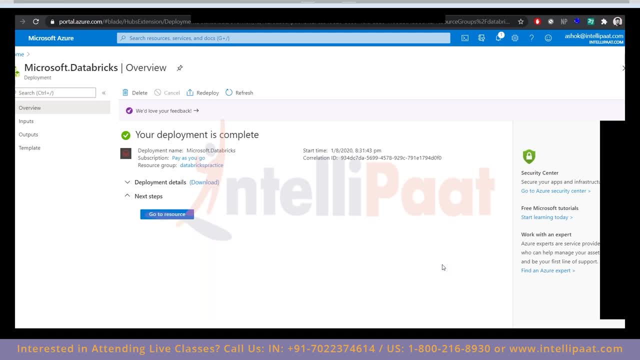 What I have learned is Spark can use either Mesos or Hadoop. Only two are allowed. Two you can use, So that's not a problem. Spark can use any Any distributed file system. Spark doesn't have a limitation to Mesos and Hadoop. 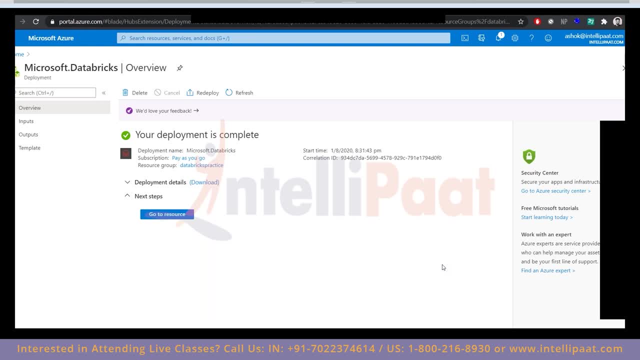 It can use any distributed file system. Okay, Is it Okay? Okay, There's no, I think there's not a compatibility issue. That is what Spark. that is why Spark is flexible. It doesn't have a compatibility issue. You can use the local file system as well. 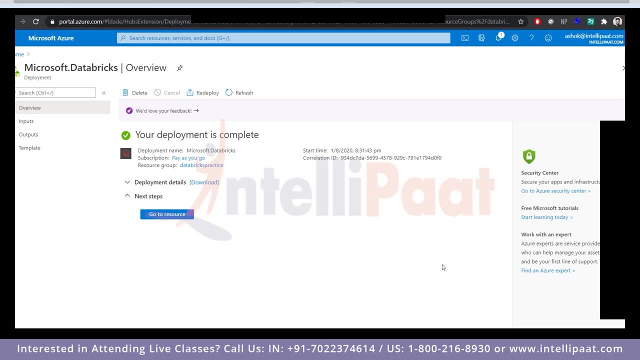 You can use an online file system as well. You can use a distributed file system as well. So all of those things are possible with Apache Spark. I'm sure you've used local files when you were practicing with Spark. Yeah, that's correct. 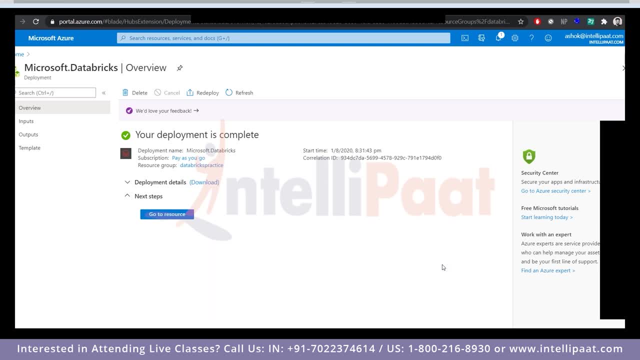 But In actual practice it has to be. this application has to be routed to all nodes, right? That has to be done either through Mesos or Hadoop. That's what I thought. Okay, Yeah, So this is going to be just that way. 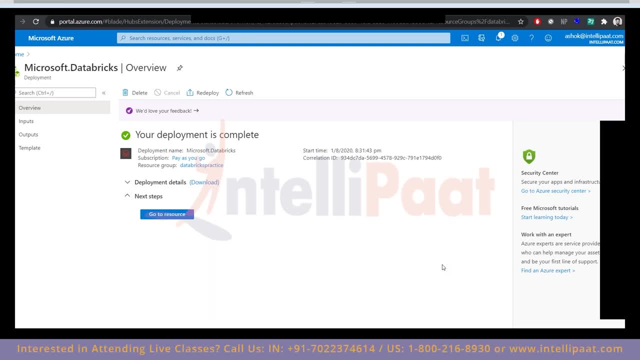 When, once we ingest the data, it is automatically replicated across, depending on, depending on the configuration, it's automatically replicated. when the data is ingested, it's replicated across, divided into parts, replicated across the nodes, And then we process it with our commands. 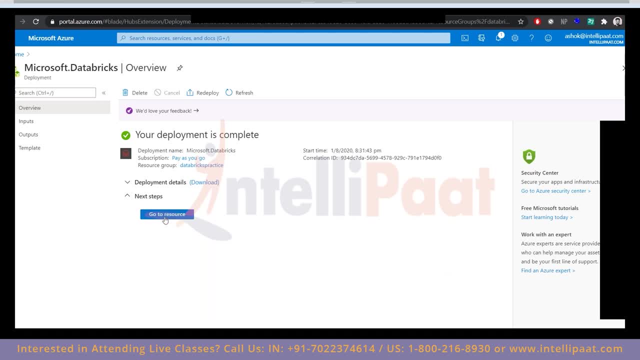 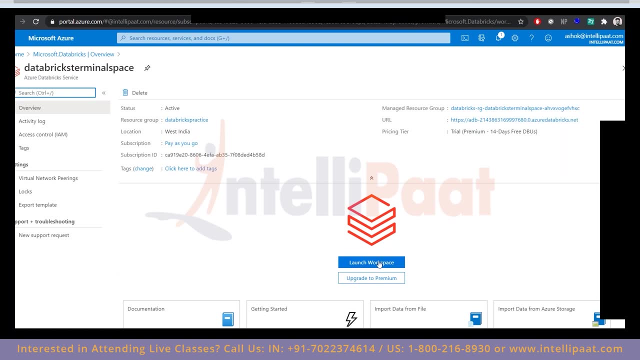 So Okay. So the next thing you will do is click on go to resource, right, Uh, so now we will launch our uh uh service. So for that, uh, click on launch workspace. I think there's one other step we have to do. 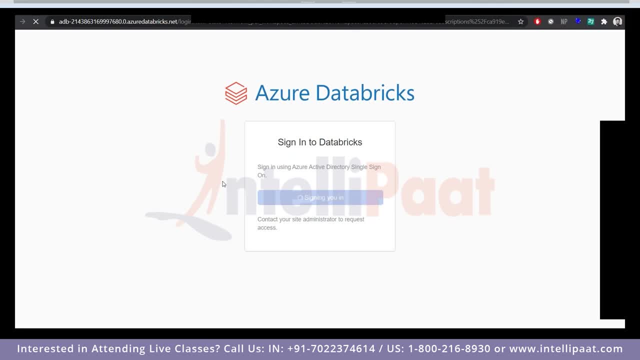 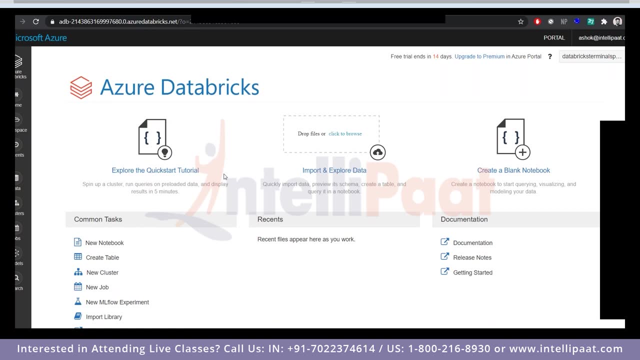 This will log us into the uh Azure Databricks- uh platform. So this is the very conveniently and well, uh well, wrapped around the terminal that you get. So a lot of things might seem familiar, Right, So we have these options. 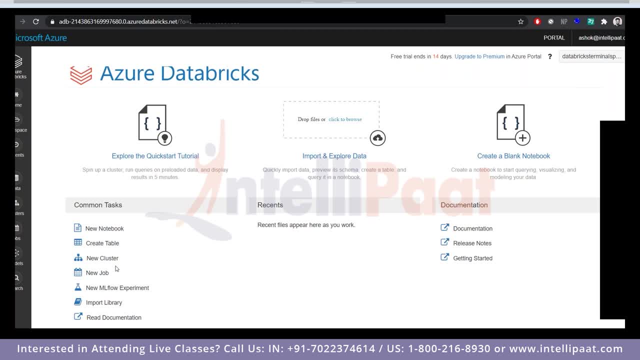 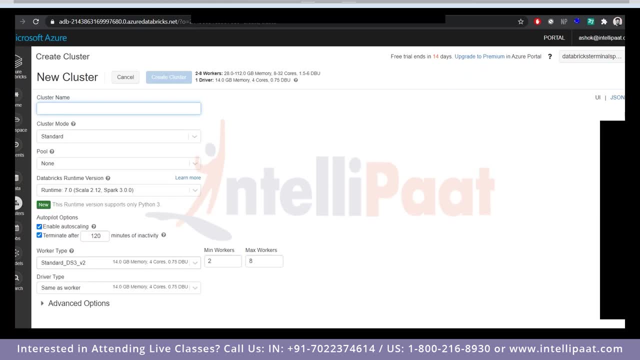 Uh, we can create a new notebook. so we can not actually do that. And why we haven't created a cluster? because we need something to run our notebook on, Right. So the first thing that we will do is create a new cluster, and now we can specify things. 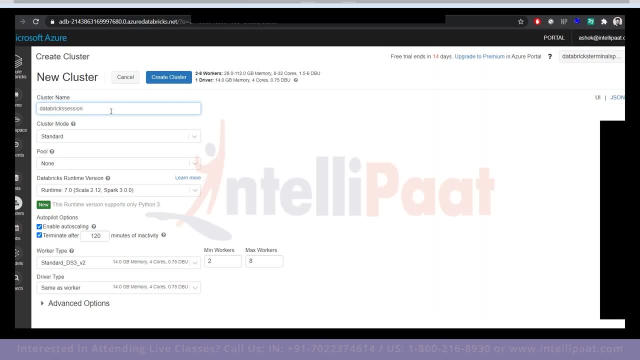 So let us just call this Databricks session. This is what the cluster is. Uh, the cluster mode would be high concurrency. So high concurrency happens when a lot of people are using the cluster at the same time, so that a lot of jobs can, a lot of jobs could. uh, the scheduling is optimized in high concurrency. 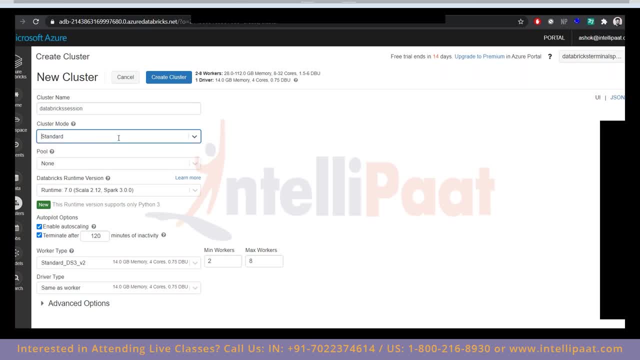 where the jobs are scheduled in the manner of resources in standard. When you're only using it for practice purposes, you would go with standard or uh jobs that are not that frequent. If your company doesn't have to do frequent jobs, then it would use the standard mode. 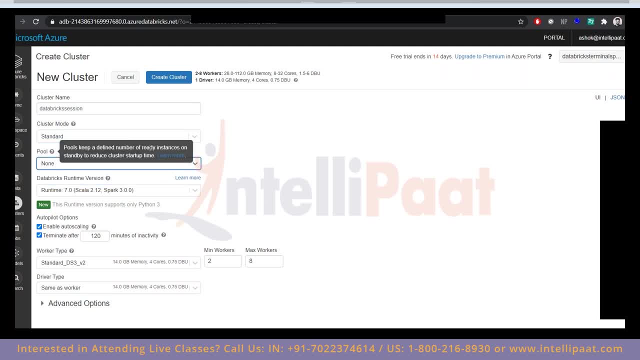 Uh, the pool is: uh, keep a defined number of ready instances on standby. It would use uh, cluster startup time. All right, So this is another feature. I haven't used this before. I think this is just a standby to reduce cluster startup time. 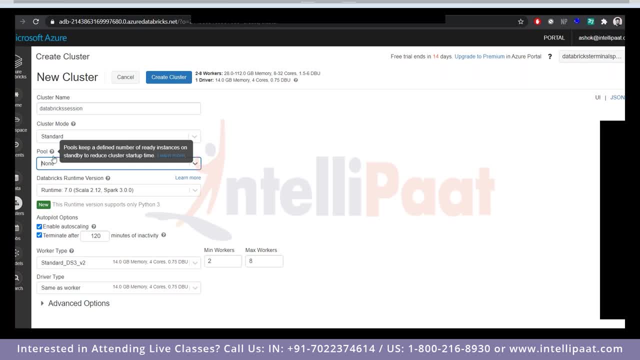 So it will preemptively start up the services. Uh, we can decide this past. uh, Scala and Spark version that we want, So there are a lot of options. Uh, right now we're going to use the stable one, which is 7.2. 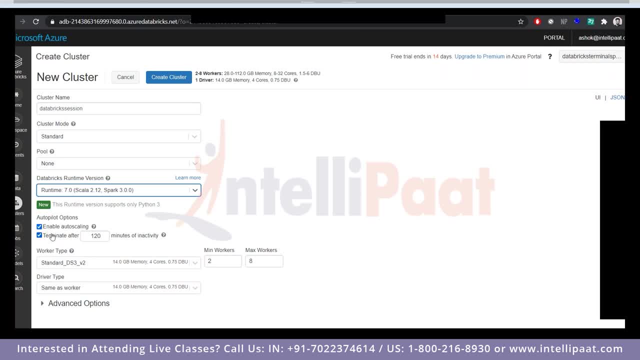 And uh, then we can also enable auto scaling or disable auto scaling. So, as I had discussed in the PPT, uh, in the minimum workers we can specify. in the maximum workers, we can specify So at the minimum, uh, in the minimum, when it's doing the most, uh, least required, uh. 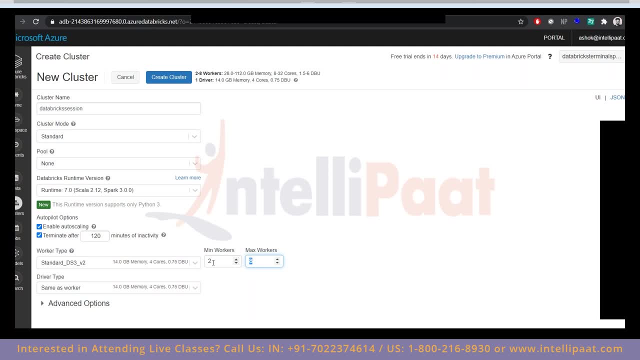 requirement- uh, uh, requiring job- then it will use the minimum number, Right, And when the workload gets really, really high, so it will get somewhere between two and eight. we can specify when you increase this to anything we want, right. 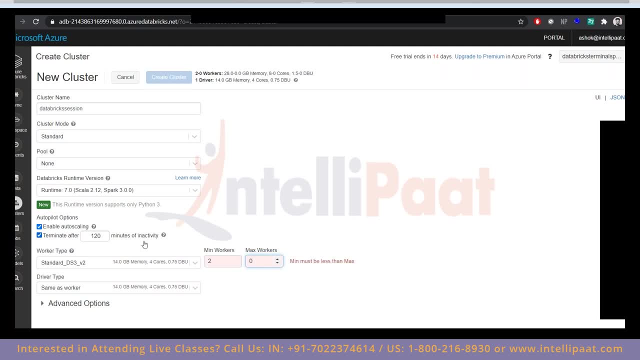 Obviously, the price would increase as well. You are actually using 17.. Uh and uh. if you are using it for practice, you don't need to enable auto scaling as well. You disable that and you specify one more. Okay. 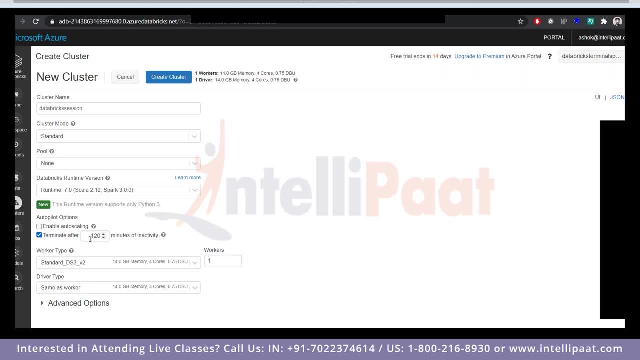 Right. So now you don't have to pay literally anything or terminate it after a dash minutes of inactivity. So if you're not running any commands on it, uh, and you've somehow forgotten that, you've like, Yeah, That is a resource, uh run forgotten you've logged out and you've uh went somewhere else. 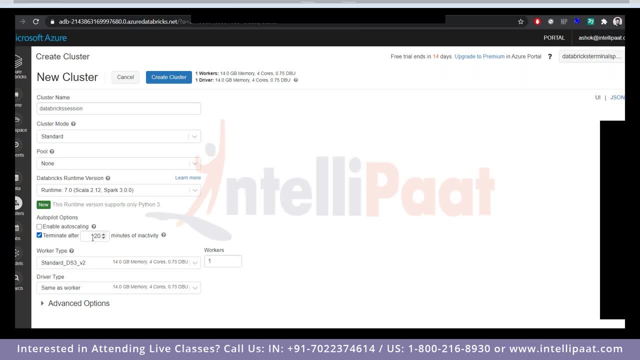 Right. So, uh, if you don't want to be charged for that charge for inactivity, because, uh, even though Azure will not cost you anything when you're not using it, what will happen is there is a certain amount of storage space in every instance that you're creating in the cluster. 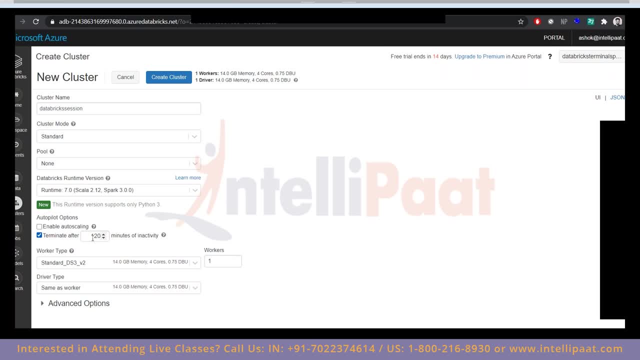 So that storage space is not entirely free. There's a nominal cost attached to it, but it's still there. So if you're using one worker it's negligible, but if there's, if you have 150 workers and all of that. 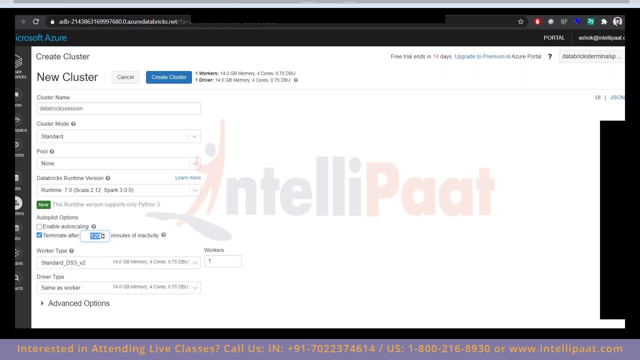 Right. So, uh, we can simply uh provide the minutes of inactivity, after which it will automatically terminate. The cluster will automatically terminate after that. So let's put it to uh something like 60.. Right, I'll just put it to 120.. 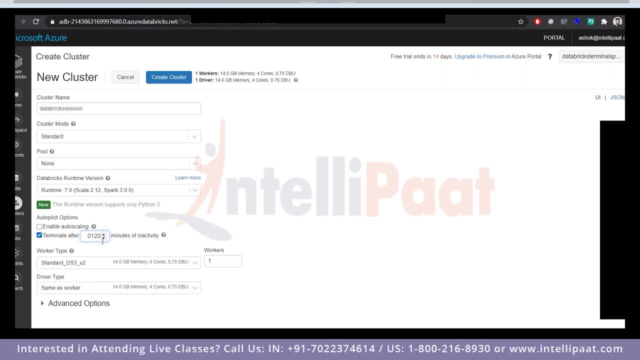 So let me do that And, uh, uh, we can choose the instance type. So there are a lot of like in AWS. there are a lot of instance types and Azure as well. So these are the instance type for the worker, what you want for the worker and the driver. 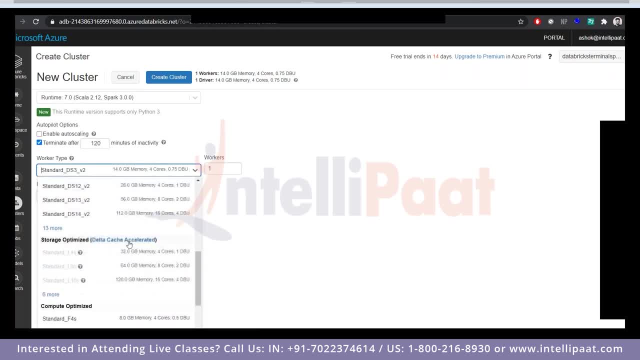 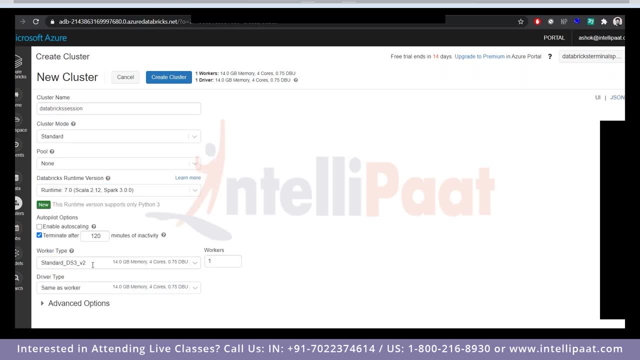 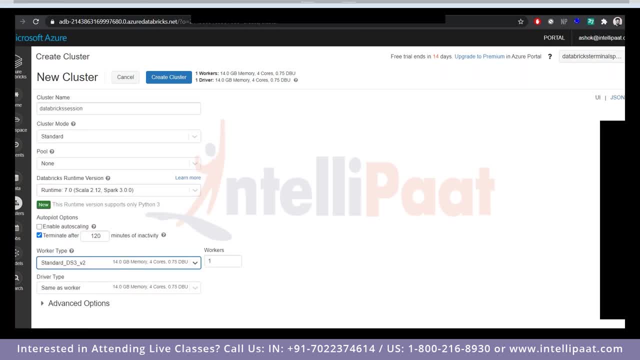 So memory means RAM and uh, yeah, this is uh, how much time it has, how many cores it has, Right, So you get that. So let us get with the default and the driver. uh, just let us same as worker because it's. 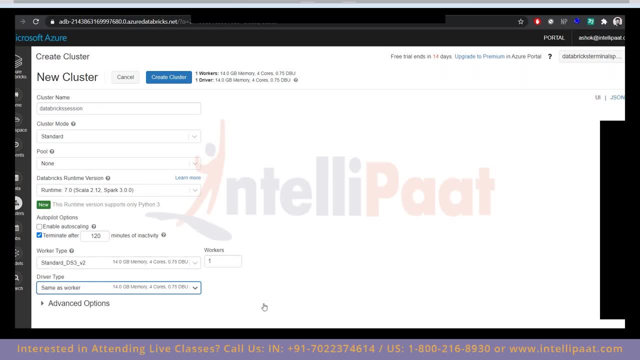 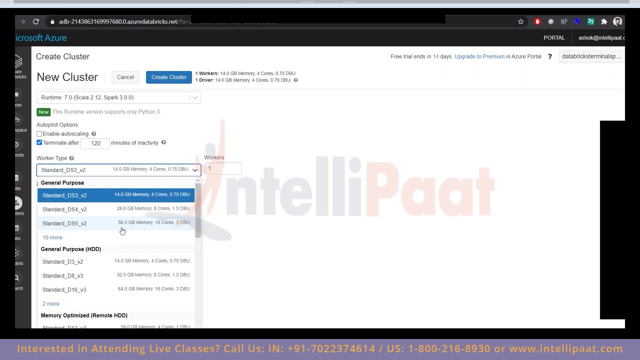 the minimum, bare minimum, the weakest possible instance where you use it. Right, But you can obviously, if you have a higher workload you can use higher instances with high memory. So it goes 56 DBs up to that much RAM. If you click more and there are more, 256 DBs. 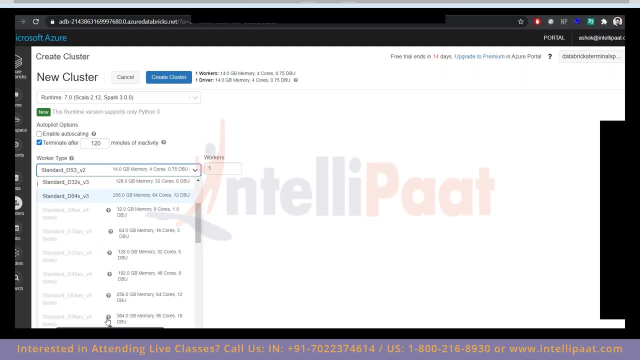 Yeah, And then in in the region that we are operating in, uh, we don't have these available. uh, in the West India, But, uh, you can opt for uh, uh, these if you choose another region, because we don't. 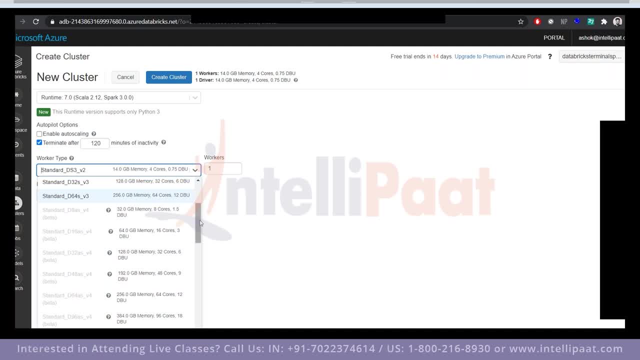 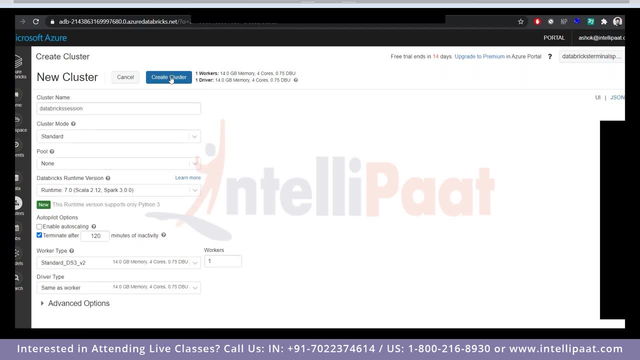 have that architecture and the Indian, uh, Indian server house or Microsoft whatever it has in Mumbai. um, let us know, uh, so we can click on. let me just check once. Yeah, So this will take some time to deploy as well. 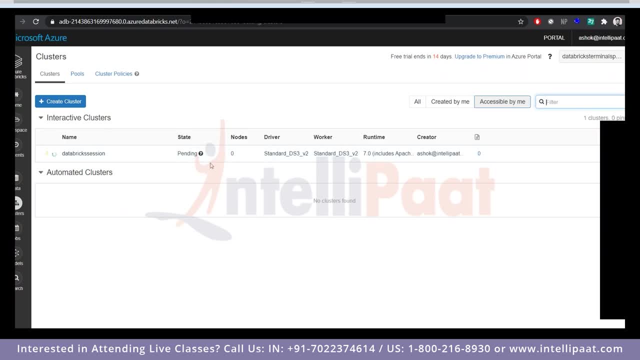 Uh, so we'll wait for that. So it's currently pending because it's being set up the the, the nodes that being initialized park is being installed on those nodes. those nodes are being added in the same cluster right. So all of that is happening automatically on its own in the, in the background, in the. 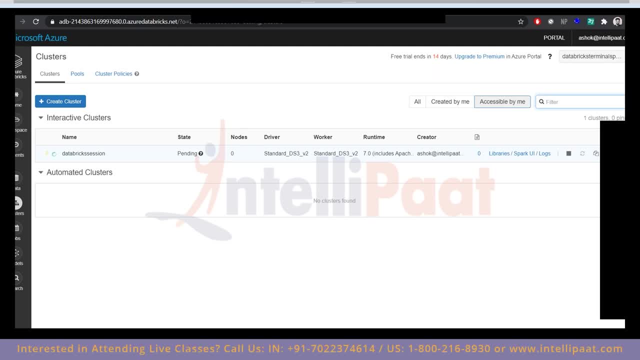 servers of a Microsoft Azure, and it'll even, once it has created, once it has resolved those resources and has installed Spark on it, then the state will be- uh, I think- running already And then we can use our cluster for our workloads. 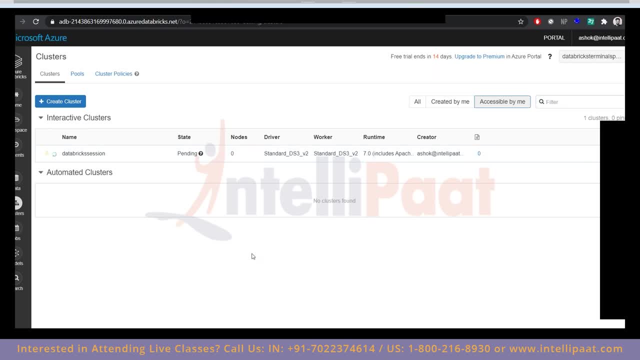 So we'll wait for that. So this pay as you go means it's not like monthly. there is no subscription charge or anything. It depends on how much you use. That's all. Yes, Yes, Yes, So workload depends on the workload or depends on the number of nodes you're using. 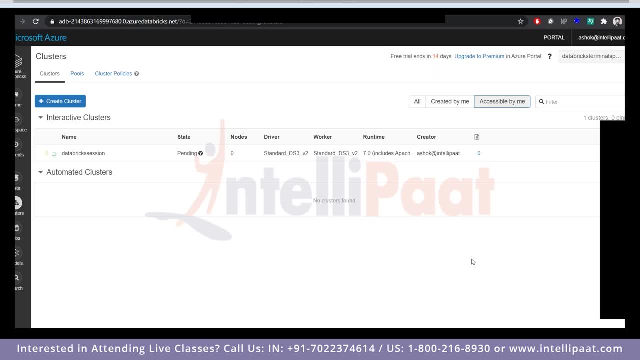 Depends on the number of, depending on the quantity of storage you've reserved for your cluster, And that is one of the key advantages as well. Right For using cloud services, say, if you're a business owner and you have big data needs. 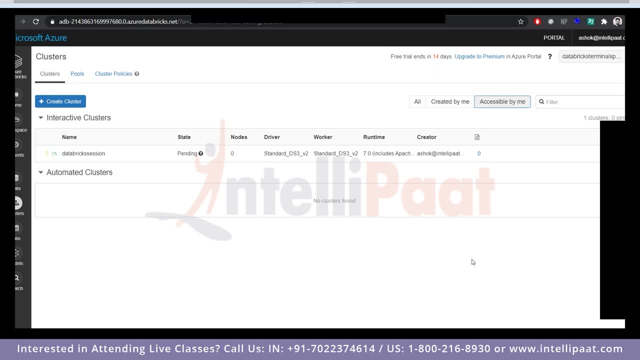 right. So, uh, you have two options. One is to use the cloud services right And the other one is to use the cloud services Right. So you have two options. One is to use the cloud services Right. So you have two options. If you use the cloud services, you only pay for the amount of users that you have. But if you're owning some hardware locally in your own office, then you have to. if you've rented it, you bought it. you have to pay for the entire thing. And then you have to pay for the electricity costs, You have to pay for maintenance. You have to pay a server administrator to maintain that server, to add any new cluster, add any new devices to it, add any new hardware to it, upgrade it. 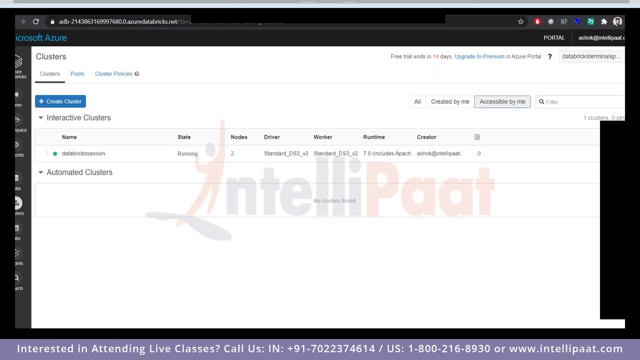 So this, all of this, is managed by Azure in this case? Yeah, So it's now in funding state And there are two nodes: One is to use the cloud services. The other one is to use the cloud services. Right, So you have two options. 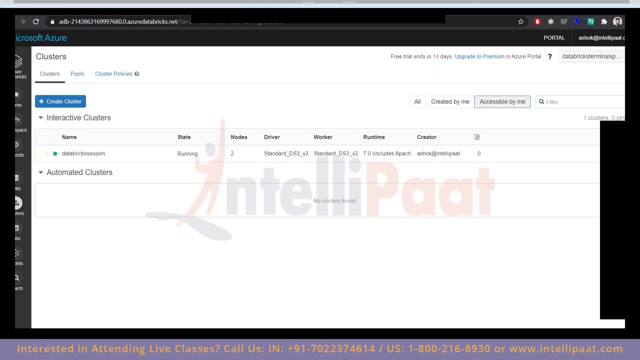 One is to use the cloud services. The other is to use the cloud services. So it's now in funding state And there are two nodes. One is to use the cloud services, Two nodes: The first is the driver node and the worker node. 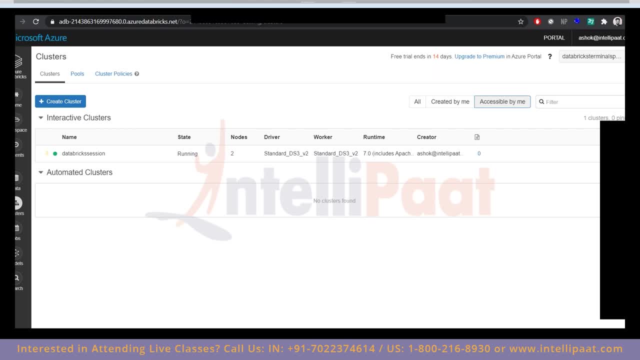 Right, All right, So we can now simply go to the Azure data picks And they have a new notebook option. Right, We can click on that and then it'll ask us which cluster we want to use. We will use the cluster, I think. 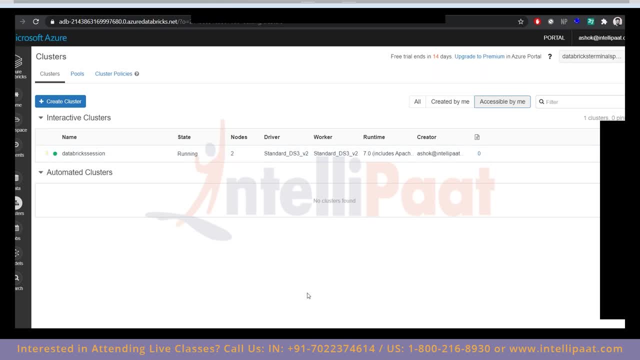 And it's going to type on the cluster. So we can go to the cluster like this Right, So we can click on that And then it'll ask us which cluster we want to use. And again we can go to the cluster and we can see a lot of different un-plugged data. 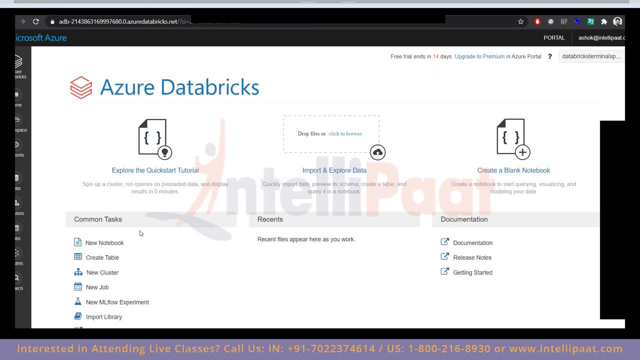 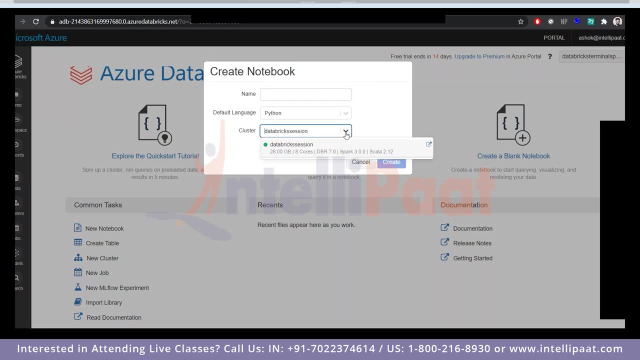 picks generally go to the Azure Databricks terminal, and here is a new notebook option. right, We can click on that, and then it will ask us which cluster we want to use. We will use the cluster that we just created. Yeah, yeah, So it's there in the 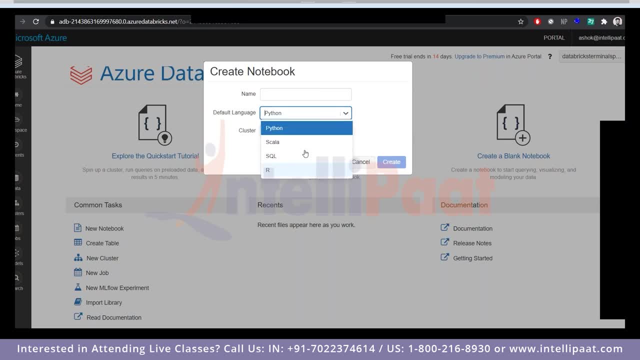 options And we can select the language that we want to start our notebook in. So I'll select Scala. Okay, Right, And then we can simply call this notebook anything. Let us call this Databricks notebook- And click on create, So this will start. 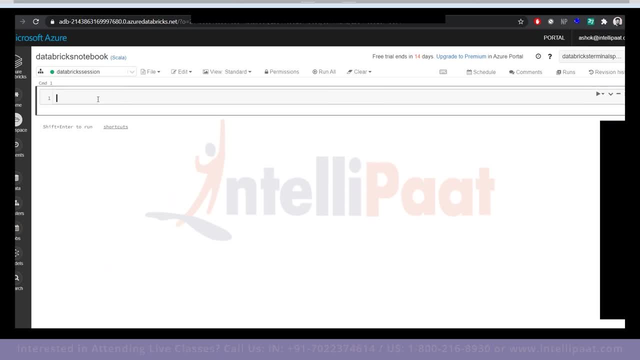 almost immediately. right, It looks like Jupyter Notebook. Yeah, It's just like Jupyter Notebook. You have to press shift and enter to run every command, and then you can add new code, blocks and all that, Okay, okay, So now what we will do. 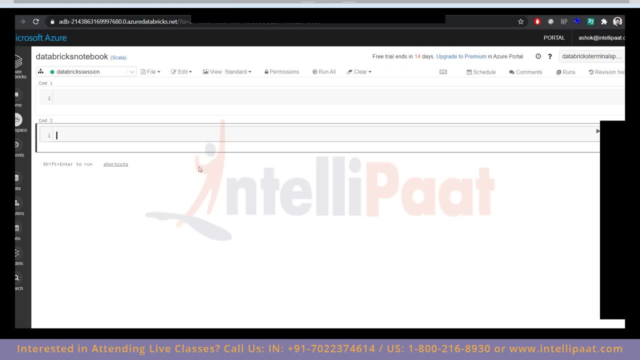 I will tell you how to upload files and integrate this notebook with a storage platform like an Azure service, a different Azure service. So we're going to be using Azure Blob Storage. So this is like Amazon S3. It provides a storage service to you- Azure also. 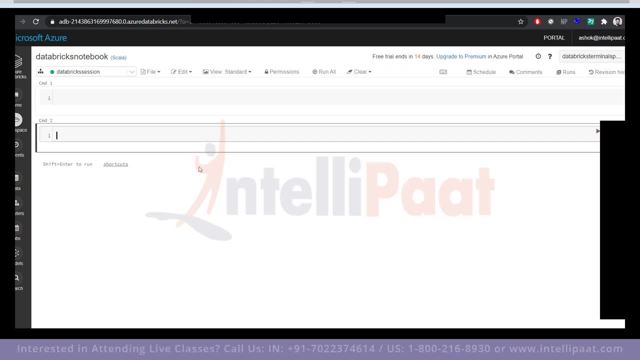 provides you with a storage service, which is the Azure storage accounts, and you can create data containers on it And then you can use those in your various Azure service packages. Not just with Databricks, you can use it with other Azure services that. 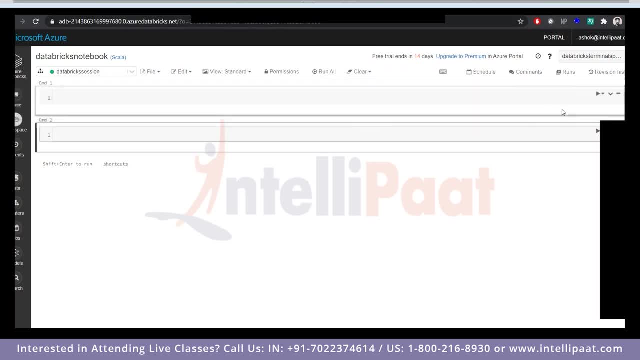 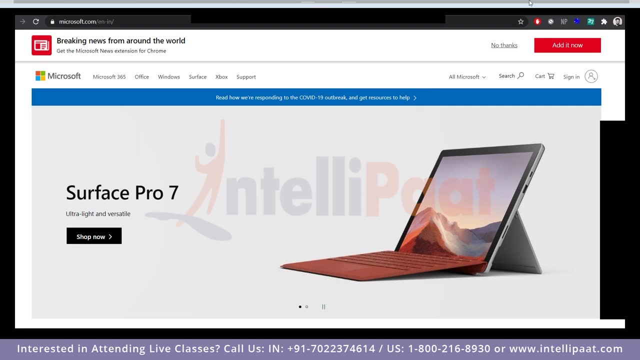 use it as well. So let us go to the Azure dashboard once again, because it is not part of Databricks. what I'm going to be doing right now, It's not from here. Actually, there's a UI element for the go-to. 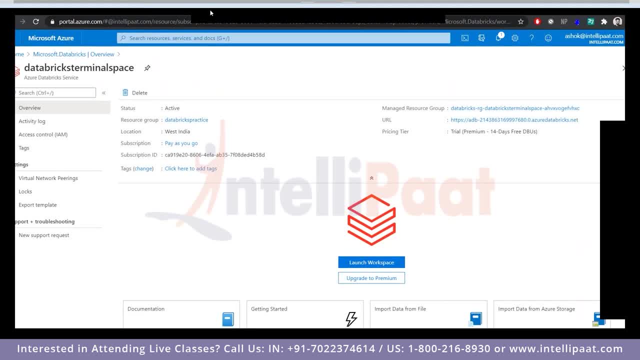 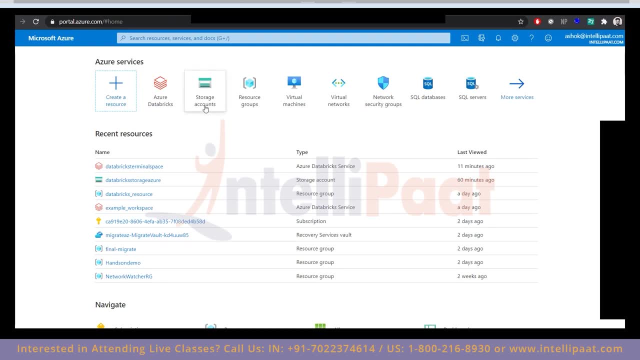 meeting thing, So that is why I'm not able to see it. I can see my tabs, So this will open that up. I'm back in my portal, right From where I can launch all of the sources. So this is storage accounts. 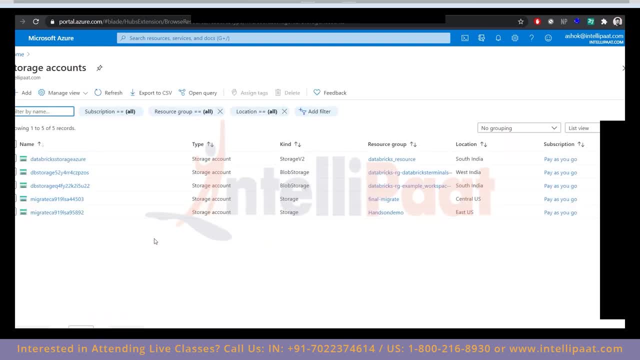 You will click on that because you will be adding some. you will be requiring store something, right? So these are already created by my peers and everything. So these are. some are big storages, some are blob storages. So, depending on whatever everybody is doing, say, 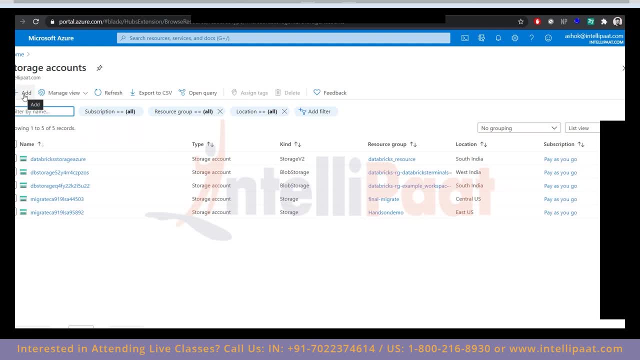 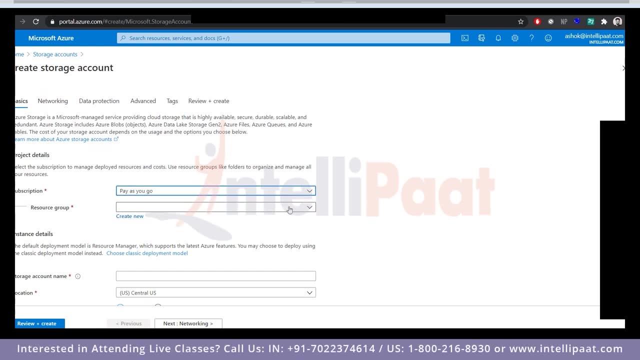 they create that And you can create your own. Click on add. So, as I was discussing before, the pay-as-you-go remains as it is, because that's the only option, And now you don't have to deal with any permission issues, because once you click. 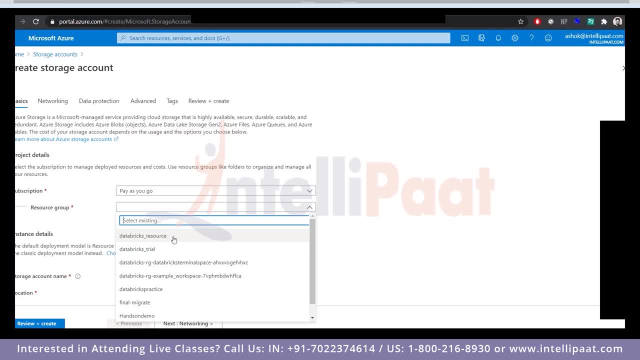 on drop down the menu of resource group, you can just find the resource that you've created. So all of the permissions are already intertwined. right, You don't have to go and allow. you don't have to create some sort of IAM role like. 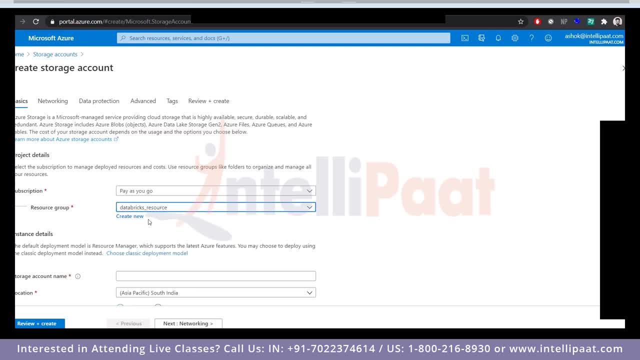 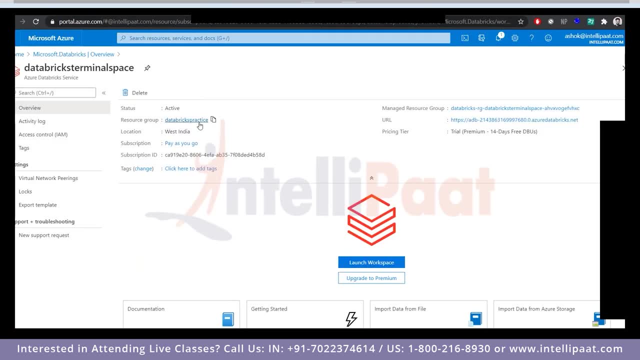 you would have to do in AWS to integrate. So Databricks resource, I think it was that, And simply check it over here. So resource group: Databricks practice. It's not- I think it's not- Databricks, whatever it was Okay, okay. 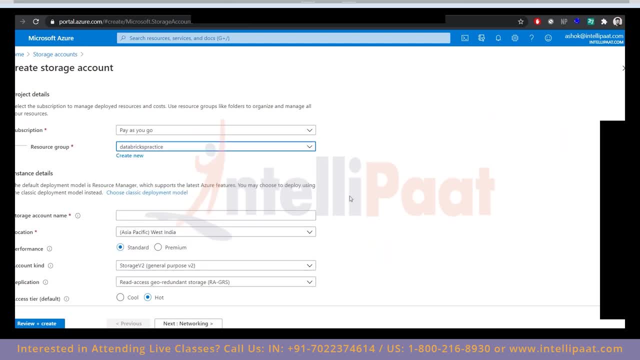 Databricks practice: Yeah, it is this one. Ah, that one. yeah, Okay, So you can name this anything you would like. Let's call this Databricks session storage And the location. it is better if you keep. 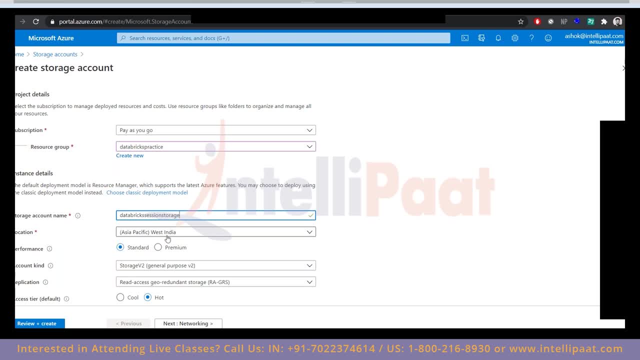 the location same for latency reasons. You can keep it different if you want, but it will take a longer time to say. if you're analyzing a lot of data right, which requires immediate, precise, low latency transfers, Then having something in the something being 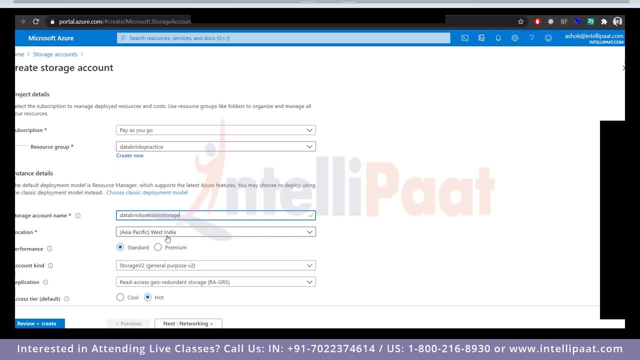 in the US and something being in India. it will take some about two seconds to actually request and respond. Yeah, So that is not a good case And account you can choose anything. So we are going to be using general purpose. The payment is not an issue over here. 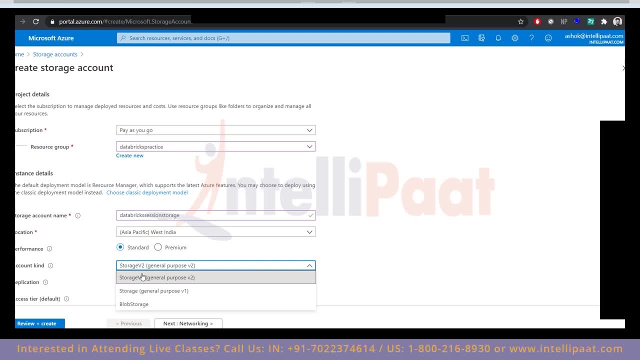 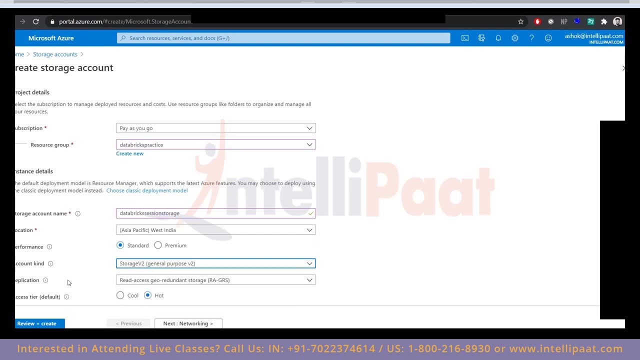 Because it entirely depends on how much data you're actually uploading, right? So right now I'm just going to be uploading a megabyte of data. It's not going to cost me anything. I can use the B2.. And just put it. 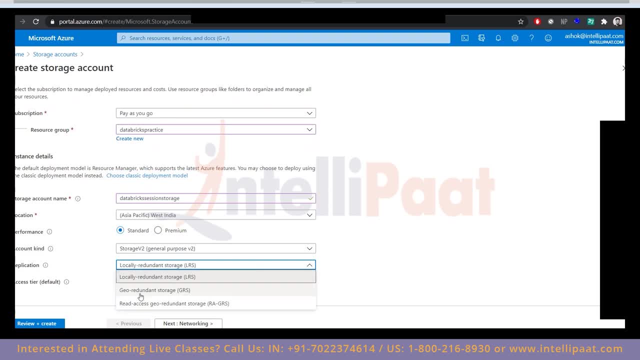 replication, you can put it to locally redundant. So the difference between geo-redundant and locally redundant is that geo-redundant, the data is replicated across regions. So in West Mumbai there would be one instance of that data. Yeah, 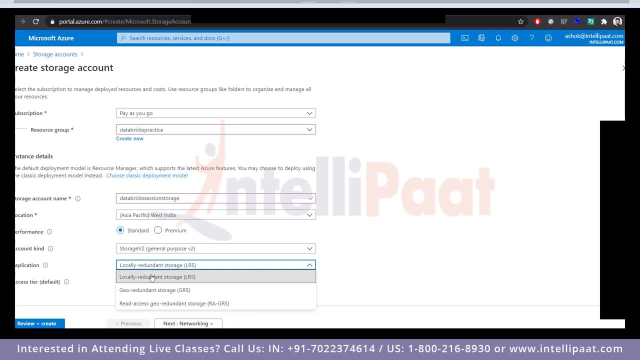 And in the US region there would be other instance, for what not? So that is something that storage accounts would manage automatically, But in locally redundant, what will happen is it will for our use case, because we are not dealing with any data, that is. 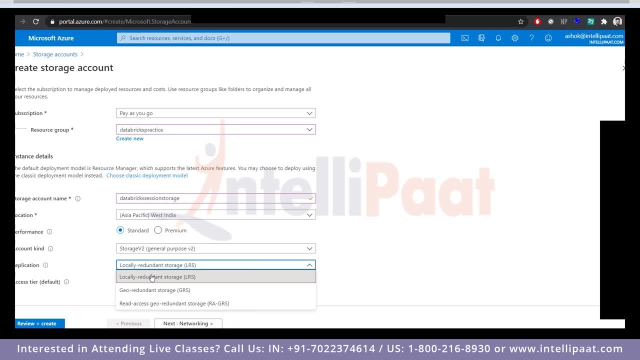 that we are fearing to lose. that would cost us money if we lose it. We don't need that sort of a need, that sort of a backup or that sort of a use case where multiple, from multiple places, people are using the storage service. 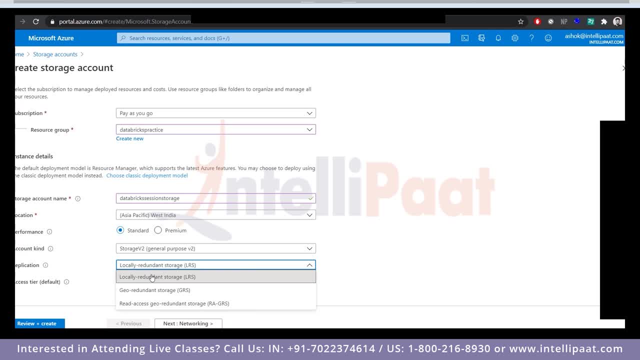 That is not the case in our case, So we use locally redundant Where the data is replicated, but in the same server space, Like it will be replicated three times in Mumbai itself. Yeah, So we are going to be using that And the access. 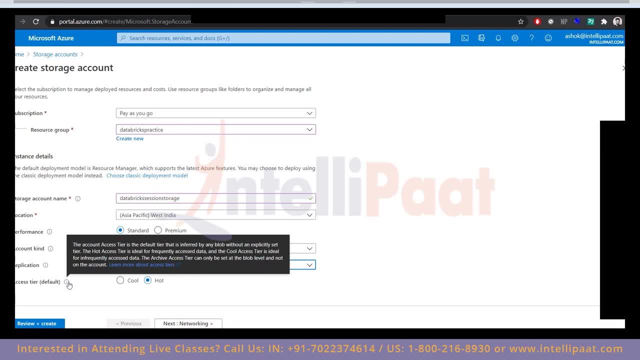 tier. you can simply look at it. So the account access tier is the default tier that is inferred by any blob without any explicitly set tier. The hot access tier is for ideally for frequently accessed data, and the cold is for when you don't. 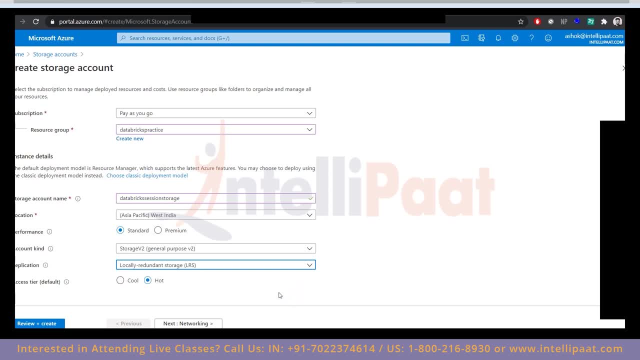 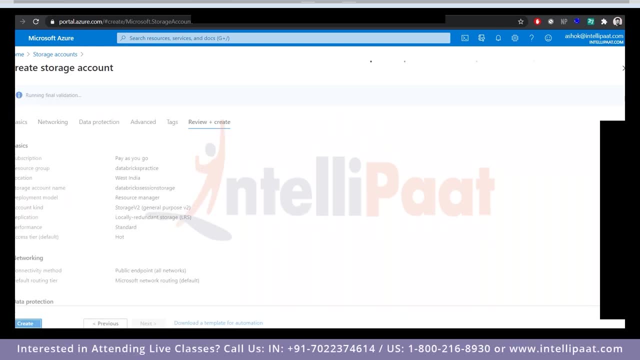 have to access that data frequently, So not a pricing issue in that case for our use case. So let us click on create and review. So review all of the details. I think they are right. West India data storage And then we can click on create. 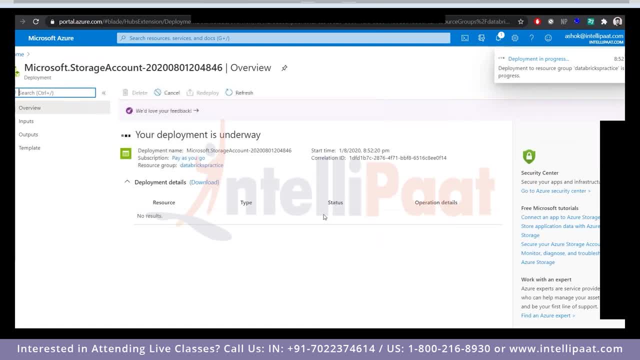 So this will create our storage account. Now we have to create a container within our account, So let us wait for the deployment. So those settings we can change if we want. is it? Yes, For example, that hot to cool we can make if we want. Yeah, 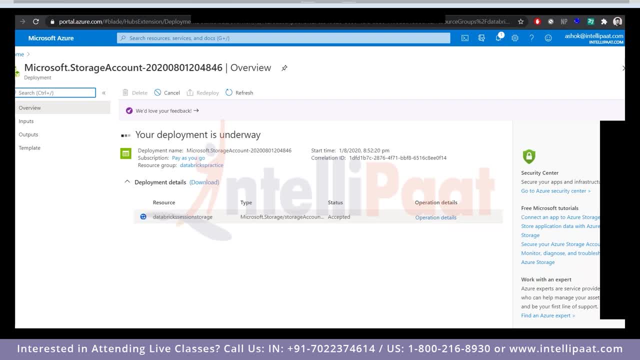 So say that your organization deals with the data analytics but it does not deal with it in real time, Like it doesn't want it, like on a minute to minute basis, right, So you want it on a routine basis. They say: your tool, whatever you assign. 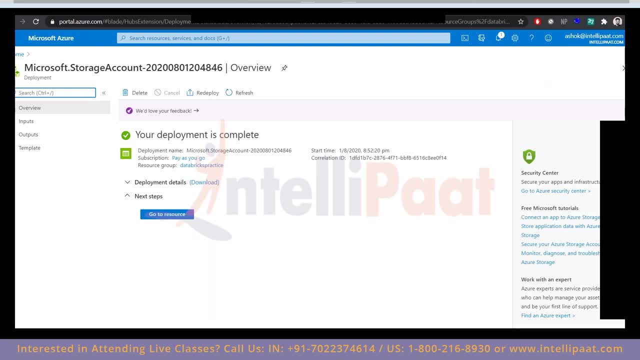 whatever your code is, it checks for the data every six hours, right? So your storage service could simply be a cool storage service where, if it's being checked every six hours, so I think there's some sort of configuration assigned to it. The request and response is pricing is. 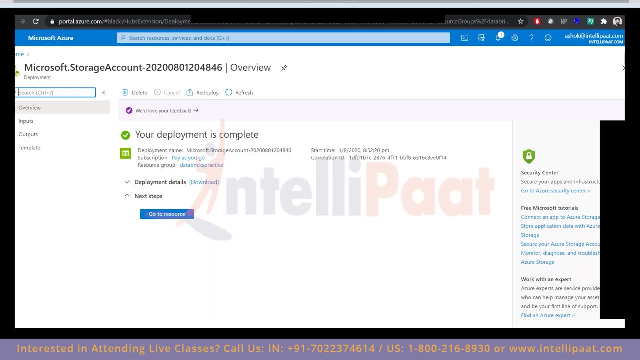 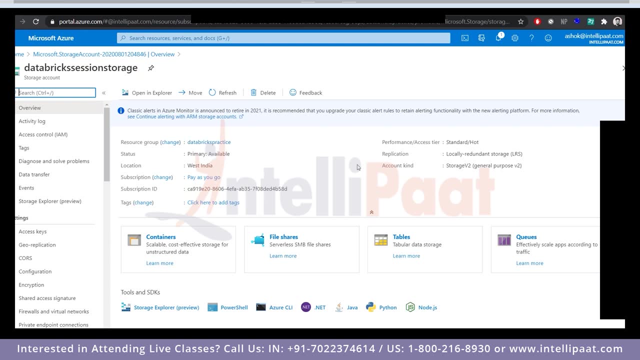 adjusted according to that. So the deployment is complete and we can go to the resource now. So all of the permissions are automatically managed just by using the same resource group. We don't have to worry about that, And now we can create our table- not a table. 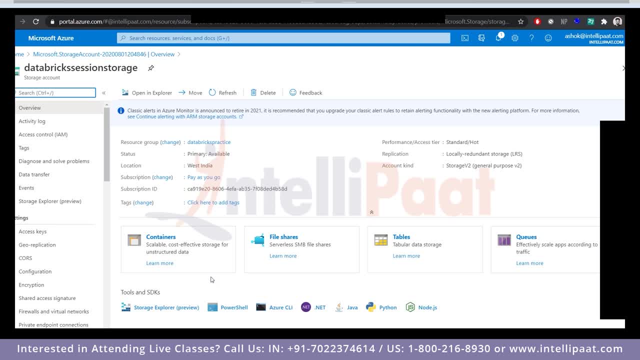 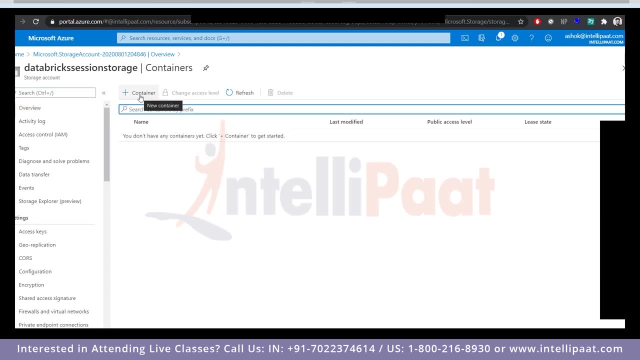 but our container where we will store the data, similar to how we would store it in Amazon S3.. So click on containers when you opened up the resource And now we can simply click on plus container. So add a new container And then we can name. 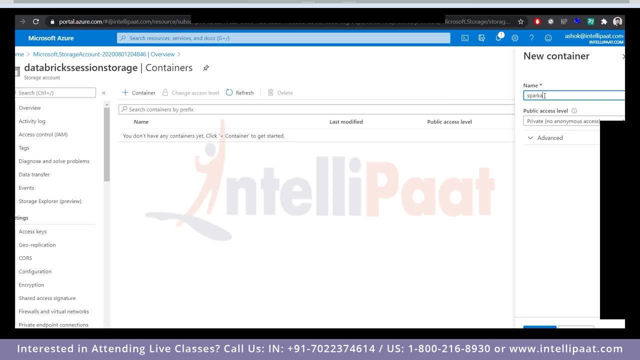 this container anything we want. So let us call this Spark assignment And let's click on create. So we have it over here, right? So let's go back to the presentation forms and get over these topics a little bit. So we have. 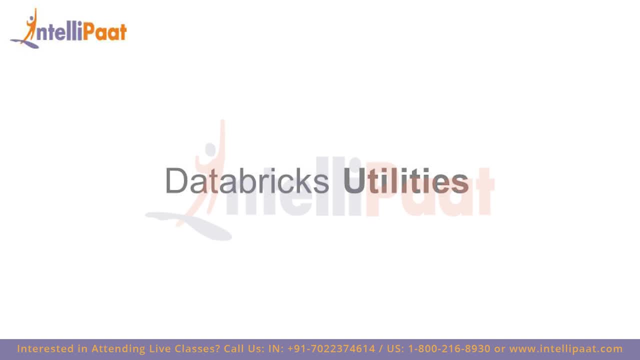 Databricks utilities. So these are. everything is virtually the same, And you are using Databricks and Spark. Everything is essentially the same. The only new thing that is there is Databricks utilities. So these are additional utilities. They are not. 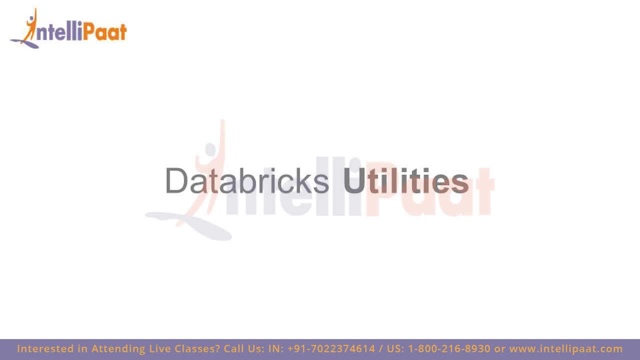 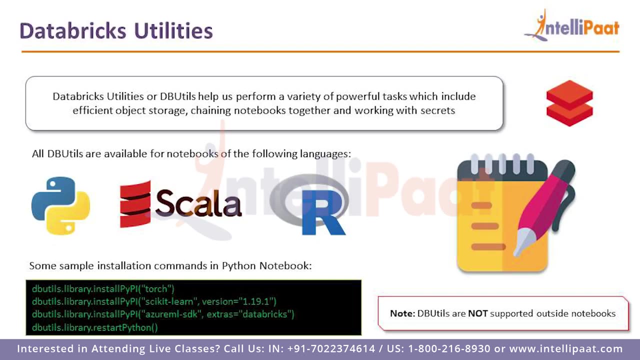 exactly libraries. These are utilities that are provided to you by Databricks, not by Microsoft. This is not a Microsoft thing. This is just a Databricks thing, right? So it is basically a utility to operate within a cloud environment, right? So help us perform a variety. 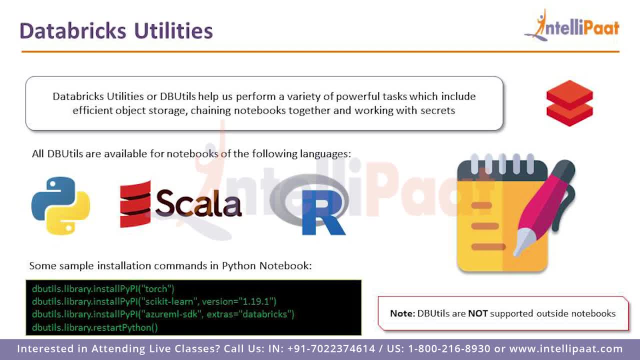 of powerful tasks that include efficient object storage, chaining notebooks together. So you have commands in various notebooks that you want to chain together for your particular use case. You can do that. So all of this is provided to you And you can see on the bottom we have 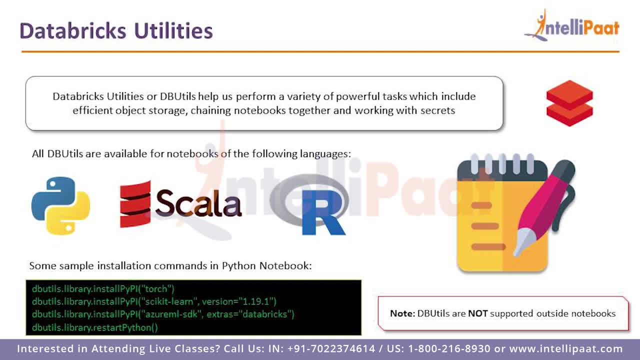 commands right, Like: install pypy torch. install pypy, like it learned. So you simply have to write that one command. It will install it within your workspace. So, since this is not, you will not open up Apache. Spark, You will not write a Spark. 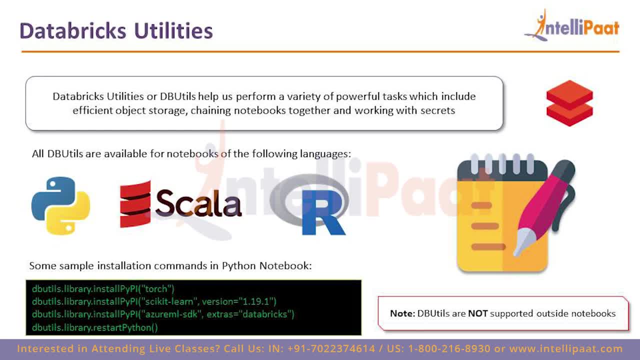 code and type installation commands right. You will not do that. You generally write what you have to implement for the data, right. So you definitely need something that would help you configure your workspace right. So that is what DB Utils is used for. 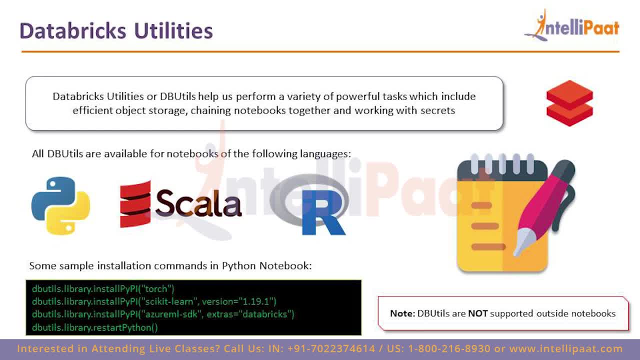 I hope you get the idea. So these are not supported outside notebooks. You cannot use it with the putty right, Obviously, because since you've used Spark with putty or anything, you would have not noticed that there's something called DB Utils. This is specifically for notebooks. 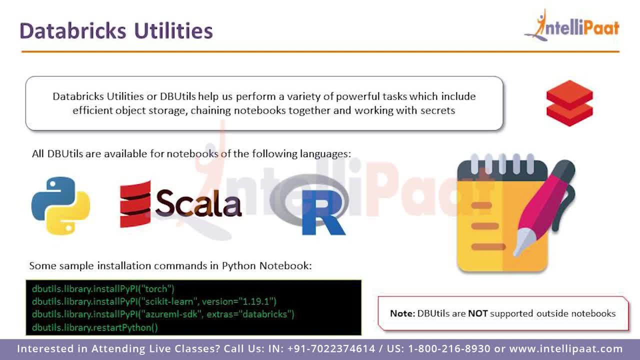 So the DB Utils are available on three platforms: Python, Scala and R. The difference in Python and Scala: if you create Python and Scala notebooks, the advantage is that you would be able to use DB Utils as a file system utility as well. 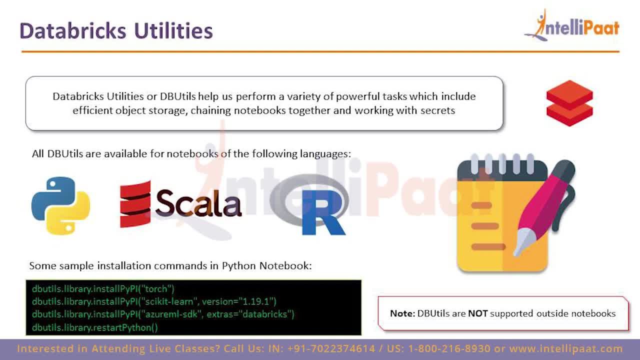 where you could manipulate the file system of your cluster nodes With R. DB Utils does not come with a file system manipulator. You can only use the other features, like installing particular packages and whatnot. R is a limited language, not much of a development language. 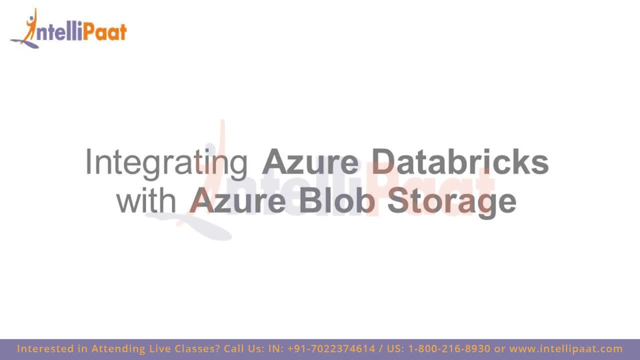 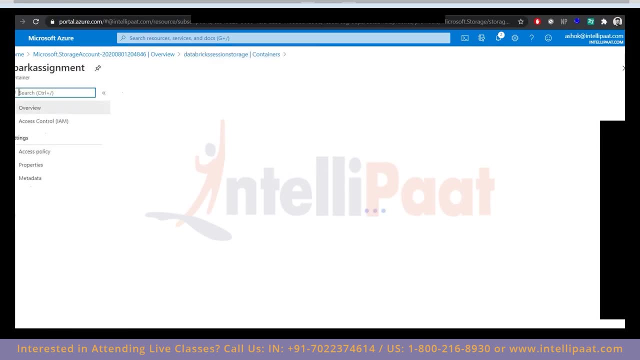 Let us integrate it now. Go back to the webpage. So now we have our container created, We can simply click on this container And we can click on upload. So this would open up my Windows file system. I can select a file that I want to upload. 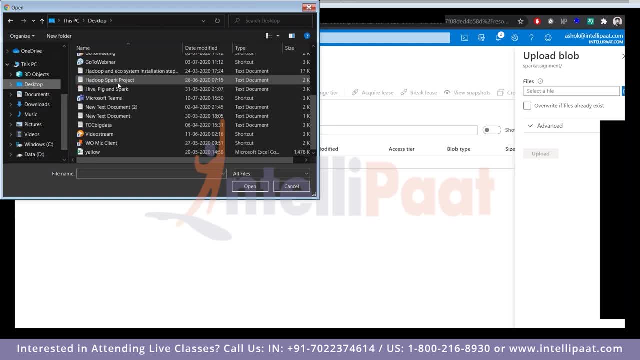 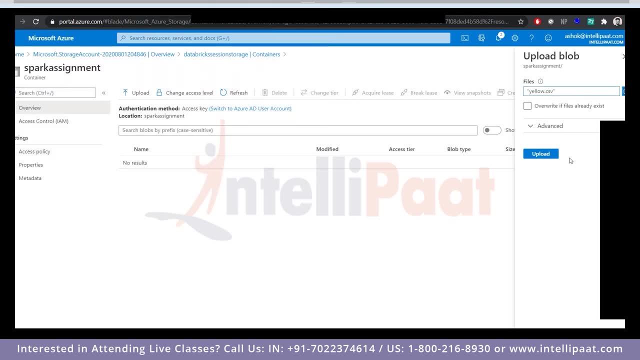 Let me go to the desktop. So I have this file, yellowcsv- already there. It's a csv file. I simply add it to my files And then I click on upload. So it's a 1.44 MB file. so it. 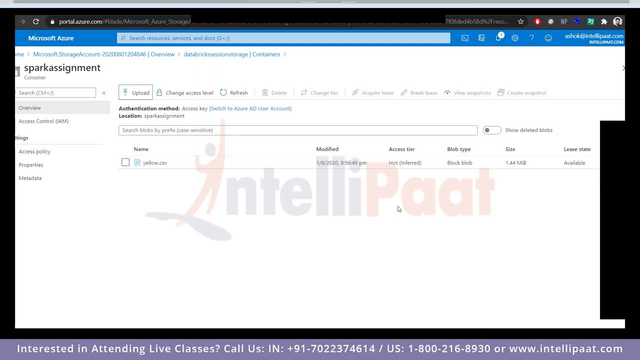 uploaded instantly. But you can upload larger files as well, but it will cost you a lot. If you are uploading extremely large amounts of files, it will cost you more. So that is how the pricing works here. 1.4 MB comes in free tier. It does not cost you anything. 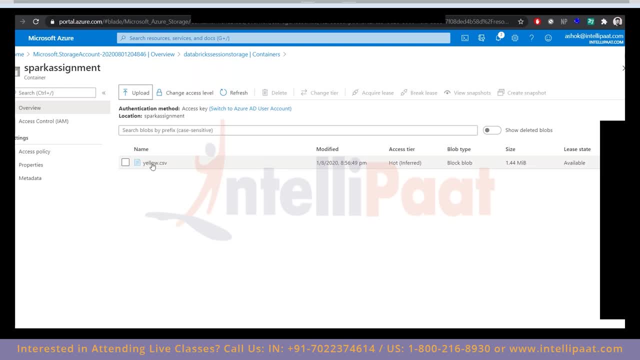 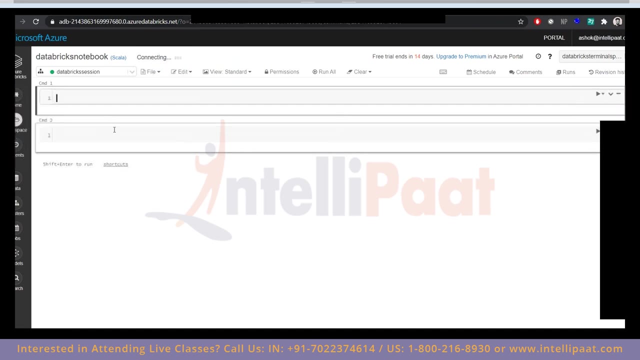 So we have this Now. we need to integrate both of these. We have our data in place and we have our notebook in place. We need to integrate now. So let us go back to the notebook. So we are back at the notebook. 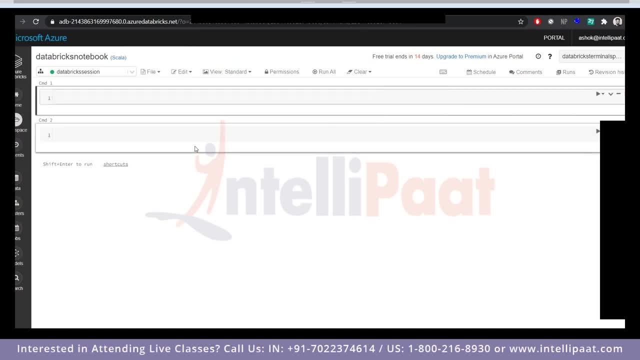 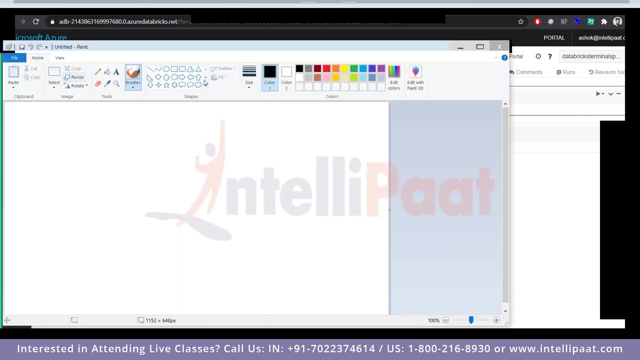 One small thing. I just want to know the hierarchy. So the workspace is like the top level, is it Under workspace container comes, or how it is Okay, So, let me, Okay, So this is how it works, right, Yeah, So you. 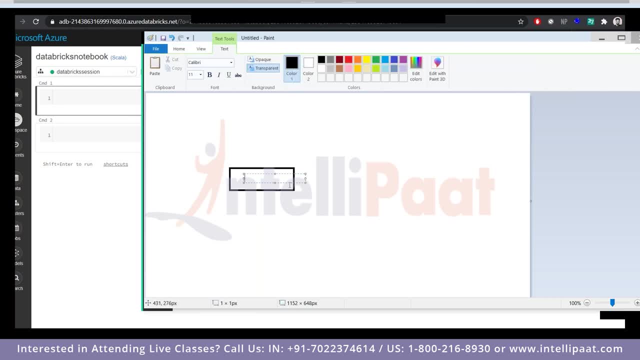 have your Azure terminal over here. This is your Azure terminal or Azure Dash Azure service, basically Datapix service- It's called Datapix service- And on the other hand, you have your blob storage or container. Like this is your storage container: 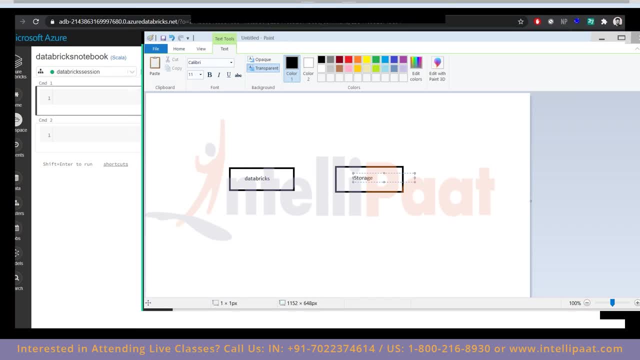 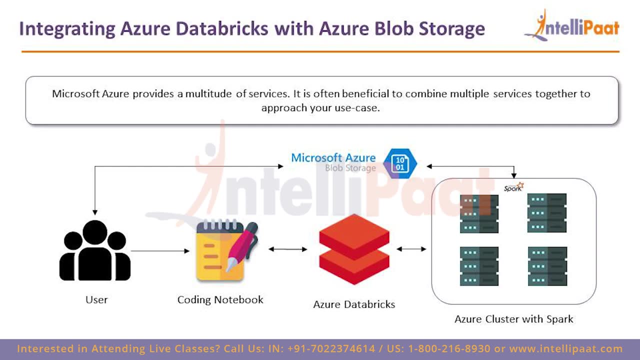 Actually, I have the diagram for it. I just forgot about it. I made this, Okay, So this is how it works. I apologize, I was actually making a mistake. So this is how it works. Okay, So there's a. 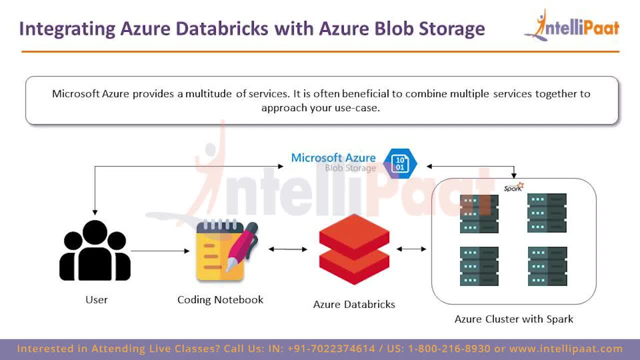 multitude of services and you need to combine. So it's often beneficial to combine multiple services together to approach your user. So you are the user right over here, Right? So there are two things you're interacting with, right. You have two things with direct access to. 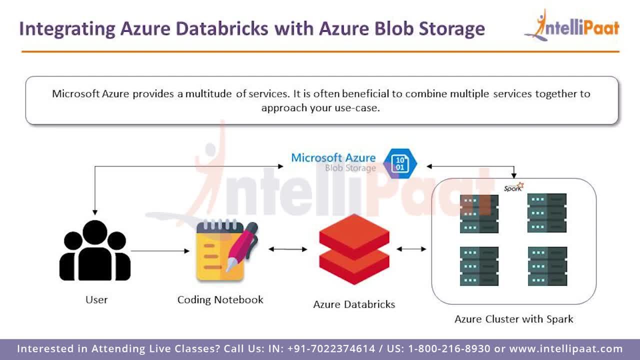 two things right. So right now we opened a separate service, which was the container service. So this was the Microsoft Azure blob storage. Right, We uploaded our file. So this is up till here we are interacting. right Up till here we are interacting with this. 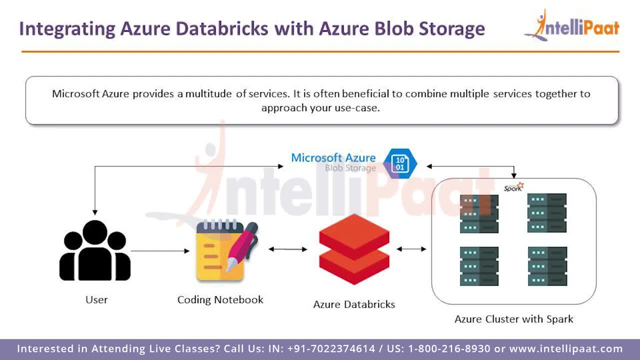 So this part is not our concern. This part is not our concern. Okay, And then Azure Datapix: we interacted, We created our coding notebooks, So this is what we're interacting with. So now all of this is not our. 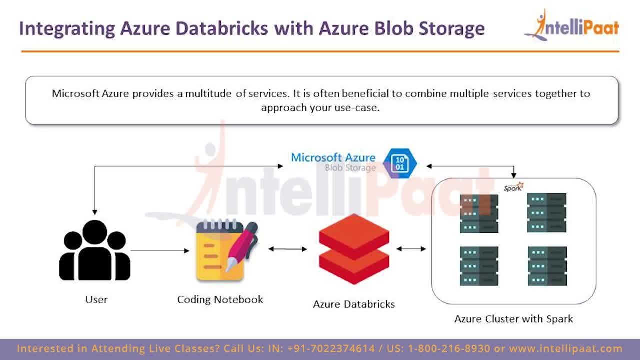 concern. right, So this is all happening in the background. The coding notebook will interact with the Datapix service and the Datapix service will interact with the cluster we've created. Right, Yeah, Okay, Depending on the instructions we're giving in the coding notebook. 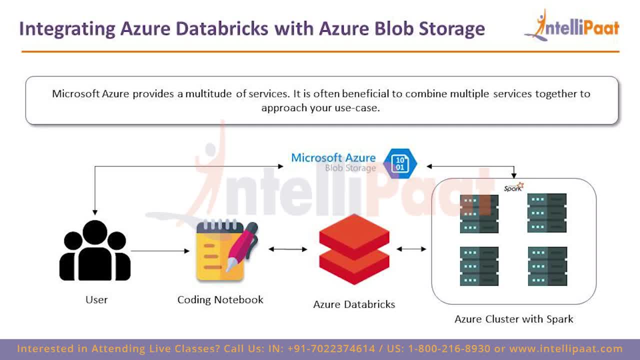 right. So it will get compiled or parsed. whatever It will go to Datapix. Datapix will send that instruction to Spark and say it's saying: take that data from Azure, Azure blob storage, Take that data from this location from. 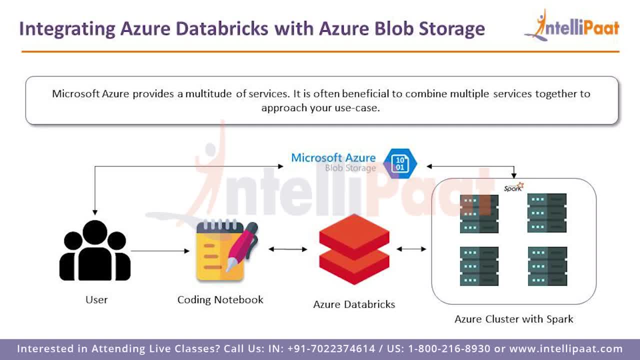 blob storage. The information will be processed, probably by the driver node, and it will basically ask the blob storage for that data And since the permissions are granted, it's in the same resource group. There will be no permission issues. Blob storage will simply grant access to that data. 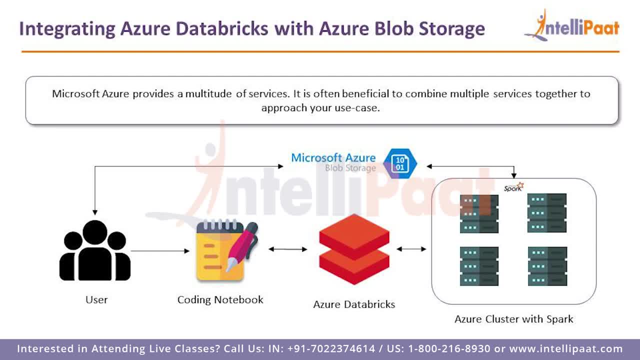 And we'll get that data in our cluster. So we now the cluster, will give that response back to Datapix and Datapix will simply get the output sort of thing that we get in every time we execute a code block in a Jupyter notebook. we get some. 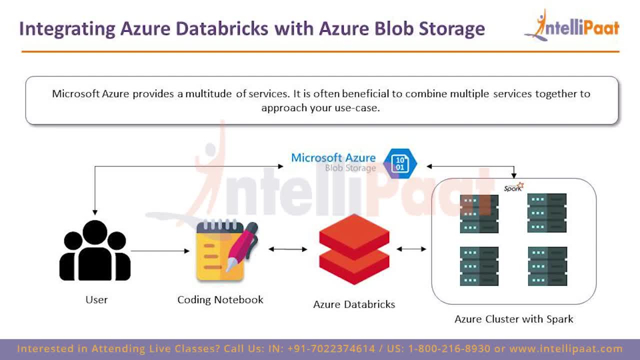 sort of an output tab, right? So we get that postback instruction, that, yes, we've received the data. It's been loaded into an RDD or whatever we've created Where this logical workspace came into picture. what is its boundary? I didn't get that. 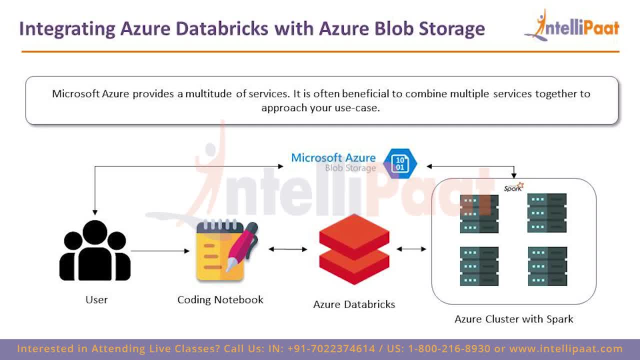 For example, my question I can rephrase: Can I have one workspace- and many I can. can I access many different storage containers? Yes, yes, Definitely. So this is just one instance of a blob storage. You can just have another blob storage on top of it. 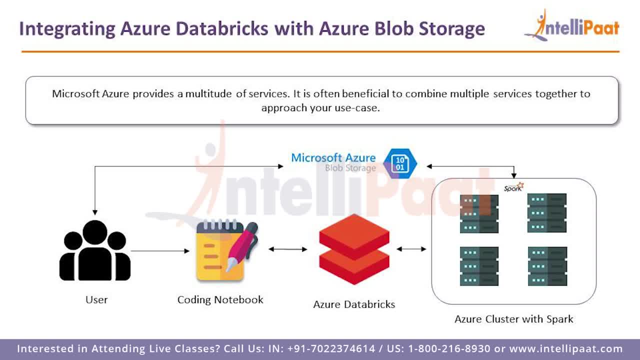 that you can access separately, Right, And you can access it with the coding notebook as well, As long as it is in the same resource group as our cluster, Right? Ah, okay, That resource group binds everything together, Okay, Yes, yes. 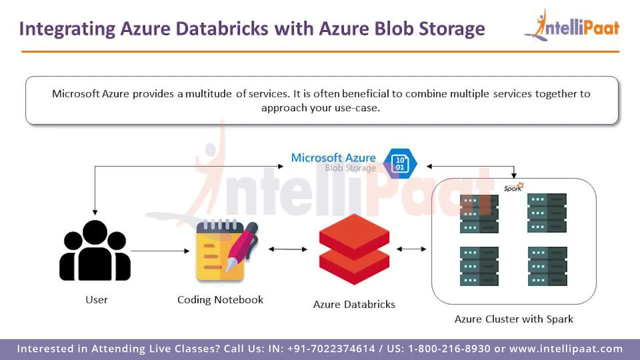 It is very essential that everything is in the same resource group, Otherwise you have to do a lot of configuration to get past the authentication and everything. Data security is a very prime concern with these big organizations like Amazon, Facebook, So it's very essential. 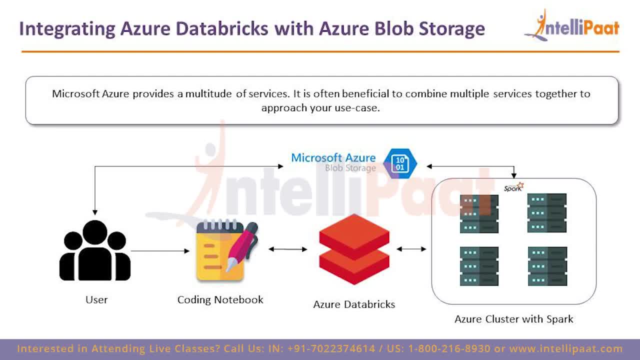 that the permission thing is matched. So then I would create more than one workspace, for example, for different clients. is it Like to give an example? One workspace I will create for one client, another. Am I talking in sense? 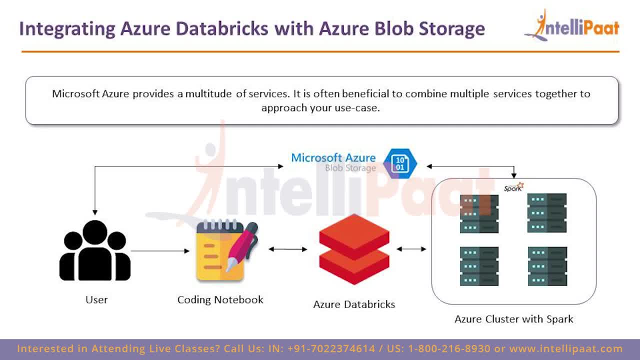 No, no, That's not an issue, I think. say you are working as a data analyst, You are not working as a data scientist, right? So it may be the case that you will not have access, particularly to the data scientist's workspace. But 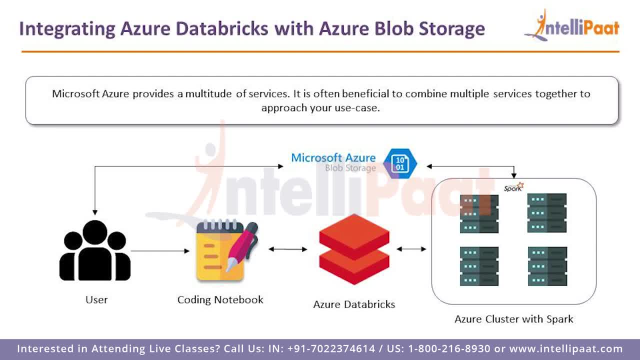 the data scientist could have the access to your workspace, right? Okay, So those are things that can be configured And multiple workspaces are created. Say, the data analyst workspace is there, So the only thing that the data analyst workspace will contain, you launch your workspace. 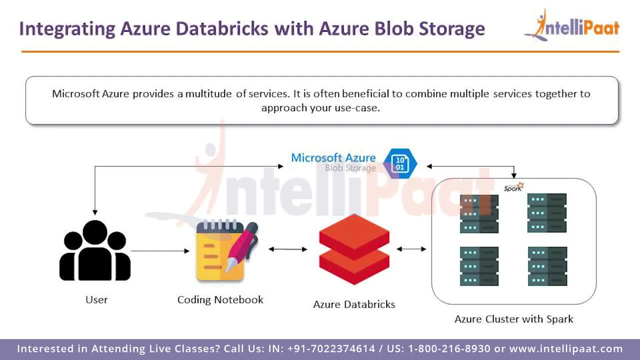 and you only are creating notebooks, which are related to data analytics, not to machine learning, AI or data science, right? So this workspace is something only for the code, is it? Yes, yes, Exactly, Okay, okay, It's like any. 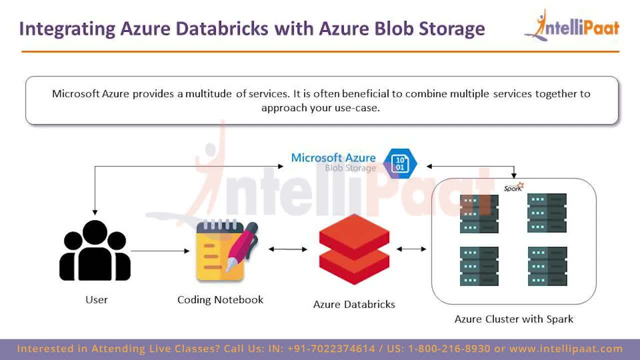 Eclipse workspace, something like that. Hopefully, yeah, Okay, yeah, You can go ahead Or you could go about the assessment. There are various ways you can implement it. It depends on the organization entirely. Say, the data analyst group contains all. 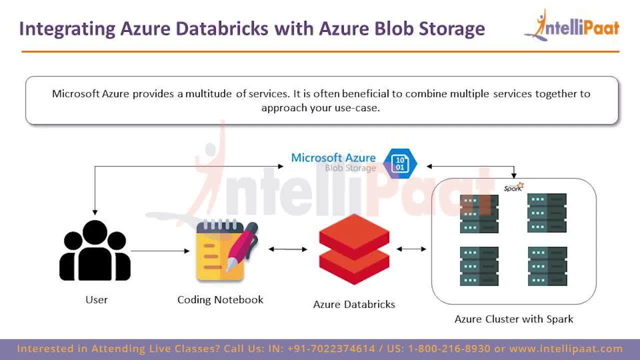 data scientists, data engineers and everybody. So you create your cluster. right. You created the cluster similar to how we created the cluster, And the data scientist could create his own notebook, The data analyst could create his own notebook, But they are using the same cluster. 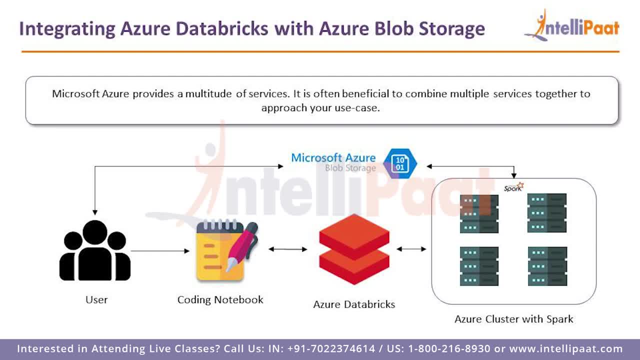 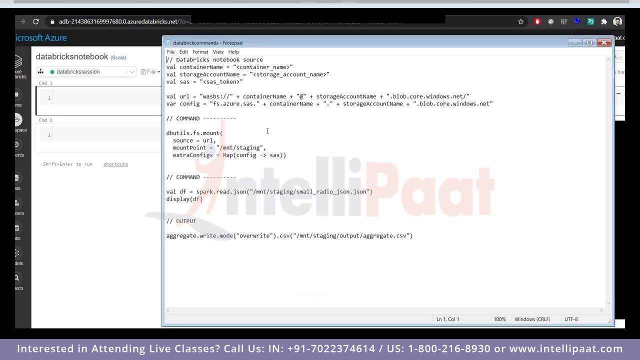 Oh, okay, That is also a way you can implement it, So that is more cost efficient. How to do that? okay, Yeah, So the architecture is clear. Yeah, yeah, So we will now integrate. So this is a little bit tricky. So. 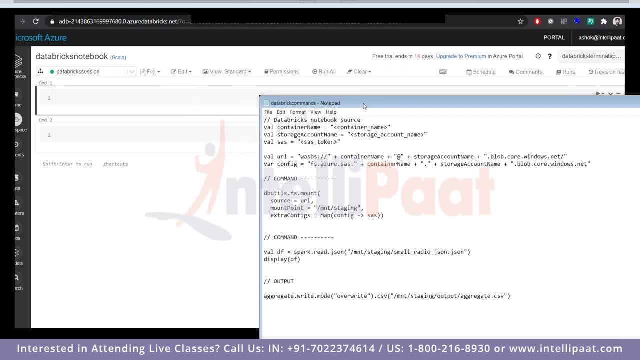 the first thing that we have to do is actually generate a token so that we can actually access this data for a particular amount of time in the same resource group. right The container name and the storage name. we don't have to worry about because we've 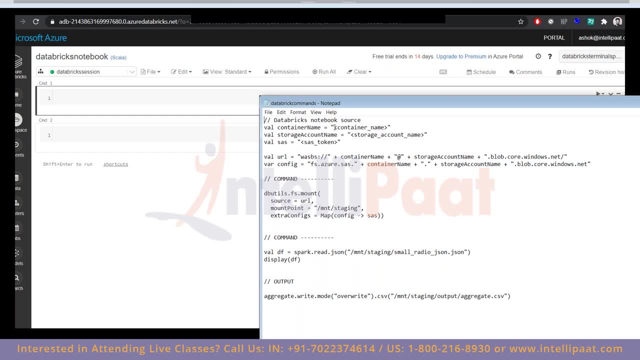 already. There are just string variables that are there in our. I'll just show you in a moment, So I'll just paste this format over here. So this is something that you don't have to memorize, This is something that will be provided to you. 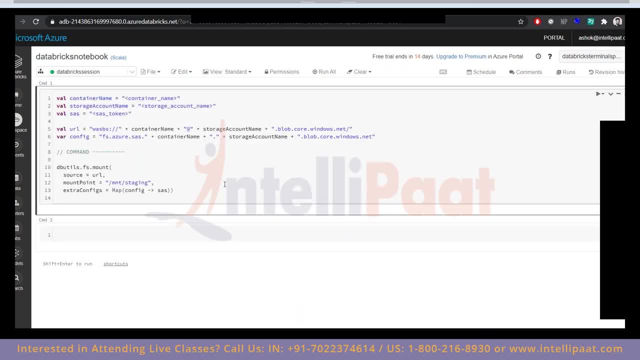 Just copy this and paste it over here. So this is in the format of Scala, So we have to paste all of these things. Firstly, let us look at the container name, right? So now we are going to refer to the storage. 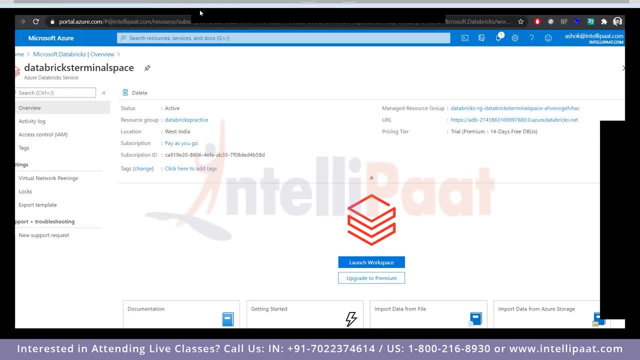 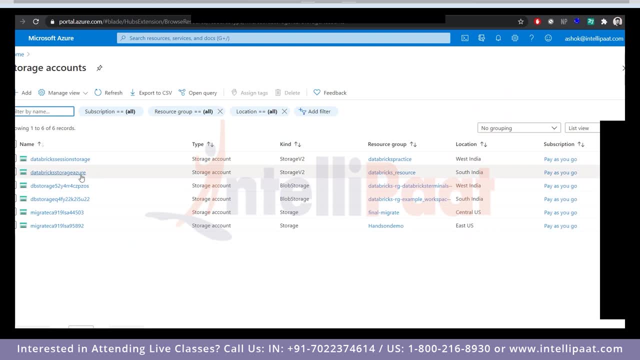 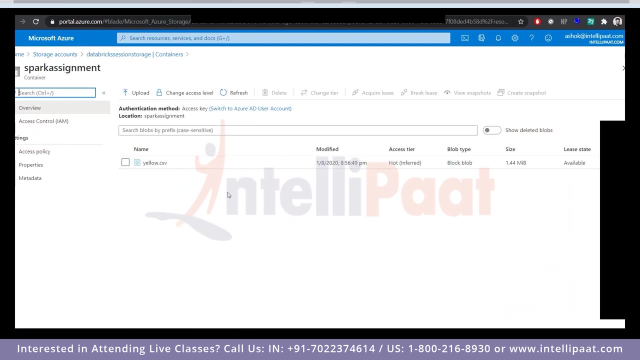 Where's the storage? We did something- data break session, that one right. So open up the portal, Go to the storage accounts, Go to our recently created storage And then we can simply: We go to containers and we have our start assignment. So this: 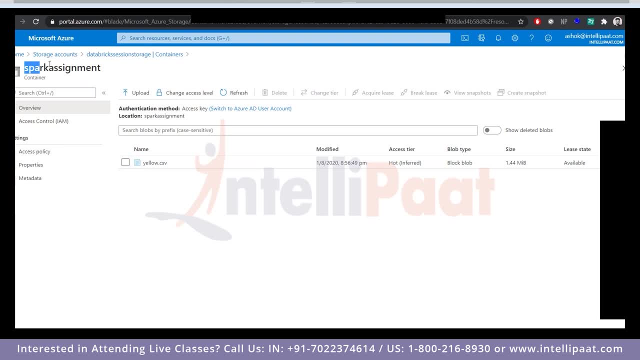 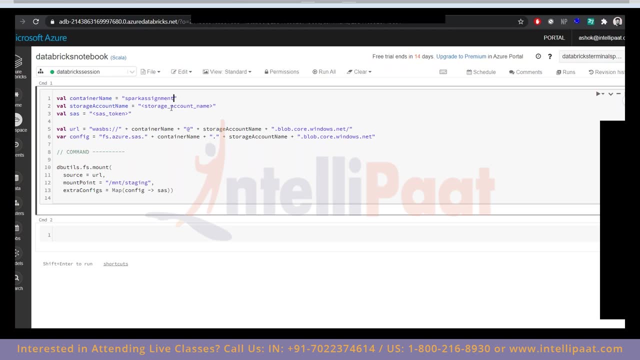 is the container name right. We copy this, Yeah, And we replace it over here. So we created the variable. This is string variable, A normal string variable container name, And it has the name SparkAssignment- Right. The resource group also helps us. 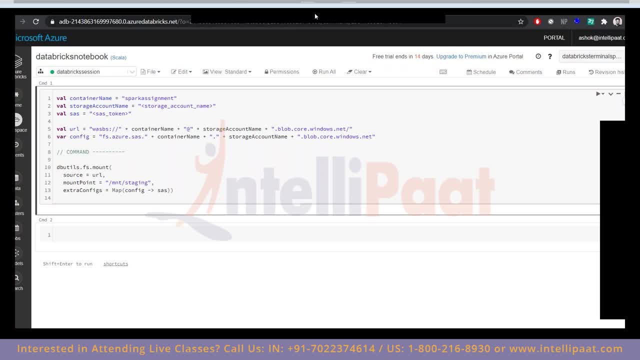 in the way that say, if we are creating two resource groups, there will be no name conflict. Somebody else working with me on the same Azure portal, organizational portal- is using the container name SparkAssignment. We will not have a conflict, Because then we are. 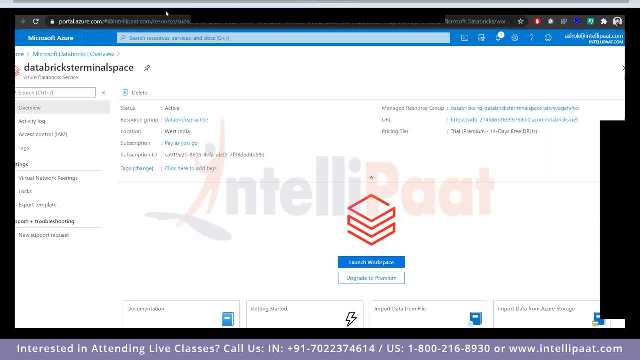 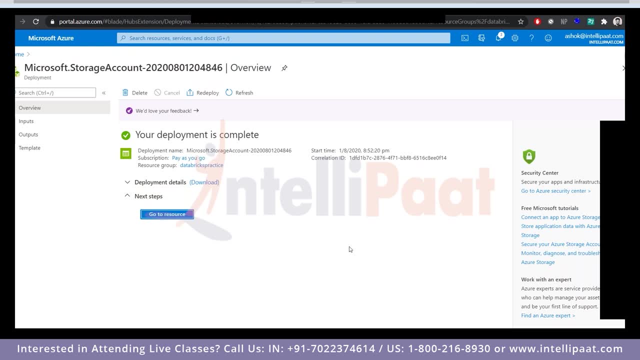 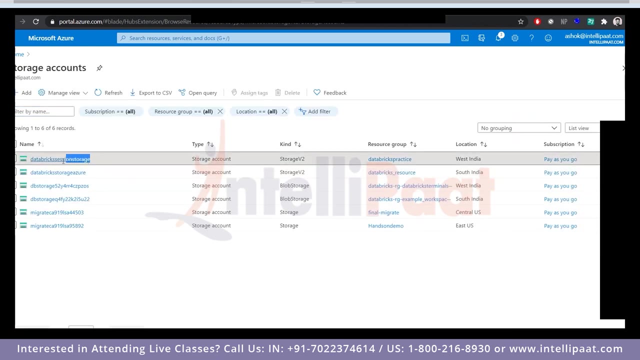 operating within different resource groups. I hope that's clear. Yeah, Okay, Let's go back And look at the storage account name. So storage account name is: Let's go back. So the storage account name is data break session storage. 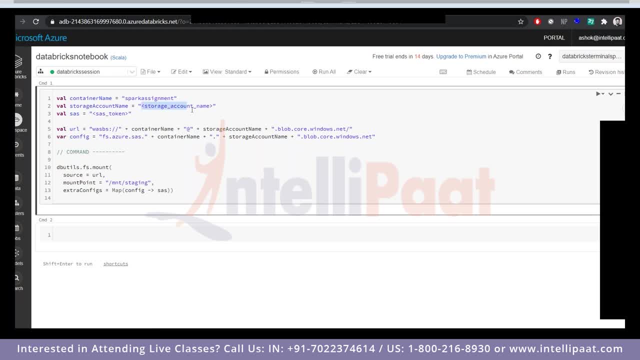 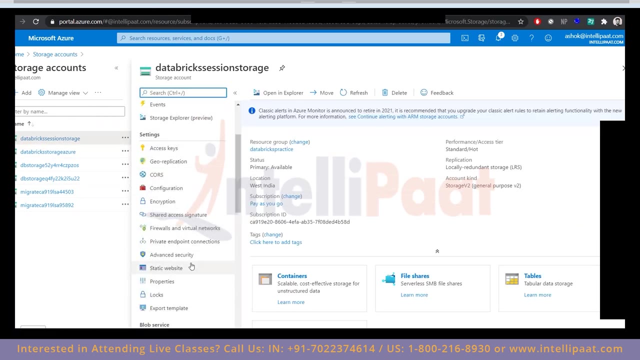 Go back to the Jupyter notebook and replace the storage account name with that Right Now, the SIS token. So this is the part where a little bit of technicality happens. So open it up. This is session storage. Then we have to go to this. 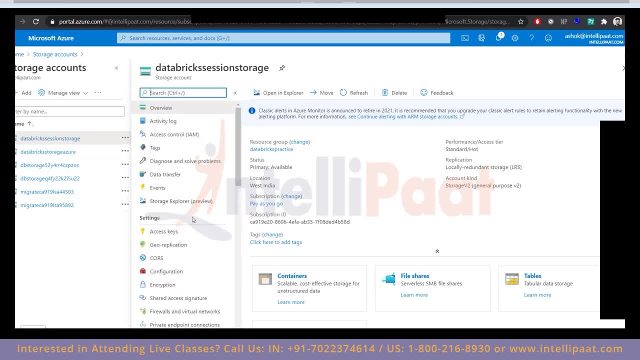 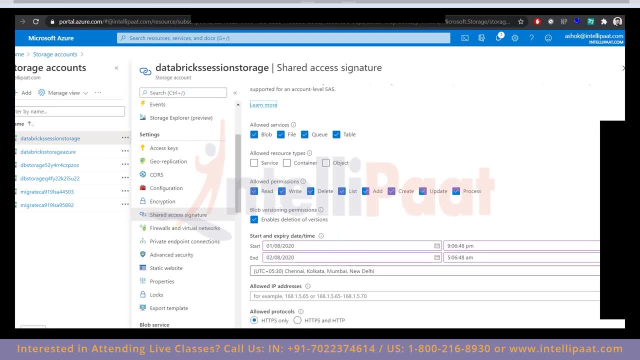 shared access signature. This option that is present in every storage account. So we go to that And now we can generate a token for a limited amount of time, So it will not be valid forever. So say, if I am accessing this data right now, if I am able to do it, 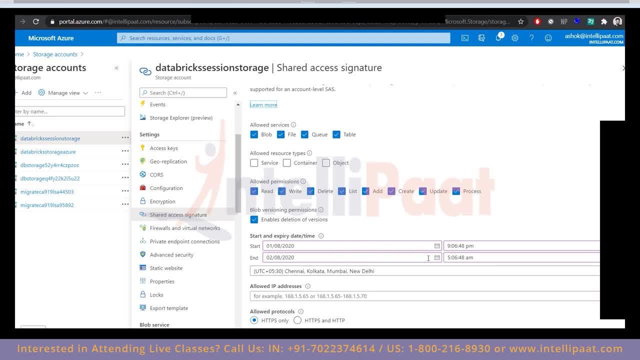 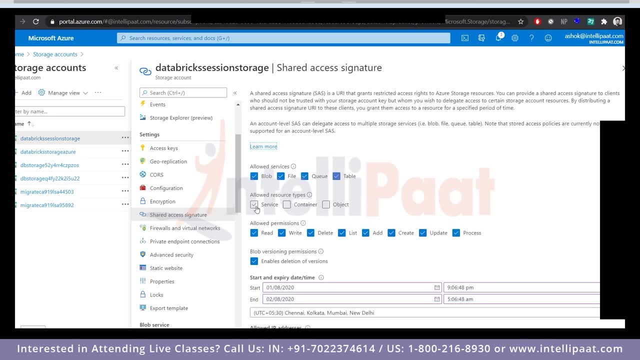 right now I will not be able to access it after the expiry date, So here we can set our expiry date, Obviously for security reasons. Okay, Yeah, That is the time when the token is valid, So we will allow the resource, type, service, container and object. 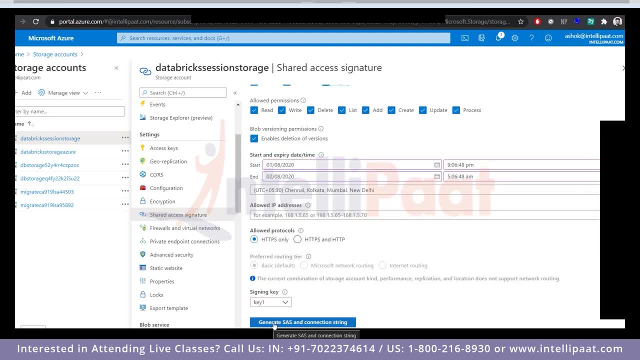 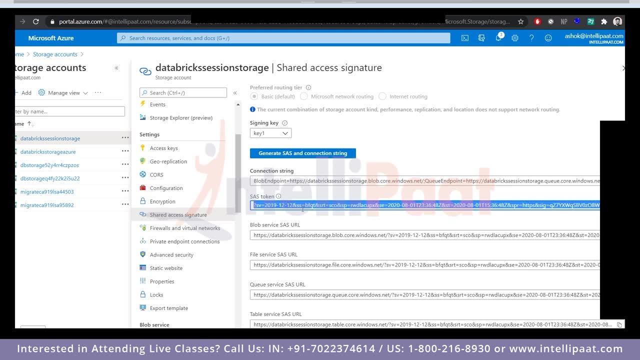 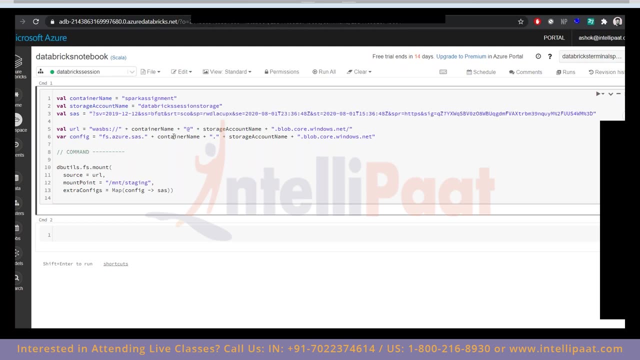 And now we can simply generate our SIS token. So here we have our SIS token. Simply select that, Copy all of it And we can go back to our Jupyter notebook And paste it over here. So we have our SIS token right here. 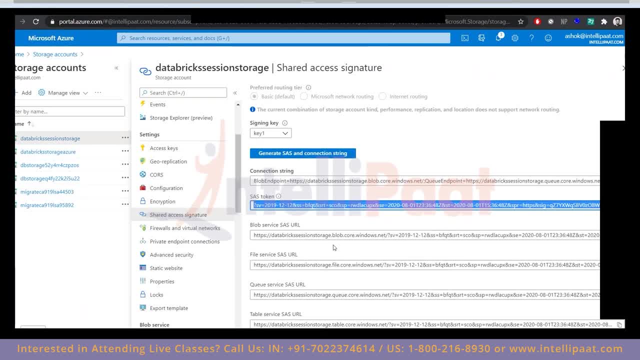 Just a moment. So this is something very it's only for Databricks, right? Not So SIS tokens are. these tokens are also, say, if you are using another service that uses storage accounts and storage within them, So there might be a requirement. 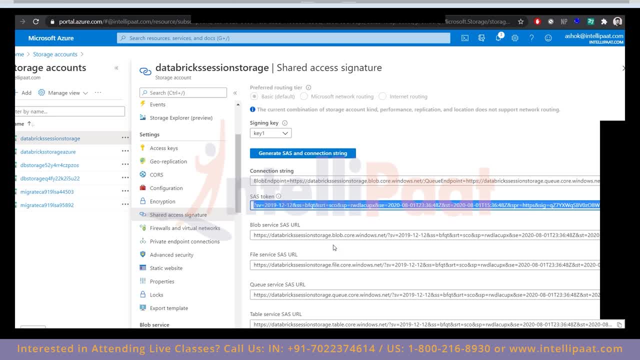 for SIS tokens if you are directly accessing the data without actually So. these are all things. so to avoid any sort of automatic script running Right. If you are doing it manually with the UI, it's all fine, But if you are running in COVID, 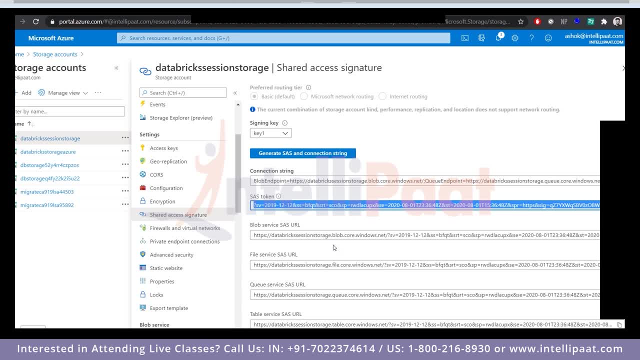 so that is where you need tokens involved. Basically, validity and some validity period involved with those tokens. So I think it should be fine, Although I had a little bit of doubt with, I think, this token itself. So it's valid for one day. 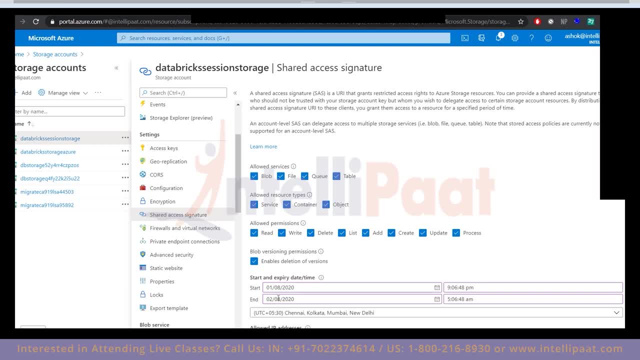 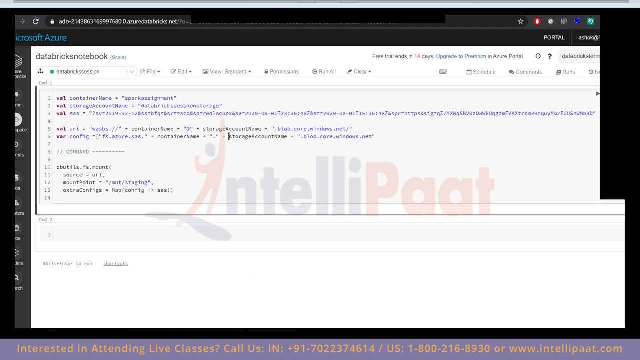 The start period is first and the end period is second August. So, yeah, Alright, So I think it's fine. Alright, So the rest of it remains the same, Right? So it basically creates new variables, new string variables, where it's creating 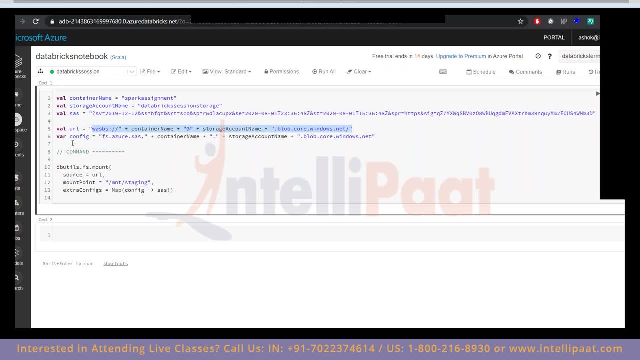 these links Right By appending all of these strings together. So we have our URL, we have our configuration Right And once we run this, dbutils. Now here is the dbutils concept, Because this is not something you would do in. 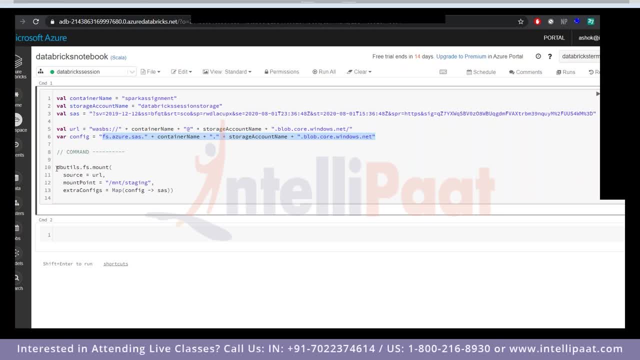 Spark or any other way, Right? So this is where Databricks comes in and tells you that: okay, if you are using cloud services now, we will help you get your data from some other service or some other storage place. Right, So we provide the source as URL. 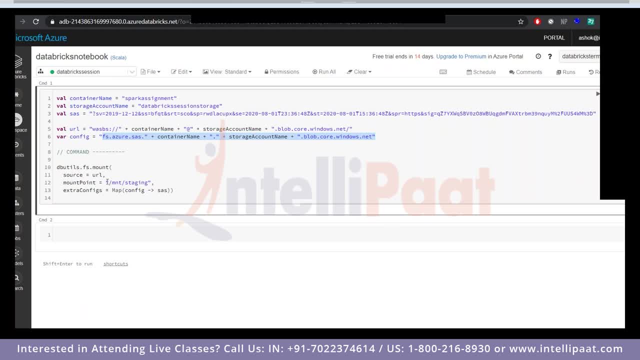 the mount point as slash mnt. This is something you are creating Right, So you can use this address to basically assign to this particular storage container that we are. We are assigning this string to that. We are assigning this string to that storage container So that whenever we use- 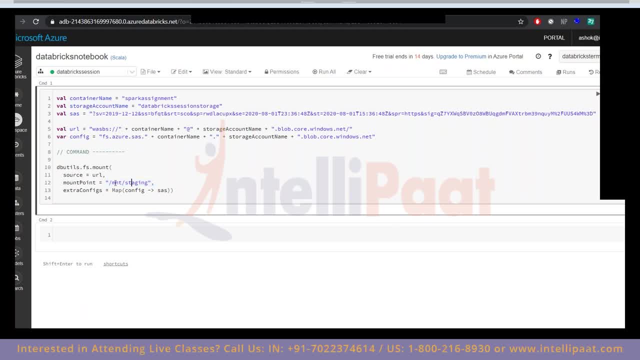 this string, we are actually referring to the storage container, Right? We can put in anything over here, Any string value that we want, And then we specify the configurations, We map the config with the SAS token that we have just created, Right? So all of this is just to memorize. 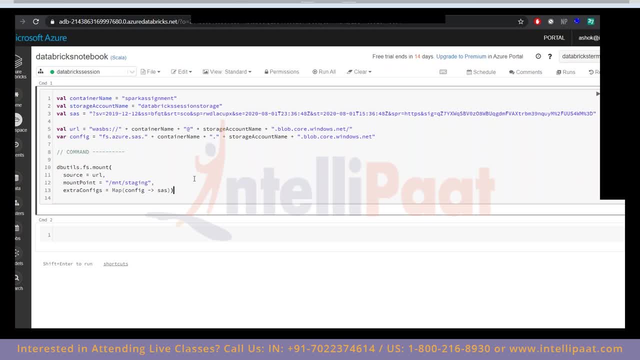 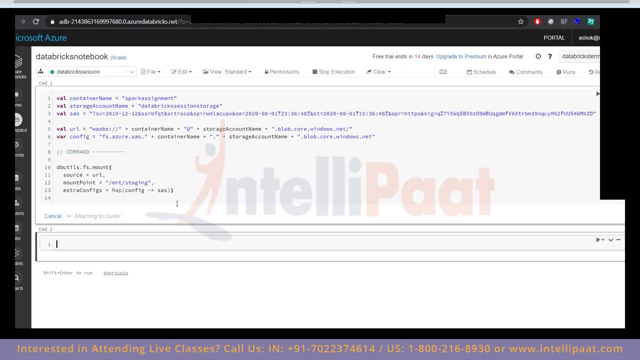 Basically And then not memorize to basically copy and paste. It's like template code, Yeah, And then you press should plus enter And it will first. the code will first refer to the first communicate with the cluster, as we have shown in the diagram. 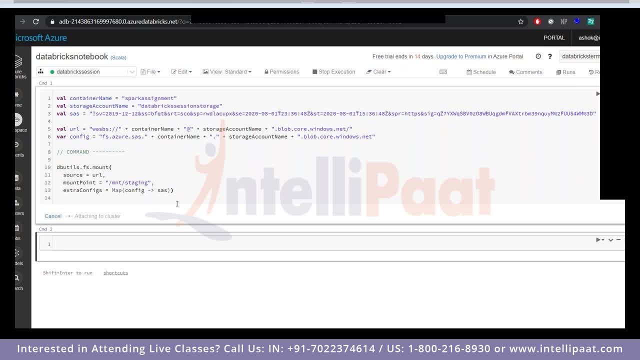 It first communicates with Azure Databricks and then it communicates with the cluster. The code executes on the cluster And then, once all of this is set up, we will get our similar to how Jupyter Notebook works. We will get our output message over here. So let us. 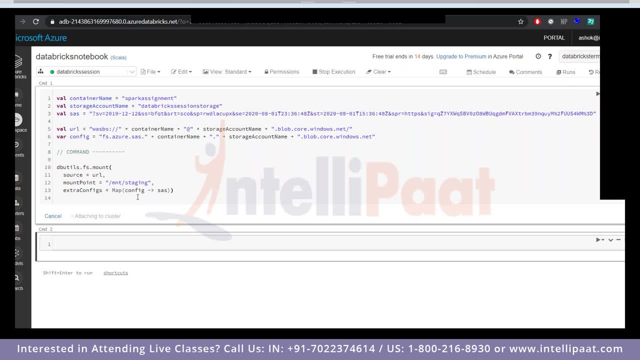 wait for that. So you just executed only those 13 lines, is it? Yes, Okay, So we are just attaching with the storage account. Yeah, And we are attaching to the container, Not the storage account, To the container Where we are having our file. 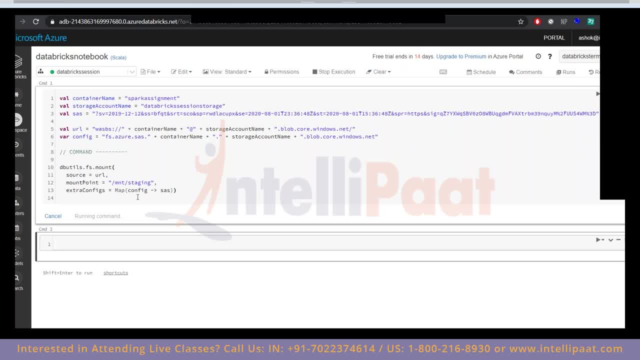 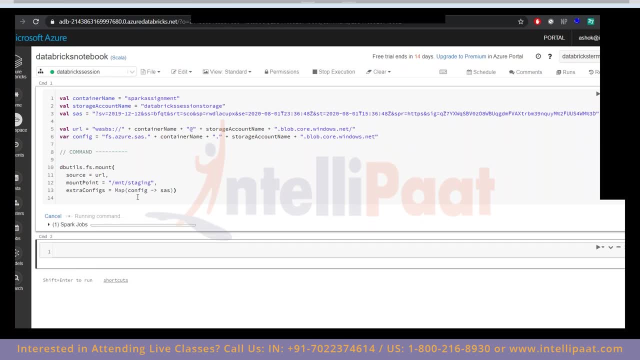 So once we have done with that, then it becomes pretty simple. Then I think we will get into the territory where you remember what we are doing, Where you are familiar with what we are doing. So now it is running the command. There is one Spark job. 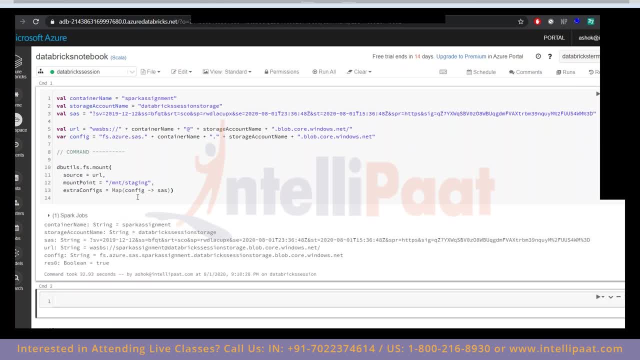 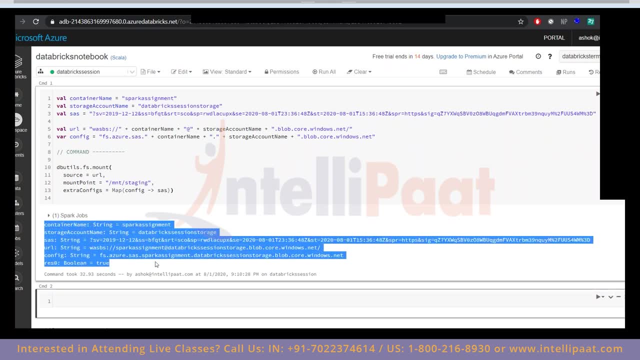 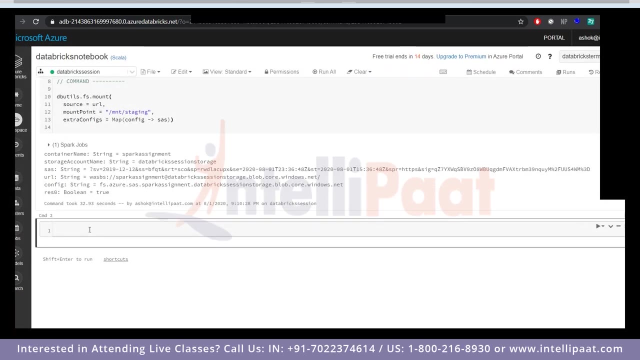 So, once that is finished executing, we have successfully assigned a particular address to our data container location. So we can see all of the details are there, Right, And now we can start, Right? So let me just look at the file name, Alright, So 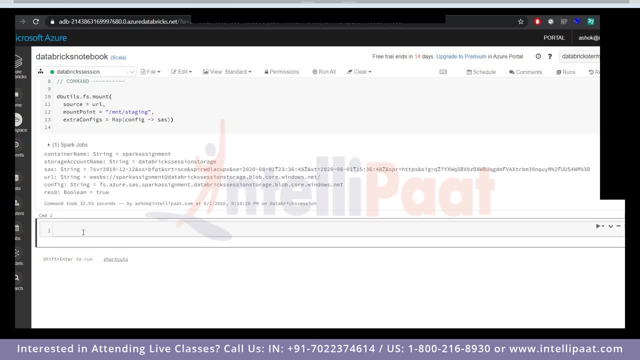 it is yellow dot chp. Yeah, That I remember. So create a val. So val is basically how it works in Python, Except in Python you don't have to write anything before your variables. So you write val and depending on the value that is assigned, 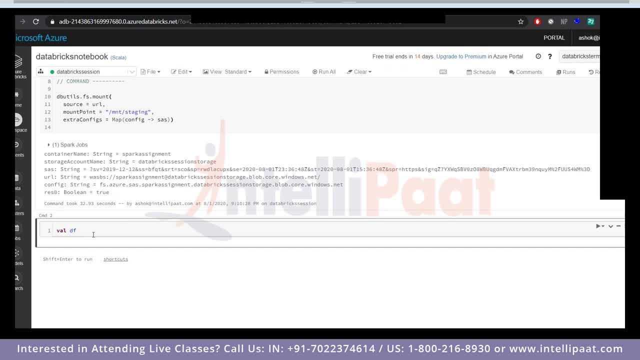 to a particular variable, it will change the data type as well. So exactly how it works in Python. And then you equate it. Now you will remember how. this is something you might remember. Spark dot read And then you give in the format. So the format right. 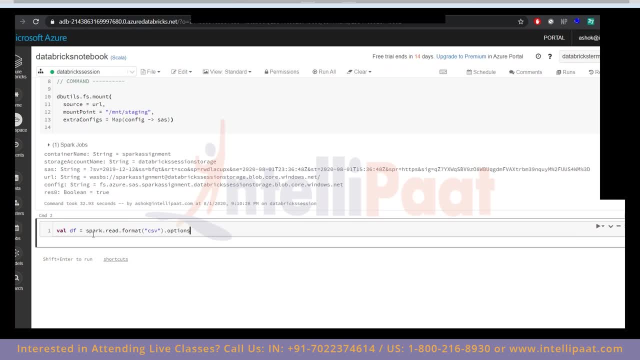 now is a csv. Then you give in other options as well. Like you want the headers to be there, Then you give in the option Because we are going to be implementing Spark SQL on it. We can essentially write this as well: The. 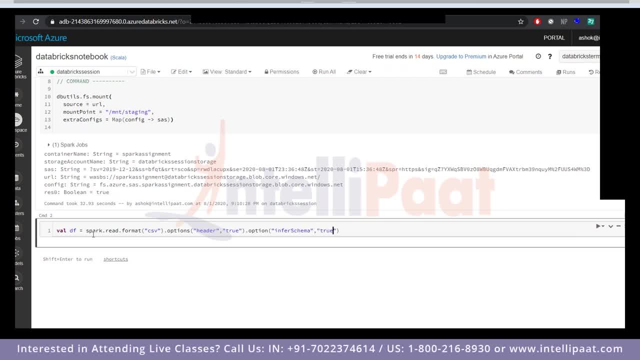 inverse schema And we assign that as true as well, And for efficient data replication requirements, we will add the fail fast mode: Yeah, And then we give in the location. Now, here is the part where the only thing you need to notice is this particular 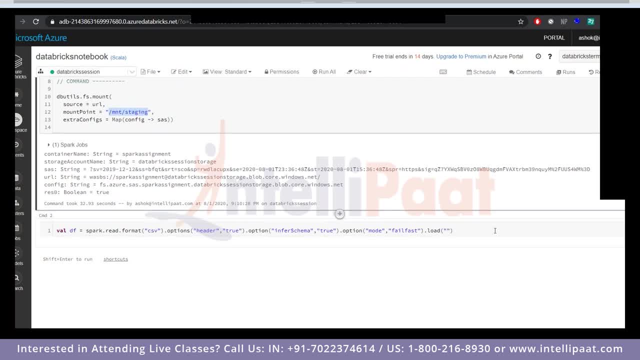 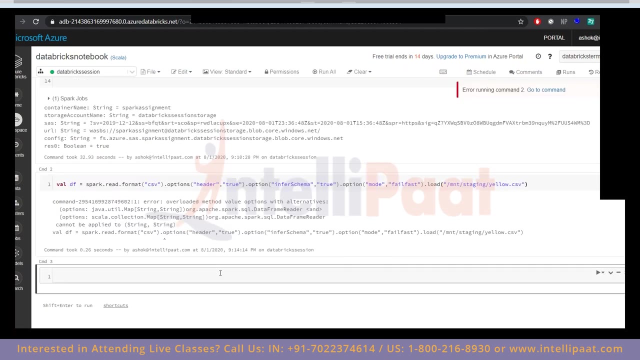 address: Write the mount point. We can use that. Copy this, Paste it over here: Yellow dot csv. So it should work. now Let's see. And then we press shift plus enter. There is an issue that we faced Just a moment. 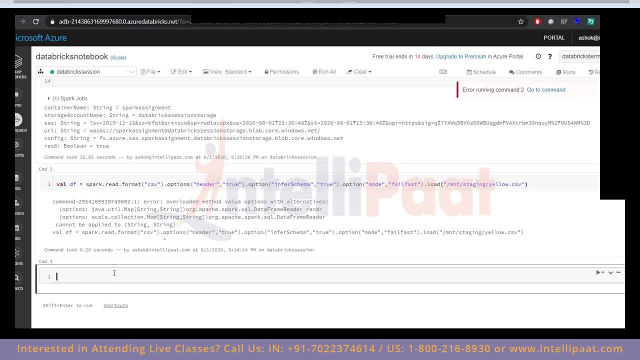 Options. No, There is option or options. You have written options. Yeah, It's options. One place I have written options, So let's just change that. So one of the other advantages of using a notebook is that you can simply go over here and just remove this. 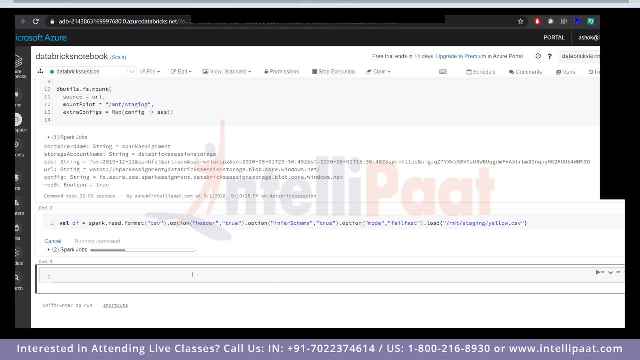 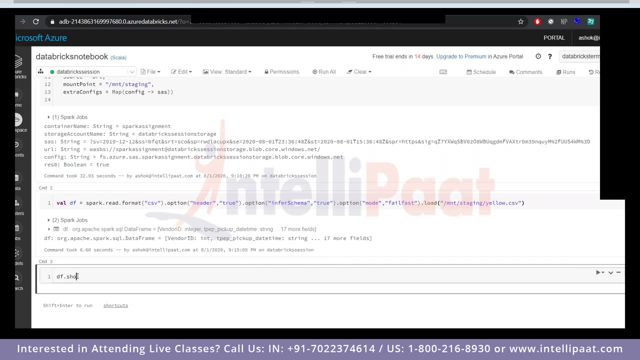 And you don't have to write it again. Appreciate the assist. Did not spot the s over there. So now we have created our data frame, Let us see that dfshow and just limit that to 4.. So let us just press enter. 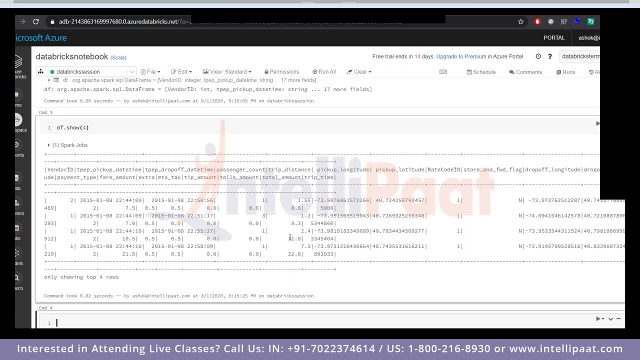 So we have our data available to us. It's quite big for the screen so that is why it has shifted in that, But it is there. So it is essentially some taxi job data, Some taxi online taxi service data Where we have the pick up time. 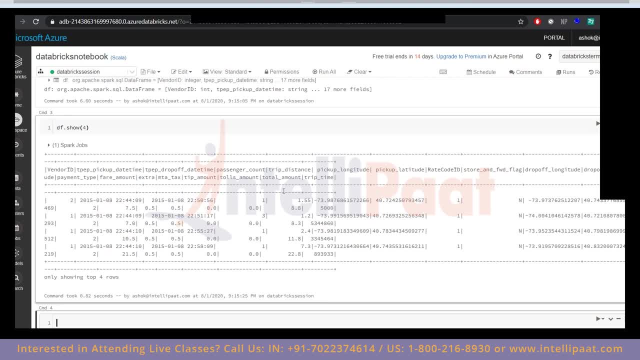 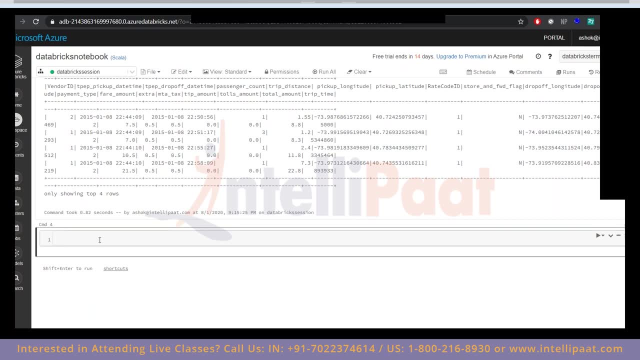 and the drop off time, The passenger count, Trip distance and everything. So it's there. Using this data frame, Yeah, So we can simply write something like: everything is something like this A df. We can create a temporary view out of it. 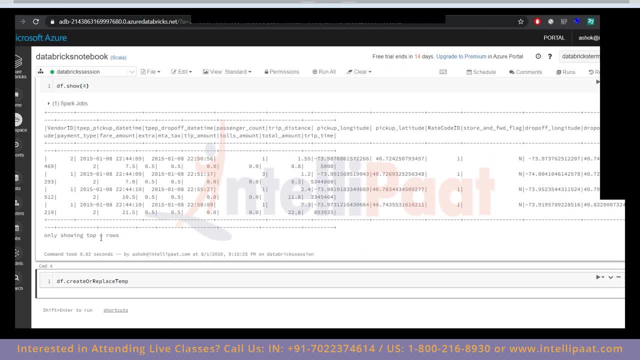 This is something you might be familiar with. This is exclusively. This is now we are in. We are done with everything that is supposed to be about data bricks. Now it is simple coding In Scala or in Python And wherever you want to use. 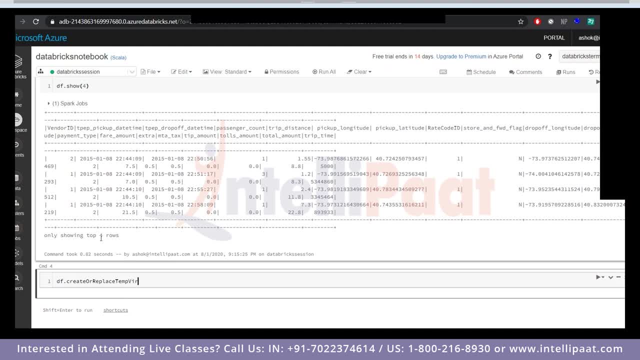 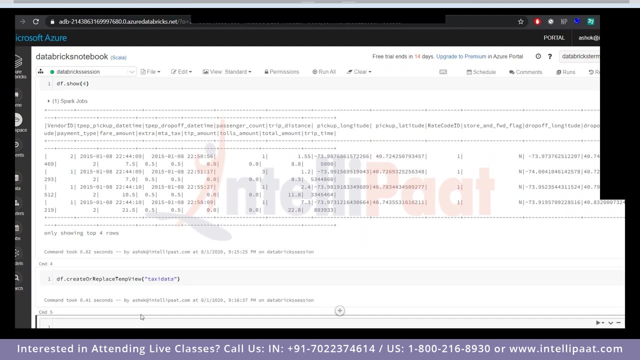 So let us just name this temp view, Let us name this taxi job taxi data, So we can refer to it by spark sql And just press enter, Shift plus enter. So we have done that. You can also click on the play button instead of doing that. 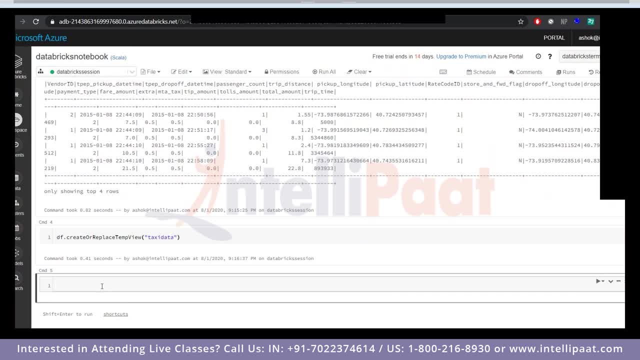 But that obviously takes a lot of time. So say, if we want to select, find out the number of rows, Number of trips, total, Right, So we can just count the number of rows. So spark dot sql, select, And then we are given the count. 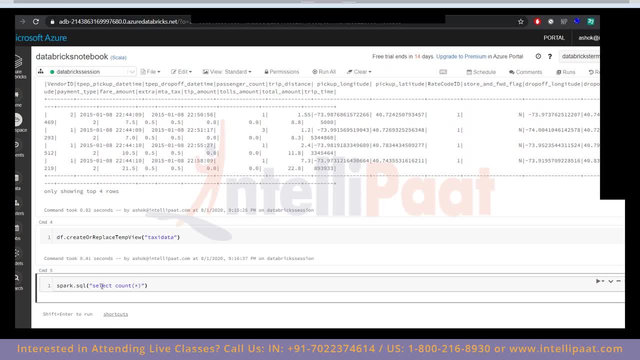 We are counting all. So we will just give that From, And since we have named the temporary view as taxi data, We will refer to that, And then we give in the dot show Shift plus enter, And it will give us the. 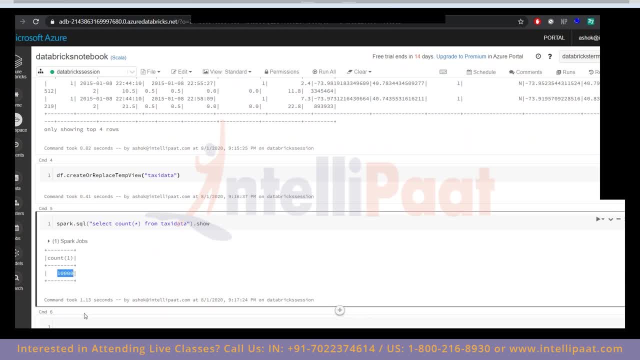 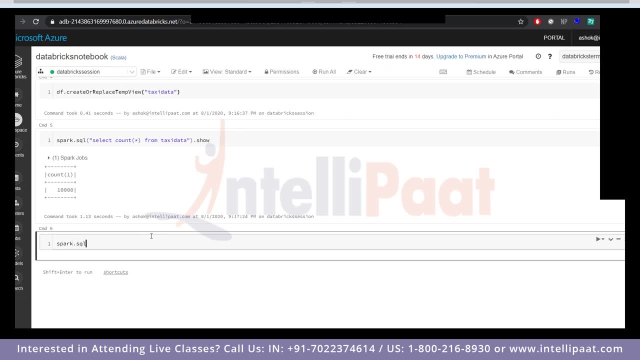 information that we need. So it is about 10,000 records. So, similar to that, You can spark sql and write anything. The reason I am using spark sql is because you might not be familiar with the inbuilt Scala functions that are there. 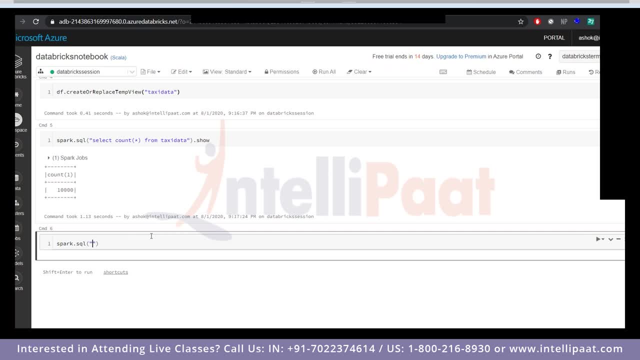 So spark sql gives us a common platform to communicate. Yeah, So now we can do something like: if you want to find out the total revenue that is generated by all of the trips, So we can do something like select sum And then, given the 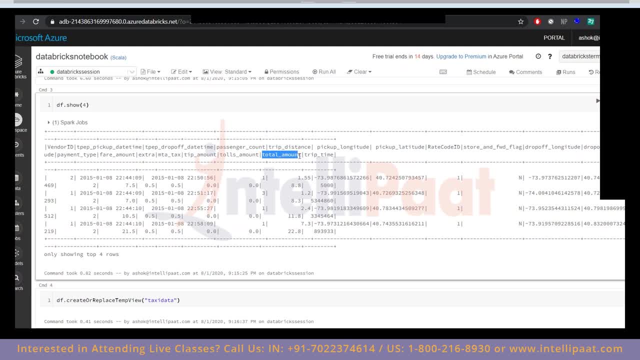 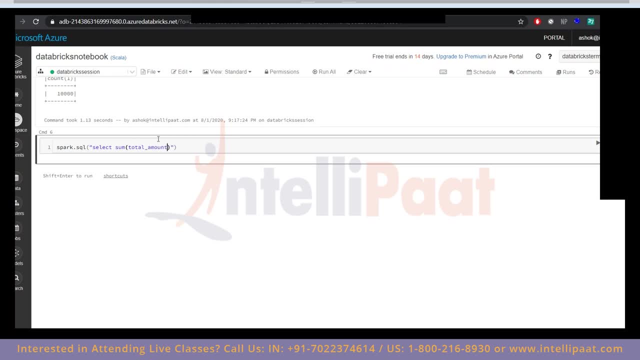 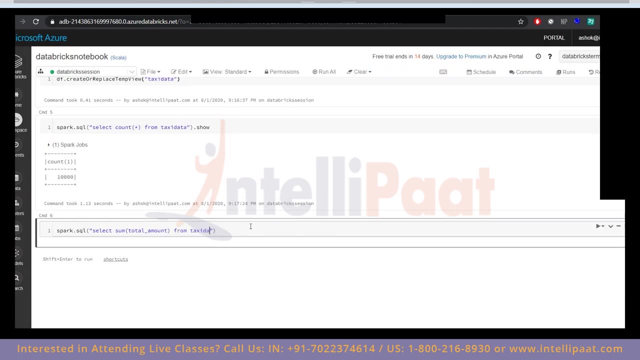 column name. Let us look at the column name: Total amount. Let us take that And put it over here: Total. I think it was underscore amount, Is it underscore? Yeah, yeah, Total underscore. So, and from taxi data dot show. 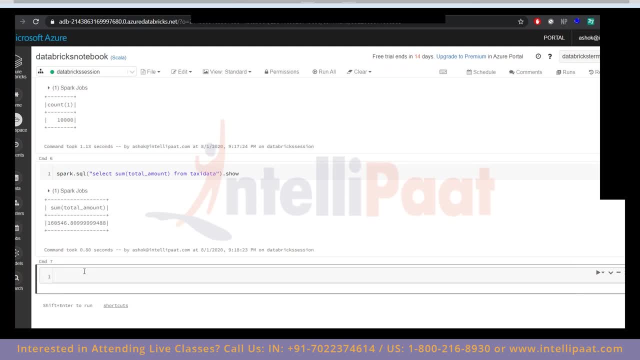 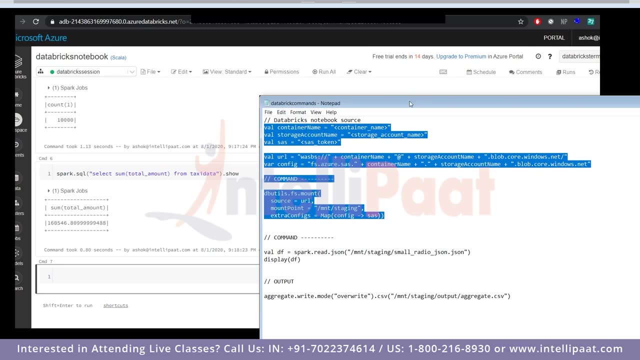 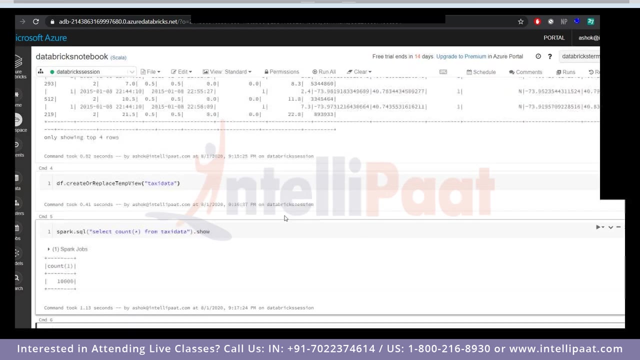 So this is the total amount. Yeah, Just a moment. And all of this if you want to simply say: Now you want to write some data back into the service, So there is also another method for that, Since we have already created our mounting location. 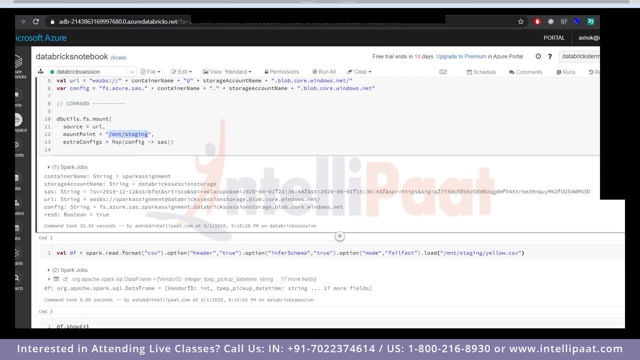 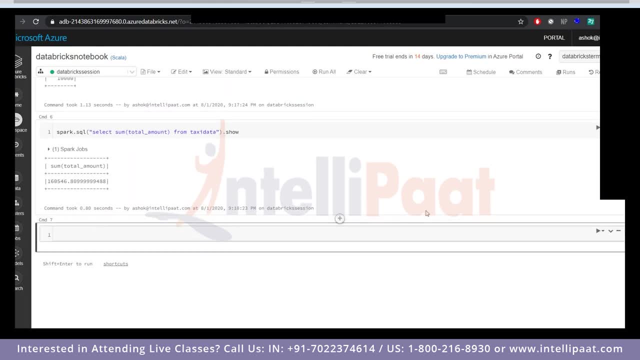 Right, this. We can use this to also write back the data. Okay, okay, Right. so So to create a new file there? Yeah, So the way we do that is use this function, Use this aggregate write mode: Right, Simply copy this and: 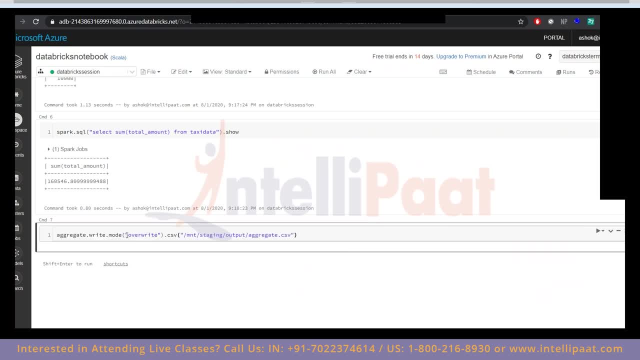 paste it over here Right, So overwrite. if you initialize the overwrite mode, So if it has something with the same file name, It will overwrite that. So this is usually done. Say, What will you do when you have a routine procedure to follow? 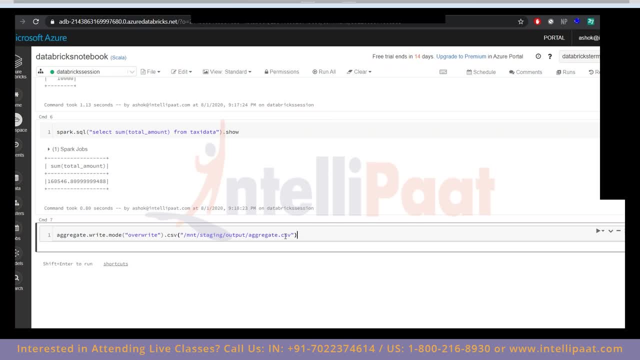 Right, say You want to constantly keep replacing the data that you have With new results, Like on a daily basis, say, Because the statistics change everyday for your usage. Yeah, So it will. If you don't write the overwrite over there, It will basically. 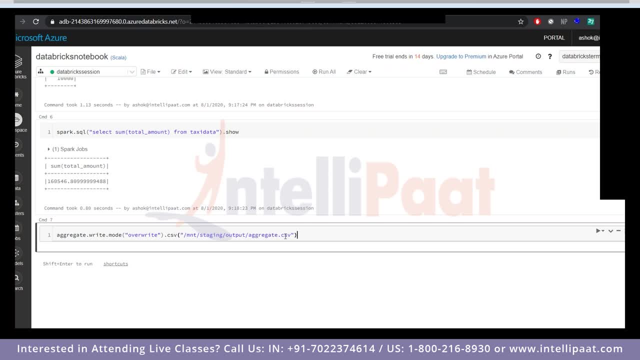 throw an error right Because the file name already exists, So you have to put in the overwrite method. It depends on the use case entirely Essentially. Or you could simply specify some counter or, and you can implement that in the string, Concatenate it over here. The counter will increase. 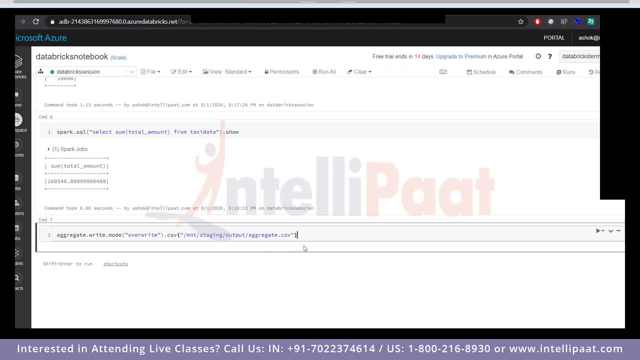 So file name should be different. You don't need to write overwrite, Right. So if I simply do that, and just a moment, The aggregate is not an actual. I think it's not the actual function. It's something for a default We have to use over here. 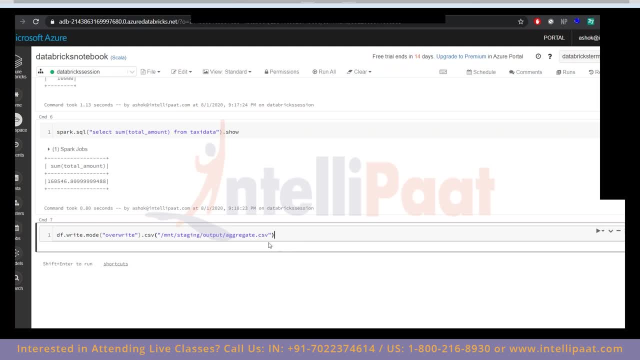 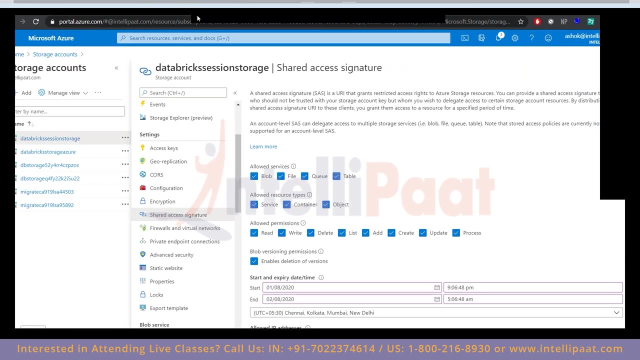 We have to use df Right. So once we've done that and put in something like dfo, That is not essential, by the way, But we're understanding it over there. So if we just simply go back And check our storage, 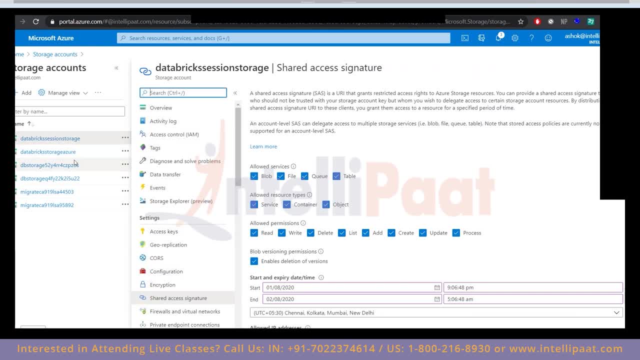 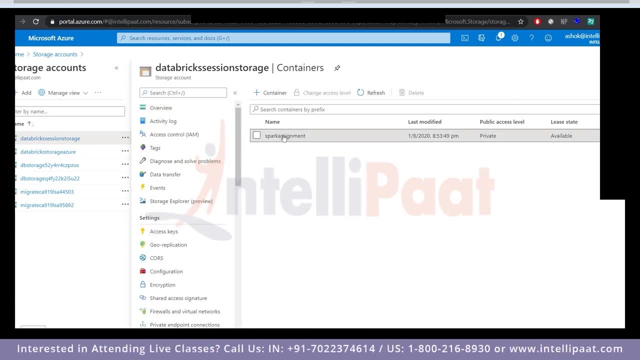 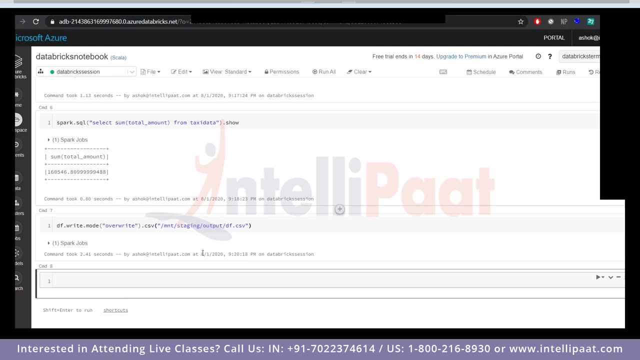 Yes, exactly So this one Overview. We go to containers, We go to spark assignment, So we have our output Right here, Right? So if we simply look at the folder structure, So it was up until mnt staging, Right, This is what we moved.